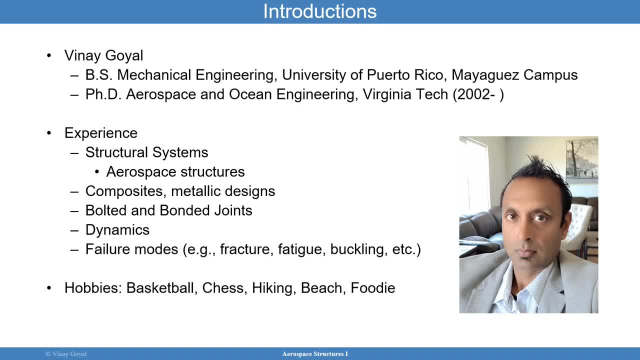 if the test is going to pass or not, And so that really increases the excitement that I have for this field. And then the second thing I really enjoy- and it sounds very strange, but I do enjoy- anomalies that occur, Because when they occur in flight it's an opportunity for me to learn. 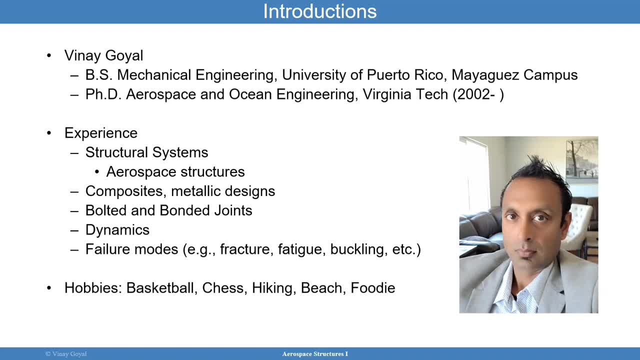 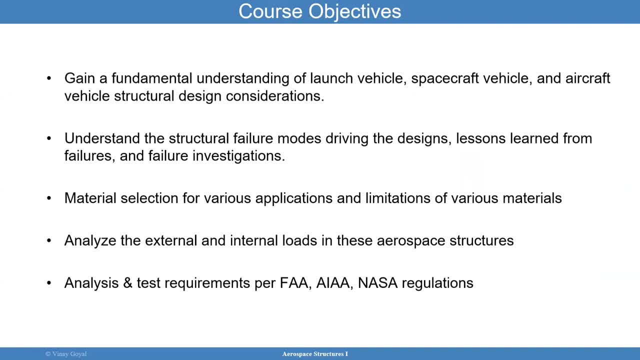 and it's an opportunity to learn from the failures that we have seen. What are the course objectives? What do we have in mind? What we want to do is gain a fundamental understanding of launch vehicle, spacecraft vehicle and aircraft vehicle structural design considerations. We also want to understand 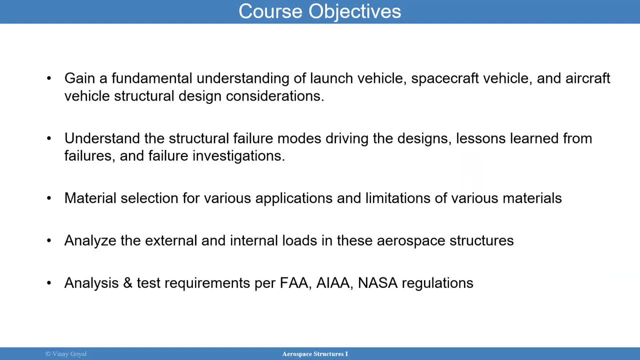 the types of failure modes that could drive the designs. We also want to cover lessons learned from these failures and how to conduct a failure investigation, which I think is very important for us to be able to understand the types of failure modes that could drive the designs. 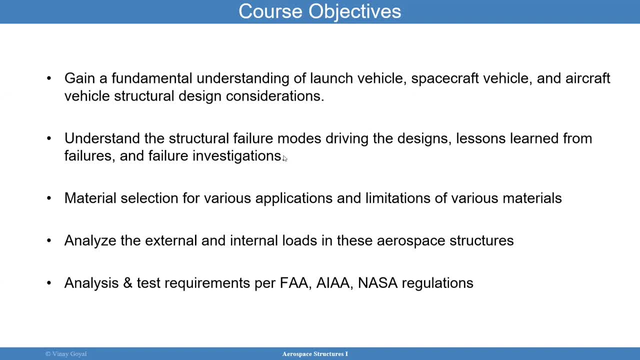 When you're dealing with anomalies. We're also going to cover material selection for various applications and the limitations of those materials to these three applications: launch vehicles, spacecraft and aircraft vehicles. We're also going to analyze the external and internal loads in these aerospace structures And then we're going to look at the 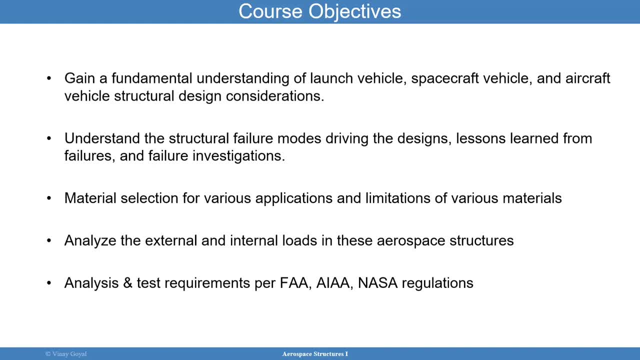 requirements that exist from the FAA, AIAA, NASA and other organizations, So you can understand what are those requirements that drive the designs in general. And as we do so, I think it's important that you start reviewing statics of materials, which can be an important subject, and also 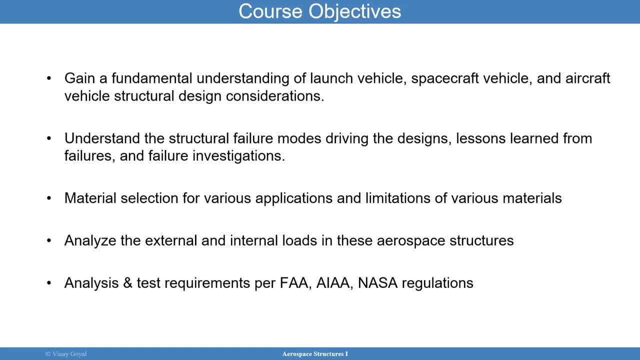 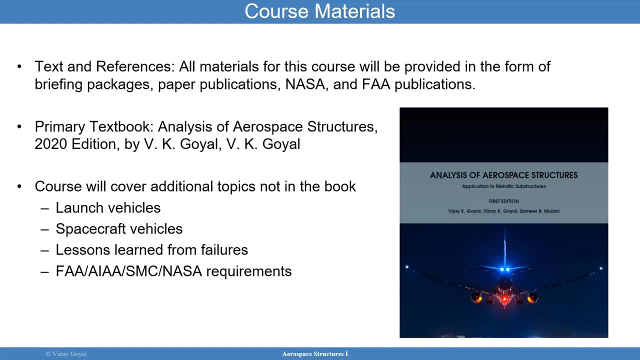 mechanics of materials. Those two courses can be quite valuable in this course as well. The next thing that we're going to talk about is the course materials. The text and references for this course will all be provided to you. I'll provide you all the course materials in the PowerPoint, in the form of briefing packages, paper publication and printouts. 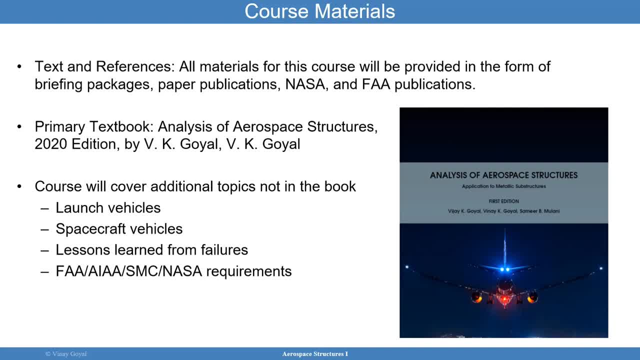 publications: NASA and FAA publications. The primary textbook of this course is the one I wrote with my brother. It's called Analysis of Aerospace Structures and it's the first edition. This edition here will cover primarily aircraft design, but it can also cover can. 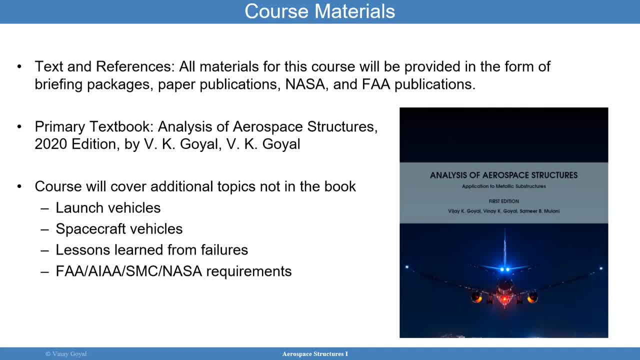 be extended to other applications. The course will cover topics that are not included in this book, such as launch vehicles, spacecraft vehicles and potential lessons learned from failure. We will cover some FAA requirements in this book, but not all of them. For example, 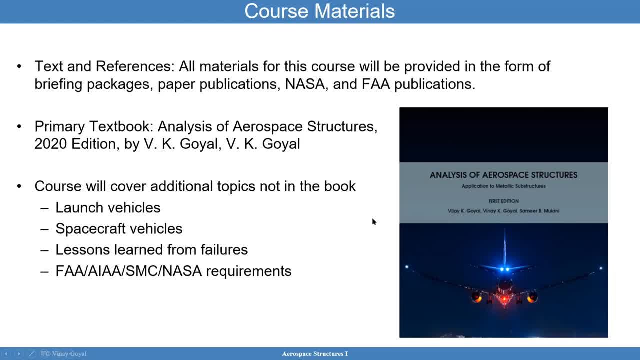 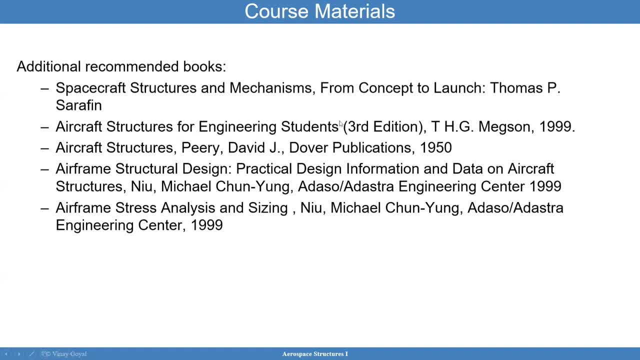 AIAA and NASA requirements may not be covered in this book. What we're going to be discussing now is the additional recommended books. Spacecraft and Structures and Mechanisms is a book I recommend if you're going to work in the spacecraft world. I'll be covering topics from that book. 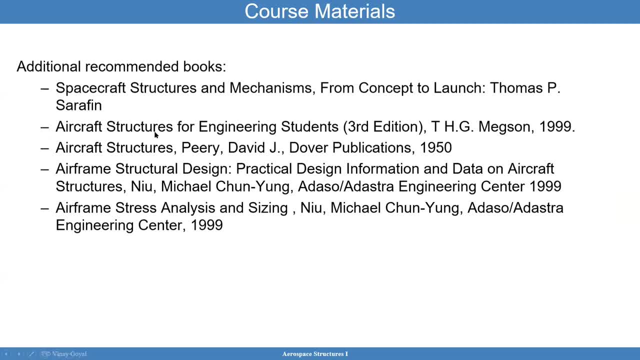 as well, And I also recommend getting hold of other books if you're going to work on aircraft designs. It's called the Aircraft Structures for Engineering Students. That's another book I recommend, if you can get it from the library or get a used copy of it. 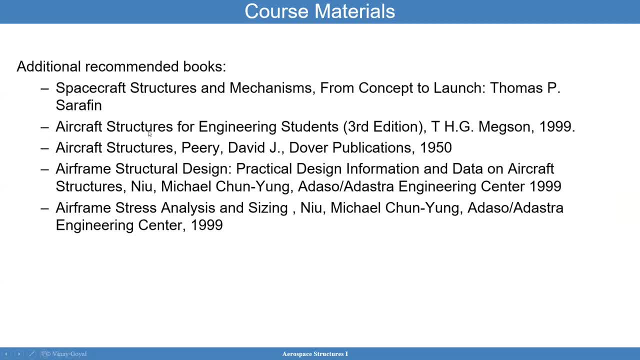 But I will primarily be using my book, so this is not a requirement. If you want to see how others will approach a subject, then it's worth it. Aircraft Structures by Peary. We also have Airframe Structural Design, Practical Design, Information and Data on Aircraft Structures. This book is also recommended for you to purchase. 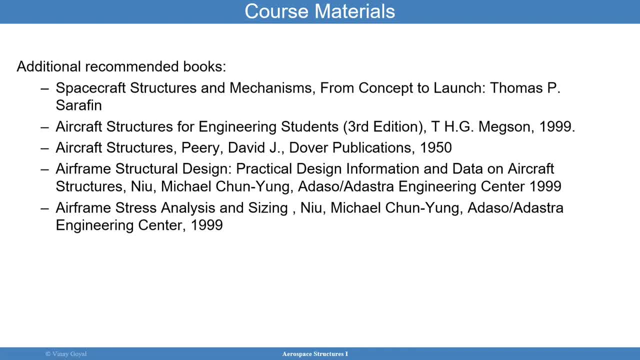 or to borrow: Okay, so, So it could be helpful in your career if this is what you happen to pursue. you also have the book airframe stress analysis and sizing- again another great book. so all these books are recommended, not required. i'll be covering a lot of these topics, uh, through, uh, these. 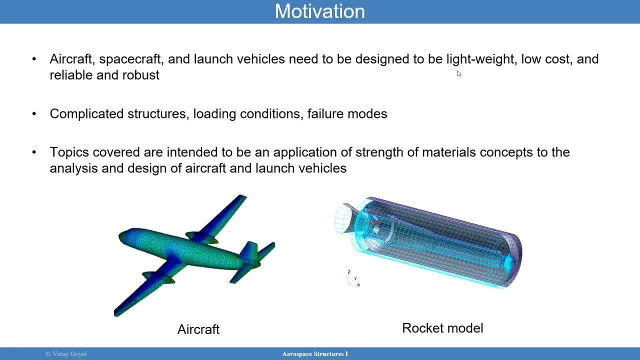 discourse materials. um, so what is the motivation for for this course? the motivation is that aircraft, spacecraft and launch vehicles need to be designed to be lightweight, low cost, reliable and robust to be able to meet some mission requirements, and so it's important to understand that. what this course is doing is giving you that background. um, and what makes aerospace? 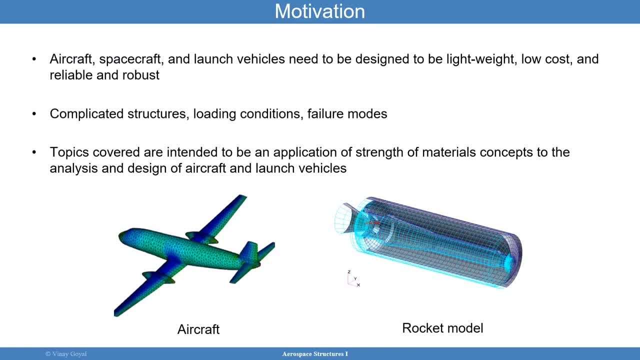 structure so complicated compared to, say, a ground system like a building, is that an aircraft, spacecraft and launch vehicles contain a lot of pieces coming together to perform a function that's not very simple. secondly, the the primary difficulty with these designs that they need to be low weight. they have to be lightweight because we're flying them and not that not. 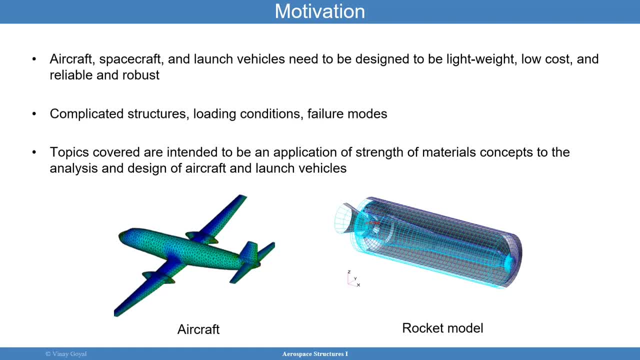 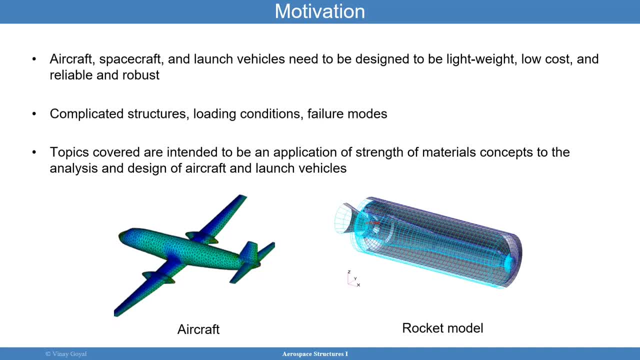 dollars as an example. So the topics covered in this course are intended to be an application of the strength of materials courses you may have taken and then applying those concepts to the analysis and design of an aircraft and launch vehicles. Here's an example of an aircraft. 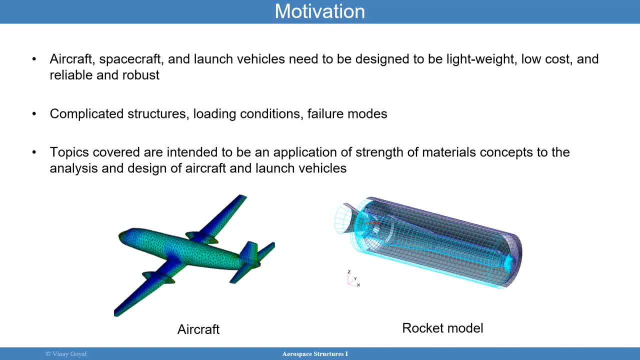 finite element model. A finite element model is a mathematical representation of the structure and it allows you to solve for specific variables of interest. That allows you to then evaluate the design to ensure that it's robust enough to be able to perform a specific task. So this is an example of an aircraft and launch vehicles. 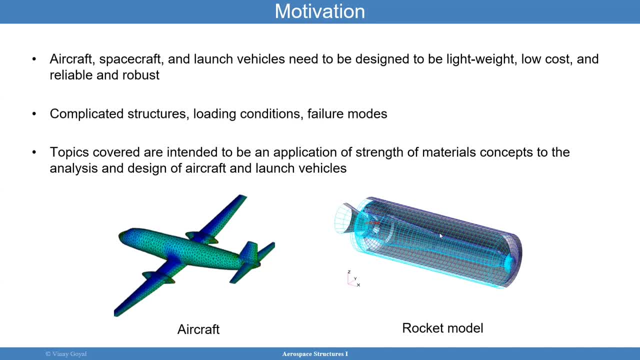 So this is an example of an aircraft and launch vehicles. So this is an example of an aircraft and launch vehicles. boeing 787 Is a finite element model as well. On the right hand side of a rocket model, It's a finite item and model as well In this case. 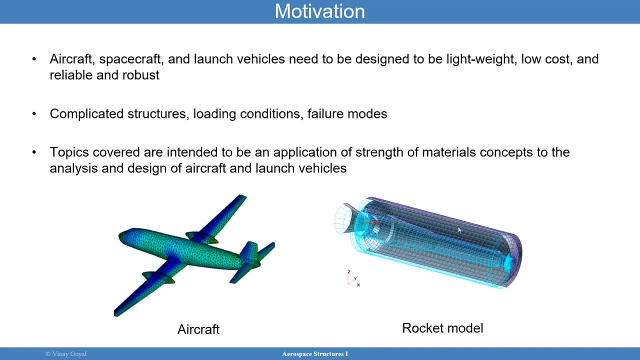 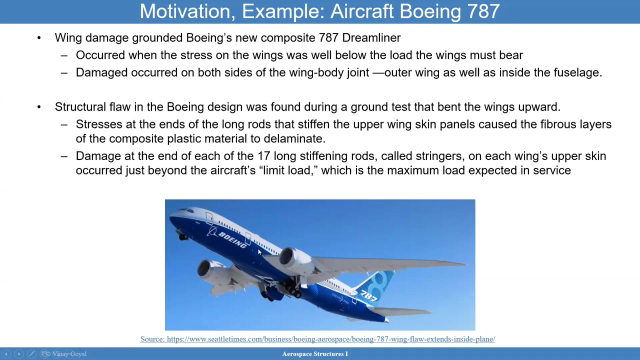 you have a solid rocket motor where the gray region corresponds to the solid rocket propellant. In these two scenarios, this finite element models were developed to try to fundamentally understand the designs during operation boeing 787. In this example, there was wing damage that grounded the Boeing New Composite 787 Dreamliner. 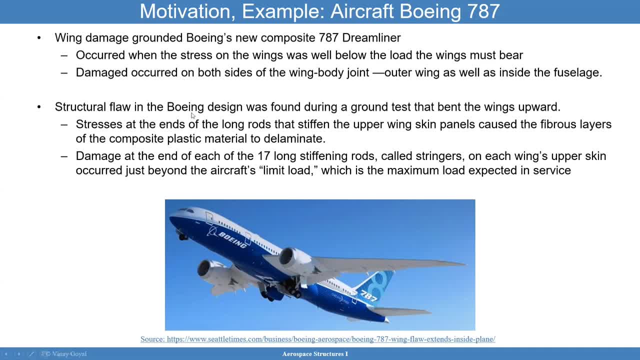 It occurred when the stresses on the wings was well below the loads the wings could take. Damage occurred on either side of the wing body joint. So here in this region and you know, in this area, the structural flaw in the Boeing design was found during the ground test that bent the wing upwards. 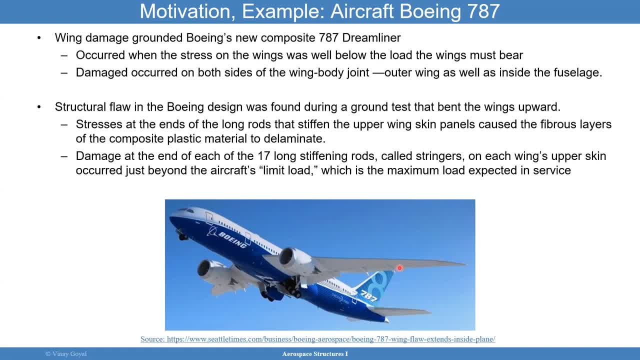 So one of the testing that's done is to apply loading to these wings, And what we do is we apply loading to the wing and we bend it upwards, and we can bend it several feet up, And the purpose of that test is to verify the integrity, the design integrity of that wing. 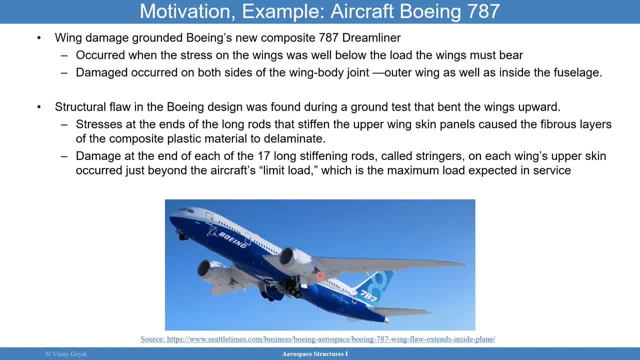 And the stresses at the end of the long rods that stiffen the upper wing skin panels cause the composites to delaminate, And damage did occur at the end of each of the 17 long stiffening rods, which we typically call stringers. 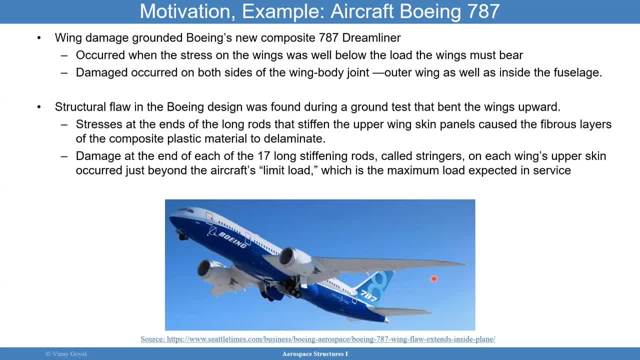 And on Each wing's upper skin there was some amount of damage and then testing. The testing was was supposed to go to ultimate load levels. I'll discuss ultimate load levels later- But the bottom line is that it occurred very close to the loads they will have seen in flight. 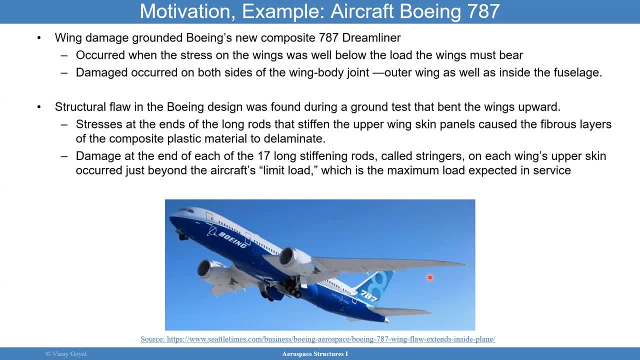 The maximum loads expected in service, And so for that reason, these, these design had to be revisited. the sources given here at the bottom. But the question then becomes: what failed here, Why? Why was there an issue with the testing? 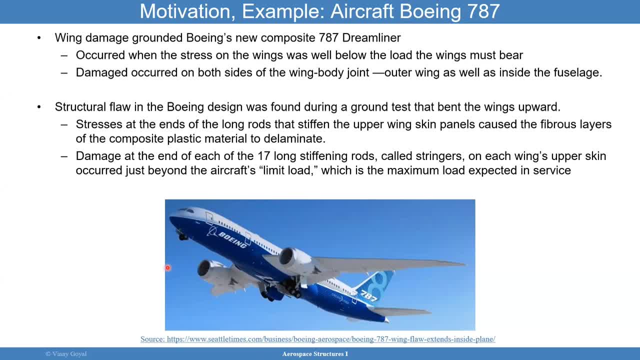 Well, the bottom line is that testing is important for a reason. Testing allows you to gain an understanding of the failure mode Of the structure. not only that, it helps validate the analysis. if you put all the stakes in the analysis, there's a potential that your analysis was insufficient or was incorrect. testing allows you to own, not only verify, the analysis. it helps you verify the design in the analysis as well. 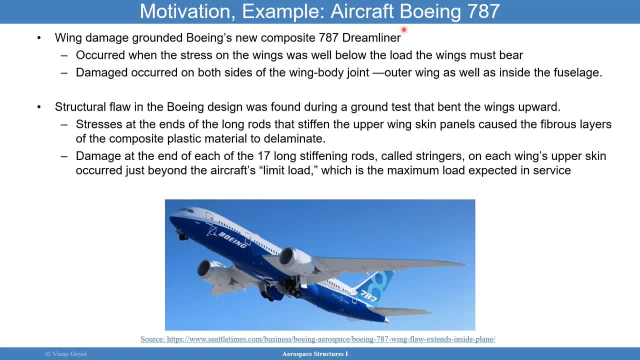 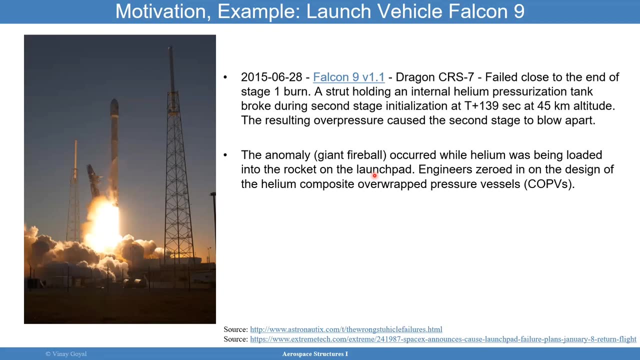 And so you can see how This Caused significant amount of delays in the Boeing 787 Dreamliner program. Another example is the motivation behind why we're studying this is there and it's not going to go in this course, and trying to solve these problems is to show you that structural failures do occur, and that therefore motivates the need for learning some of this material. 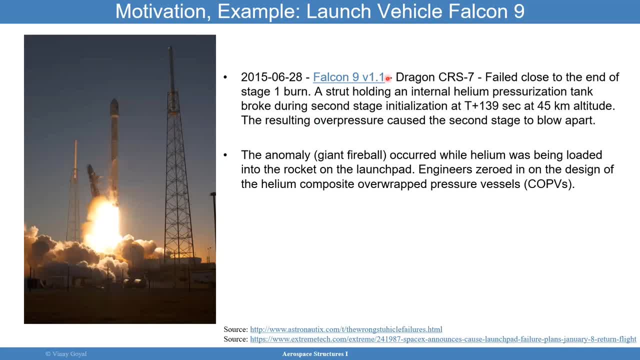 In 2015.. Uh, the Falcon 9, B 1.1 design carrying the Dragon CRS-7 mission failed Um towards the end of stage one burn: a strut holding an internal helium pressurization tank broke during second stage initialization at T plus 139 seconds at 45 kilometers altitude. 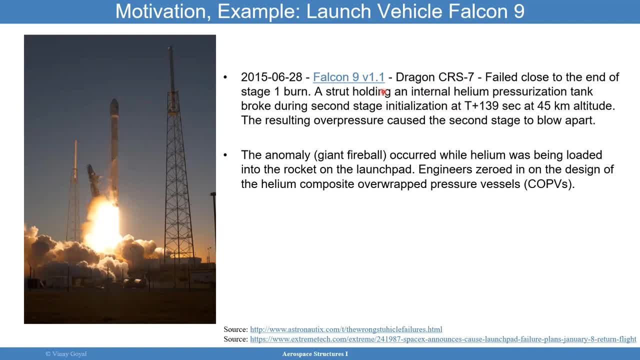 The resulting failure of this strut caused the second stage to blow apart, And this scenario here is described in the source here at the bottom You can link. you can go to that link and study this more. But there's also a second anomaly that occurred. 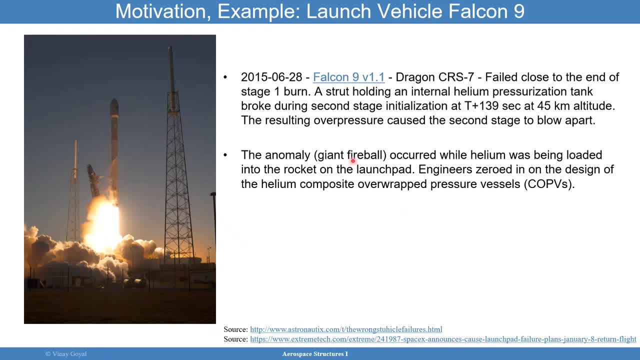 It was a giant fireball during the launch pad on the launch pad, when the vehicle was on the launch pad preparing from some testing And the helium being loaded into the rocket caused a failure And the engineers at SpaceX zeroed in into the composite, overwrapped pressure vessels. 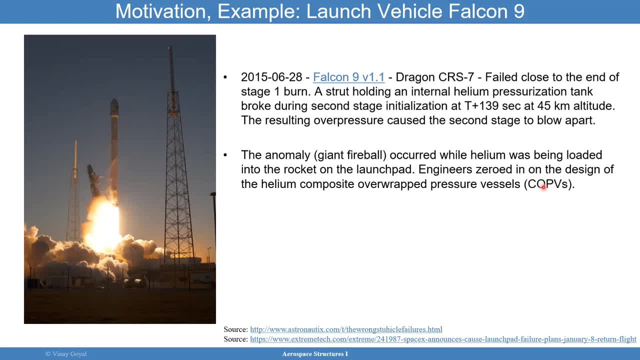 The COPVs is a topic I cover in part two of this course, the second part of this course, And so that's also linked here at the bottom For you to study more. The bottom line is that aerospace structural design allows you to understand the failure modes of the system. 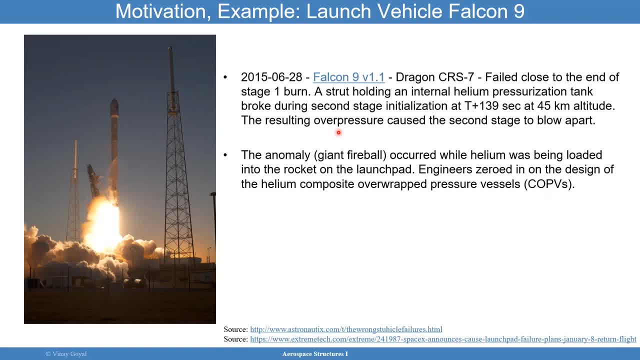 It allows you to learn how to prevent these failures from happening. But even when you try your best, it doesn't mean that when you try your best, failures will be precluded. There's still the potential for failures to occur, because failures Are are complex in nature and it can be missed by analysis approaches. 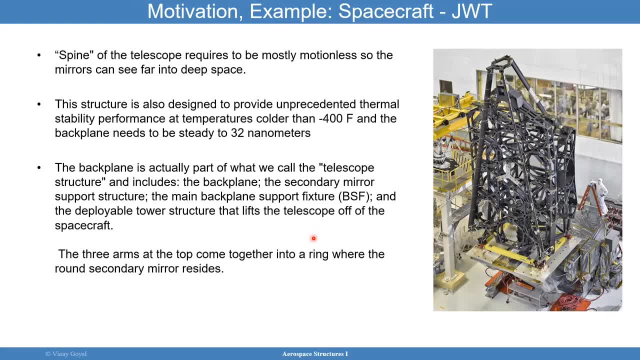 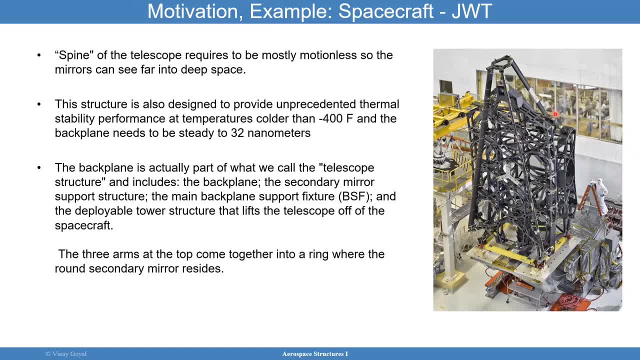 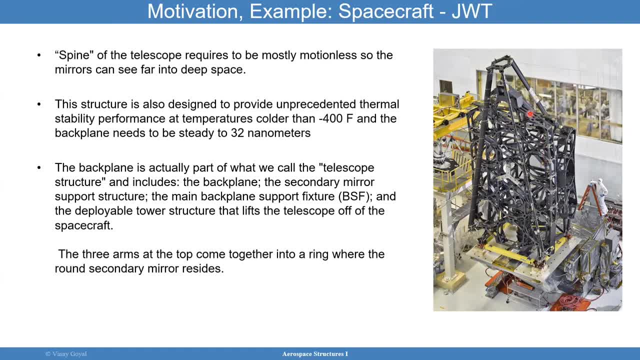 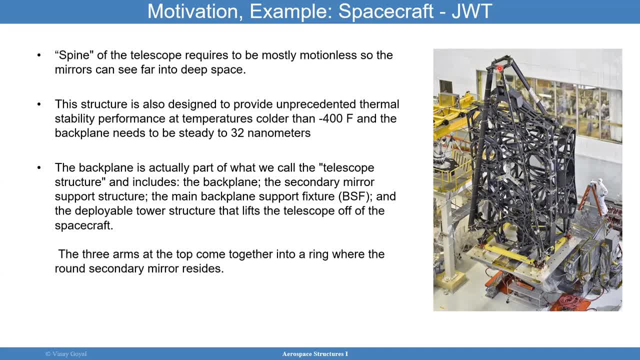 And it almost needs to be motionless so that the mirrors are attached to his backbone- can see far into deep space. And it almost needs to be motionless so that the mirrors are attached to his backbone can see far into deep space. And it includes the secondary mirror support structure. 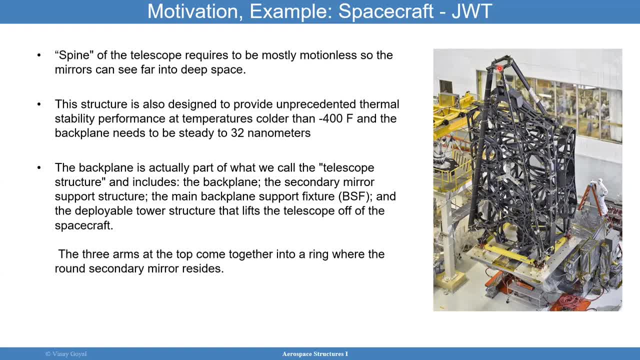 It includes the deployable tower structure And you know, all this has to work well together And it's no surprise that the James Webb Telescope has experienced delays, Because these are very ambitious and very complex programs. The course outline is as follows: We're going to go through the overall design process for Aeris. 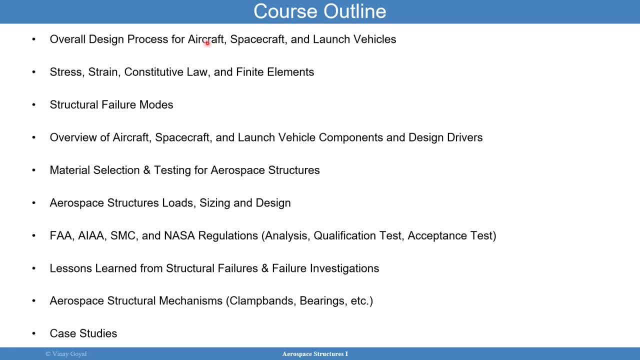 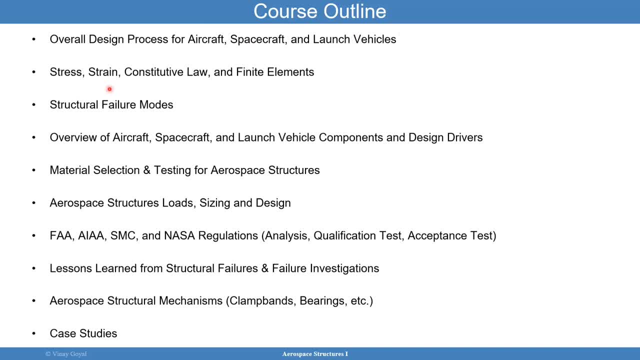 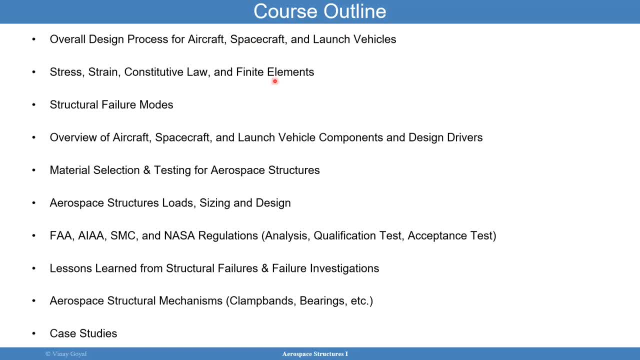 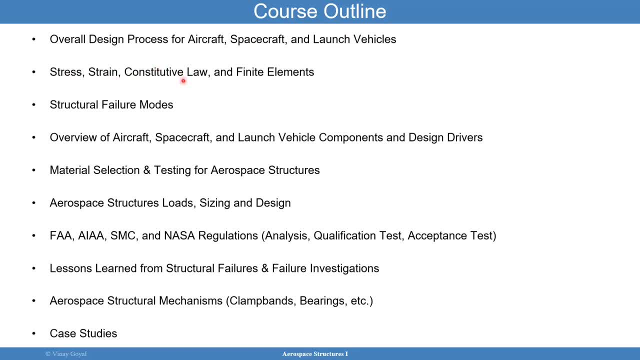 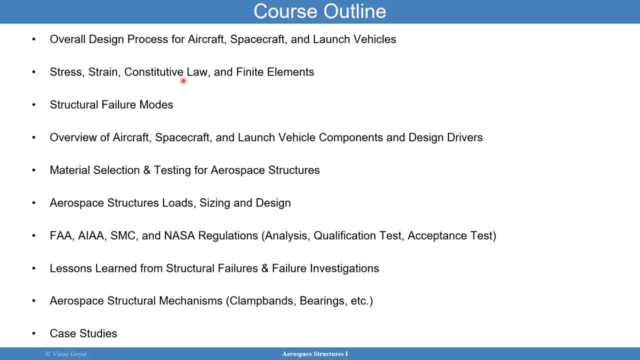 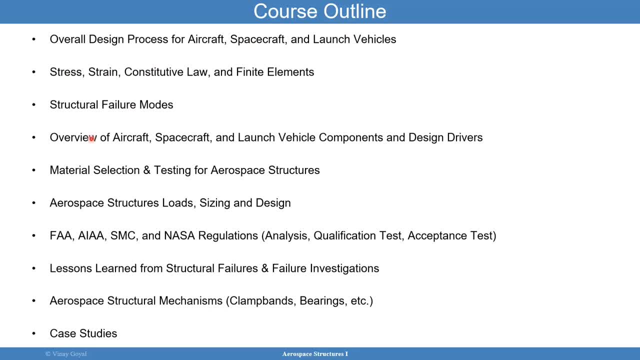 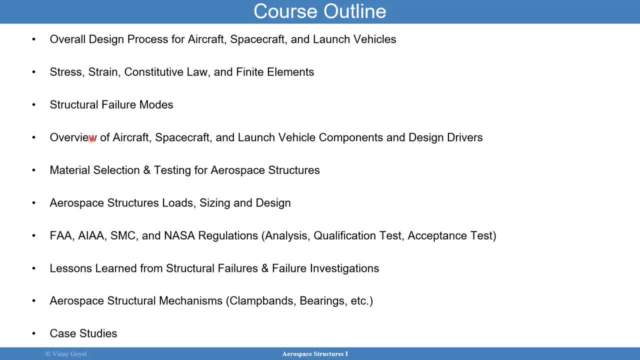 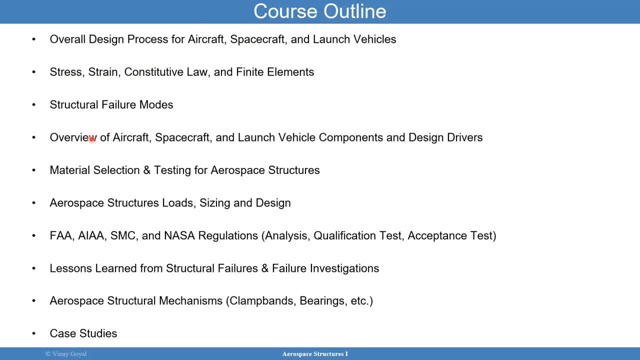 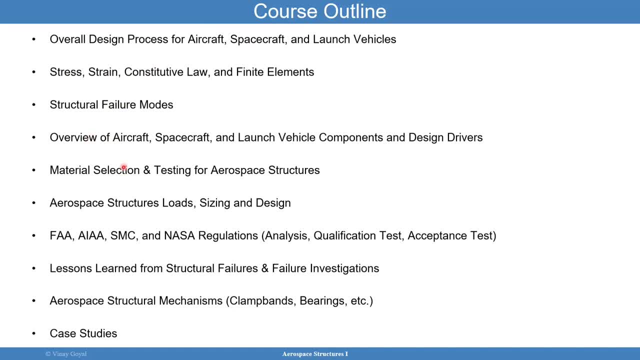 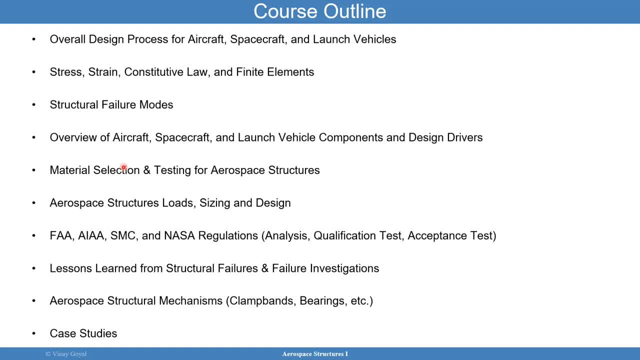 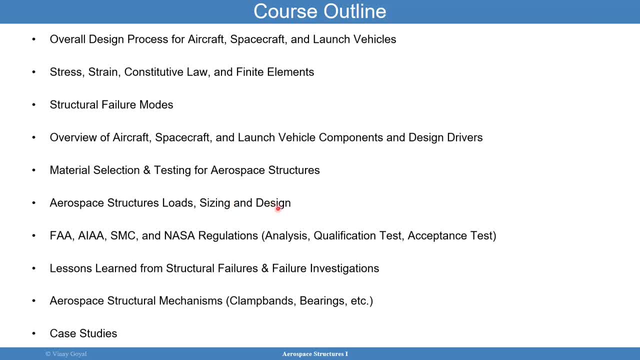 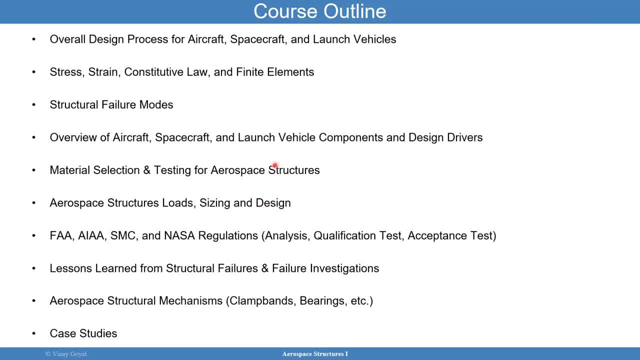 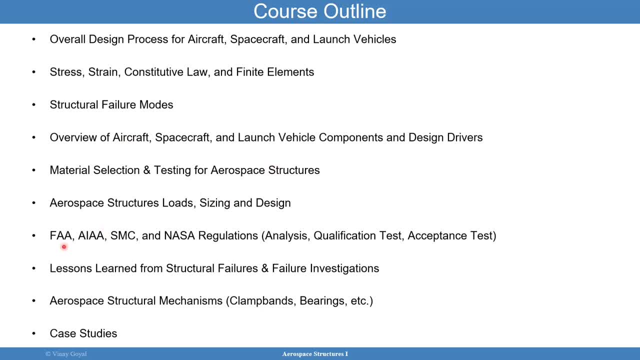 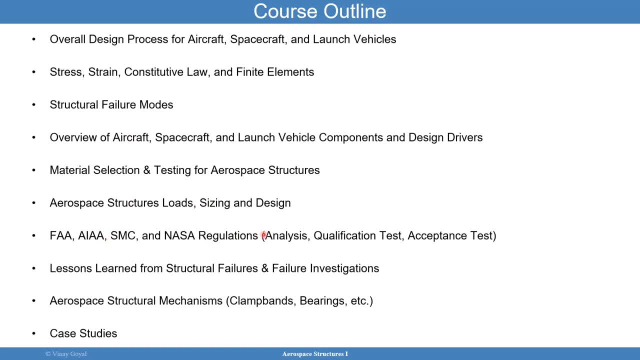 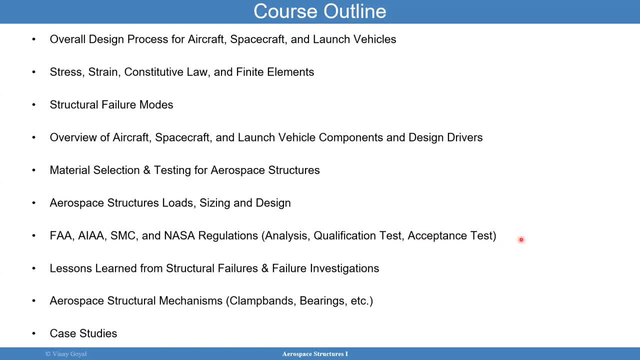 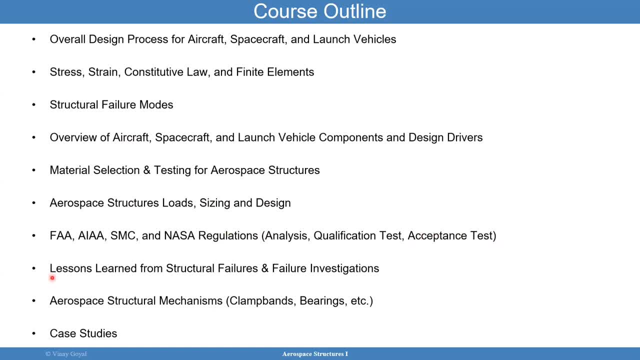 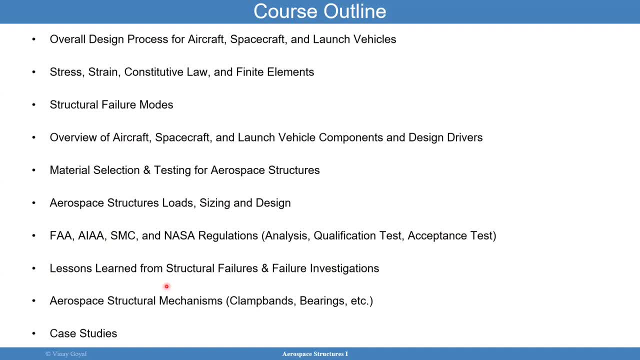 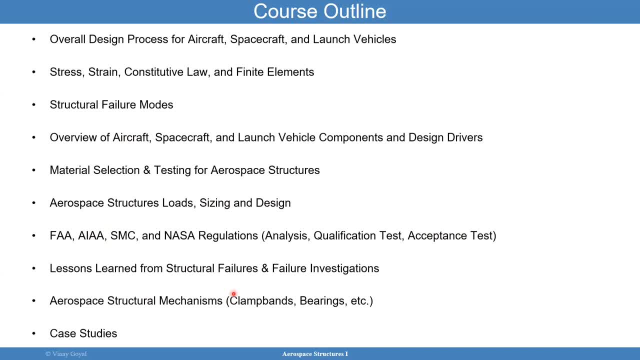 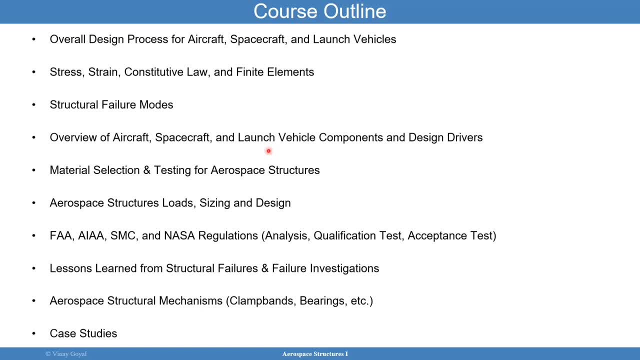 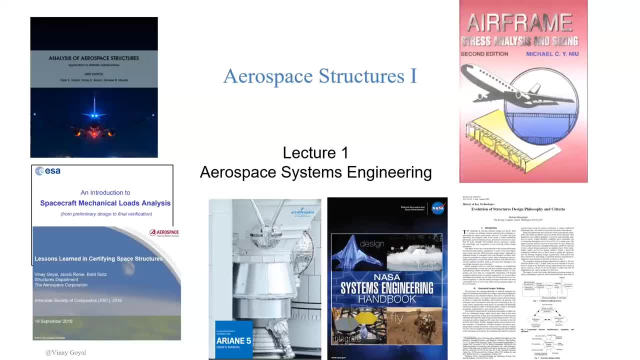 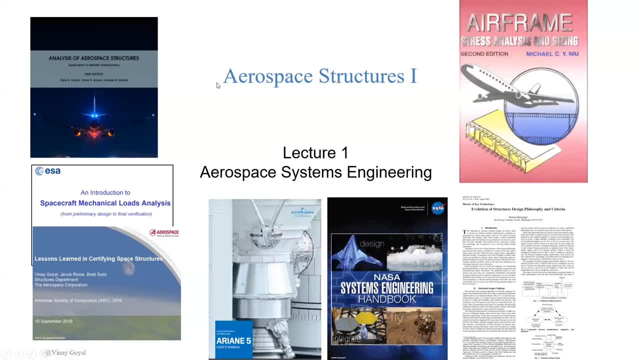 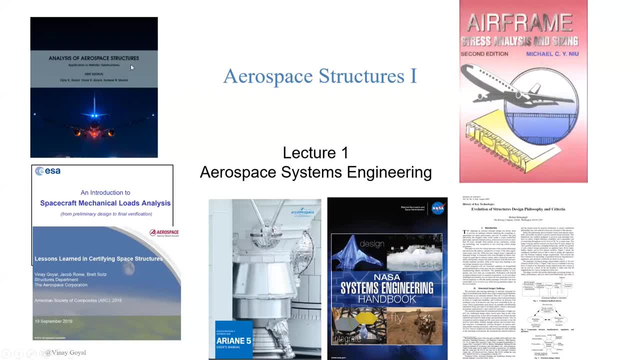 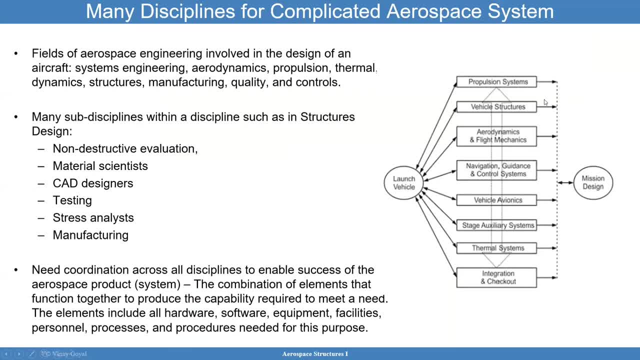 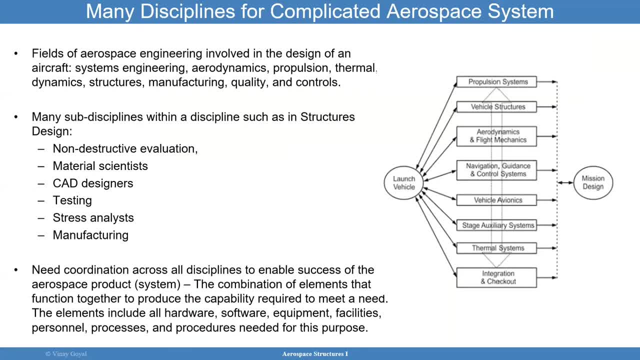 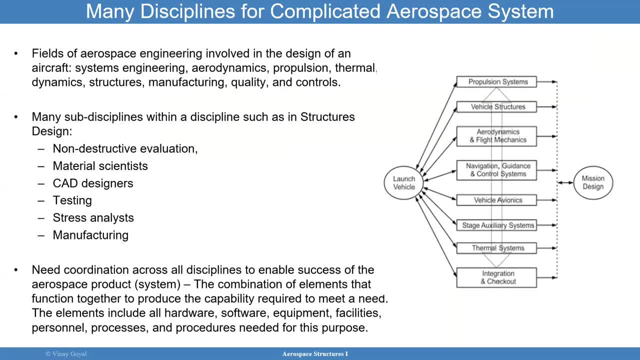 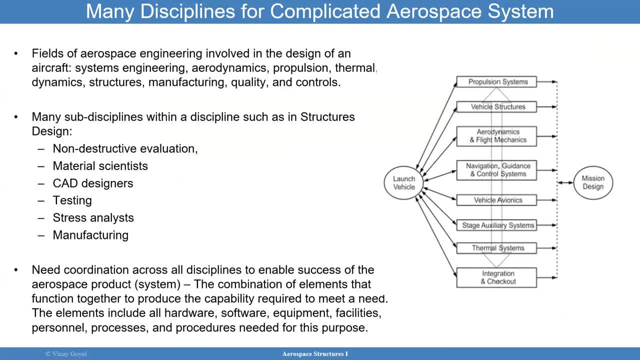 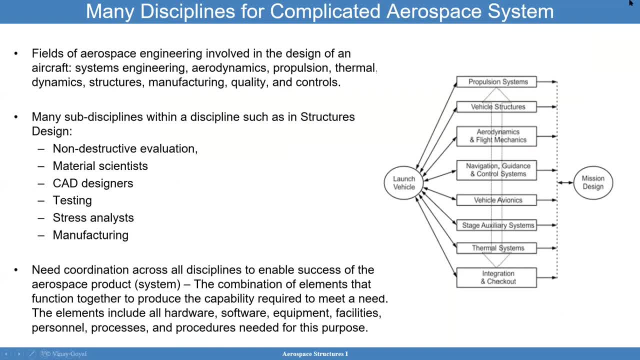 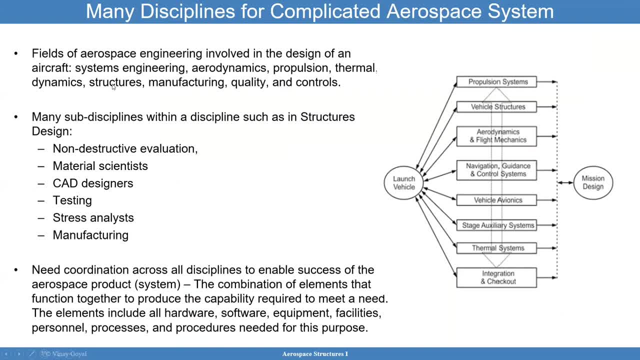 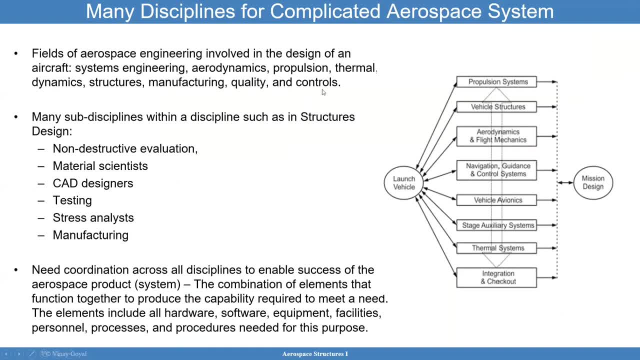 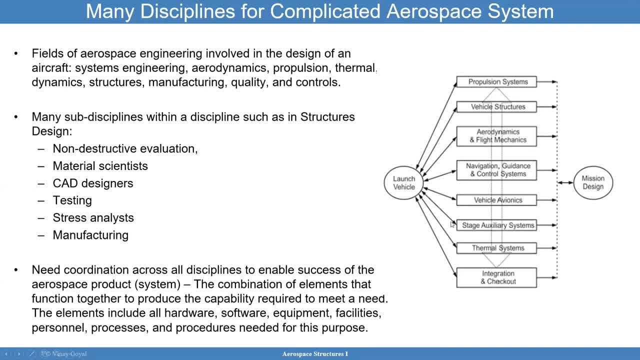 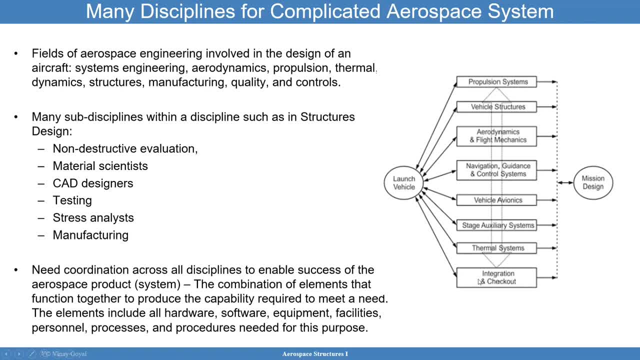 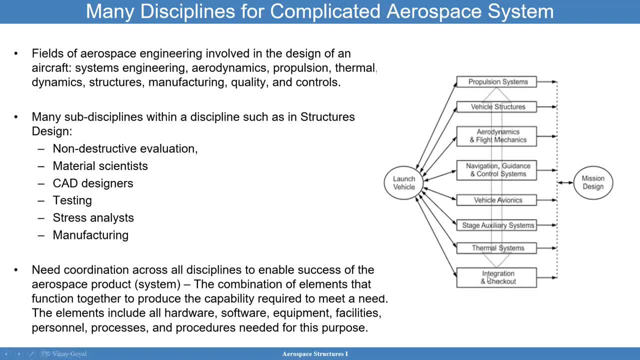 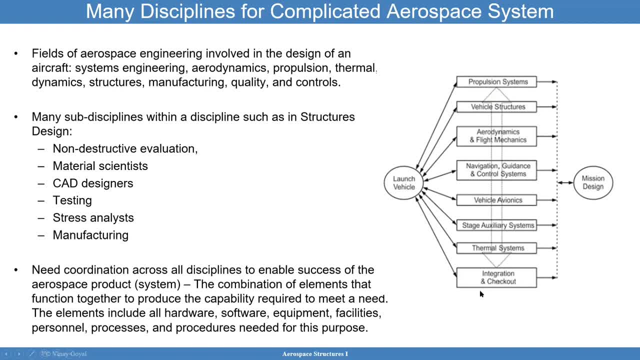 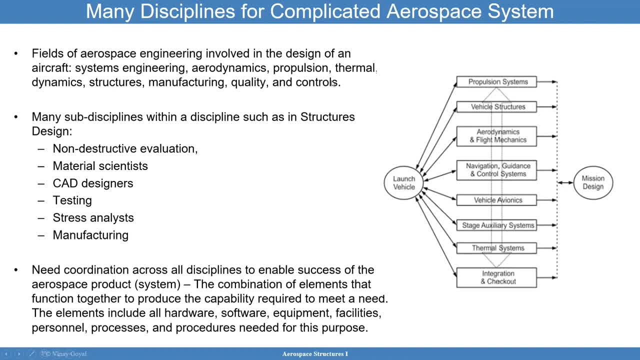 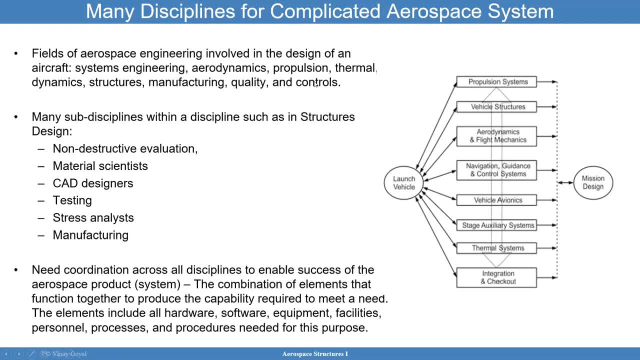 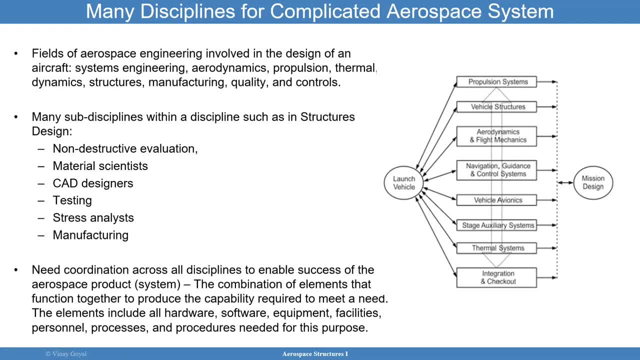 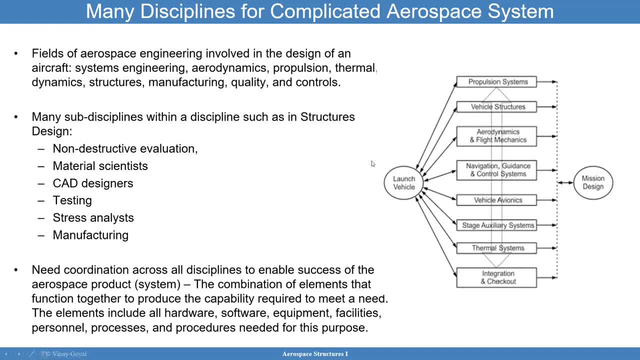 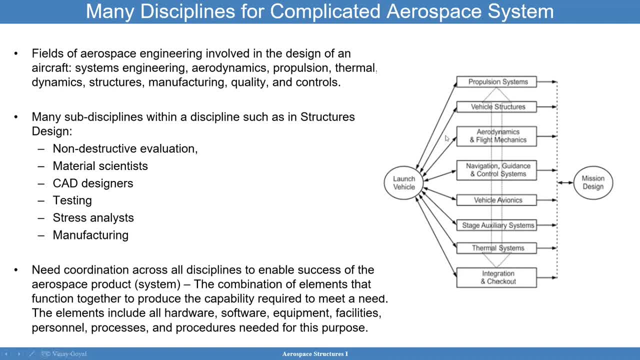 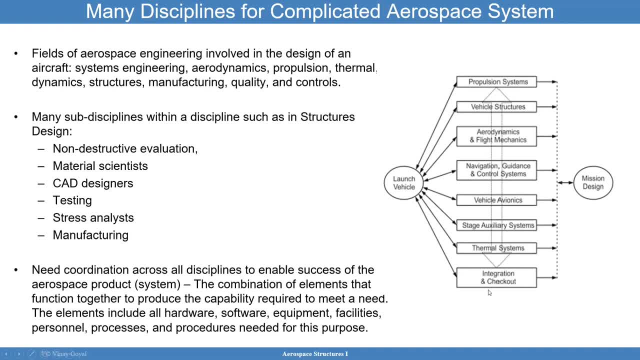 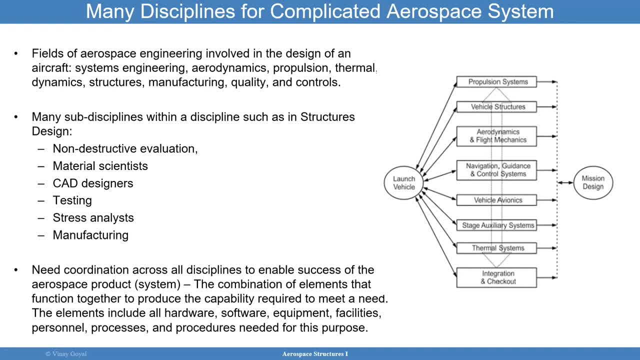 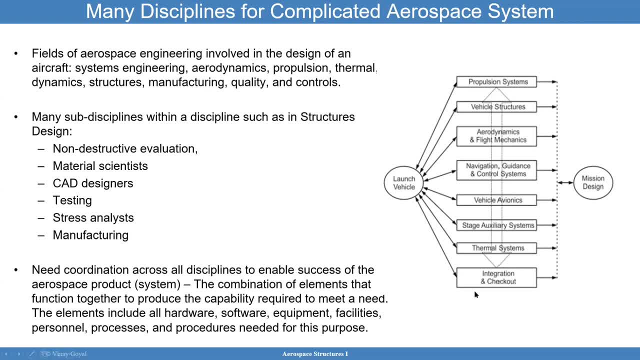 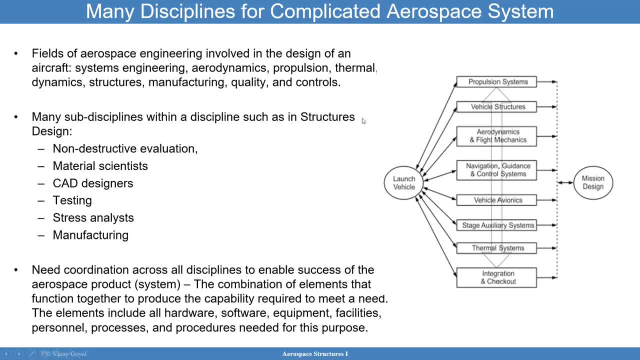 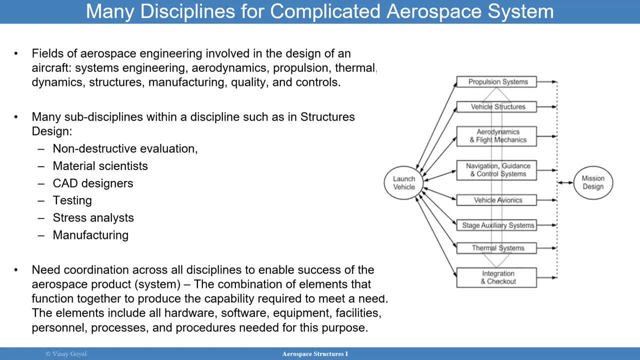 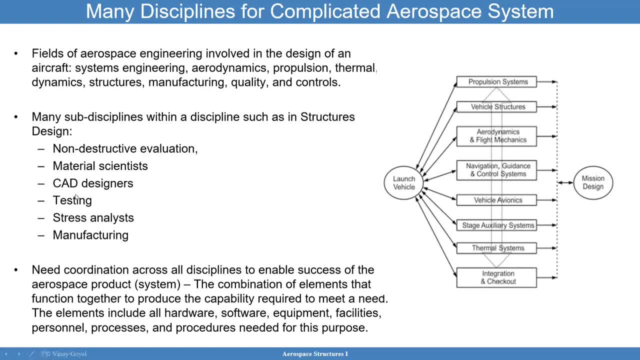 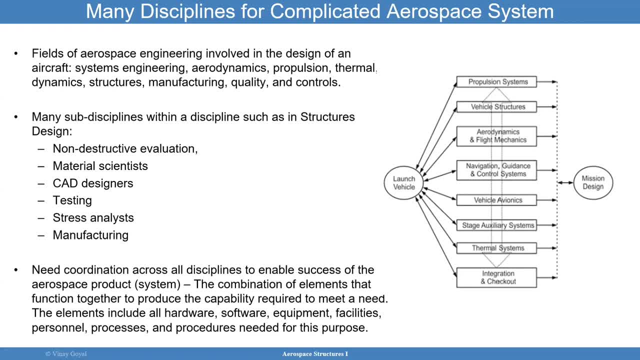 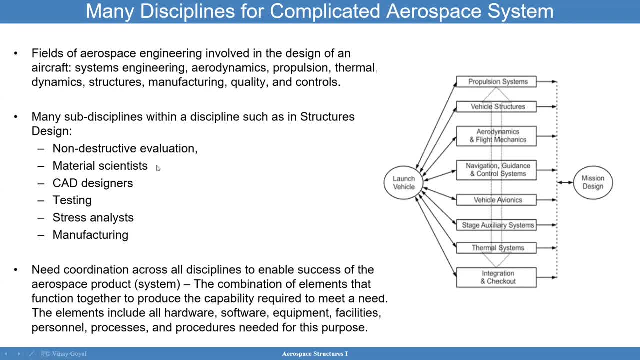 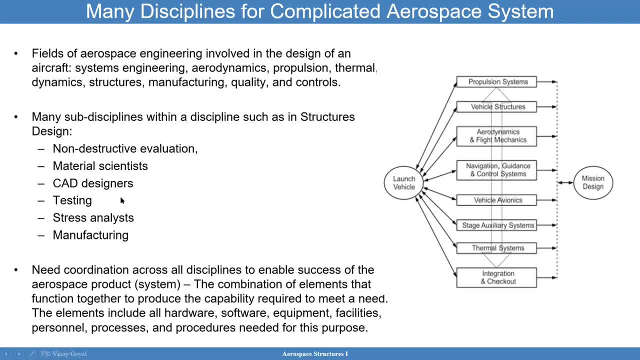 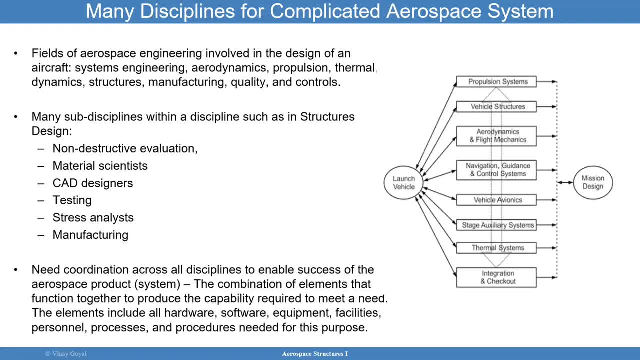 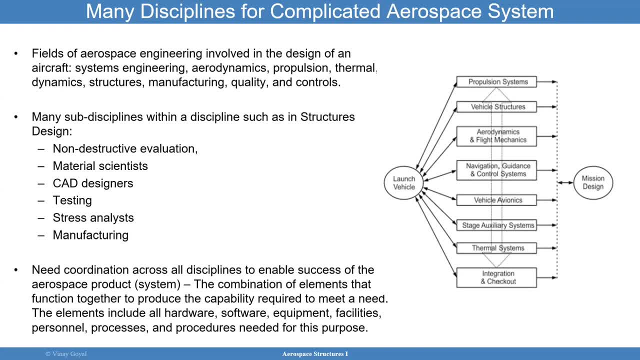 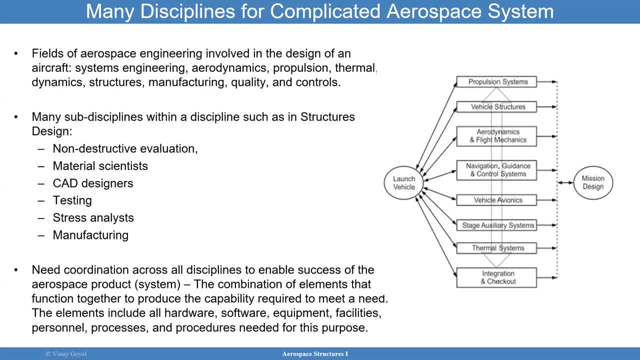 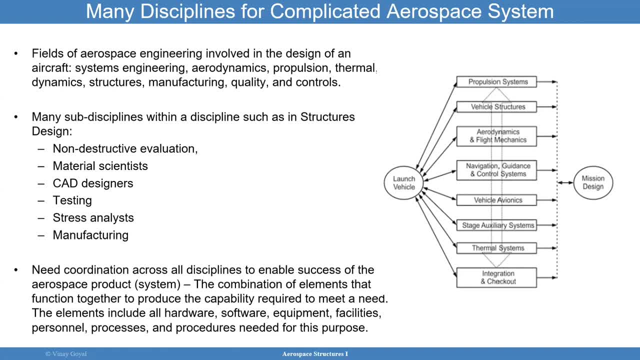 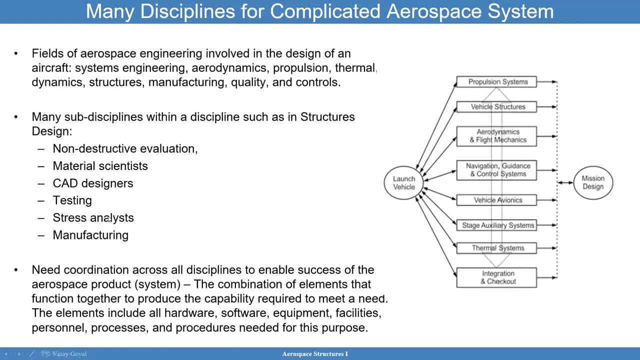 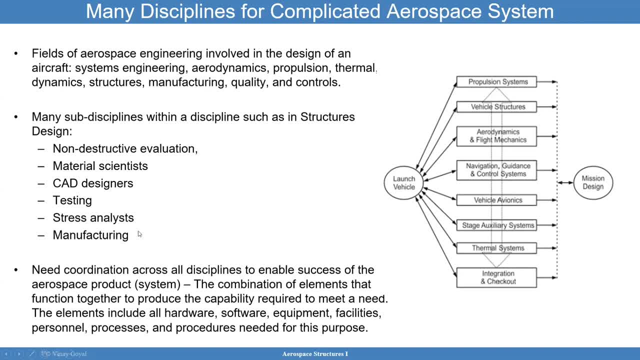 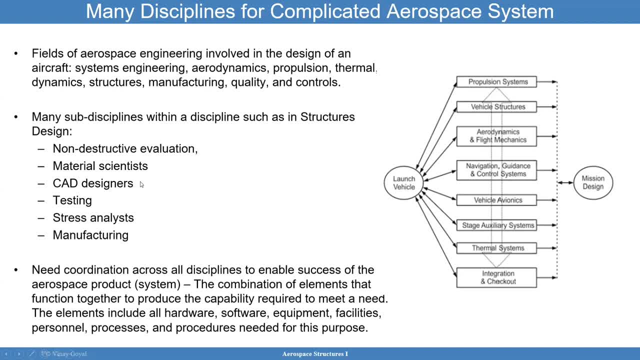 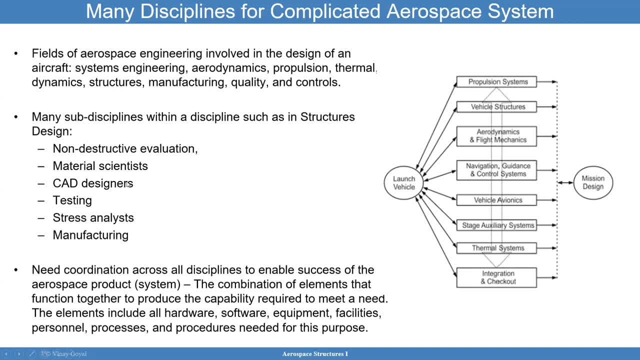 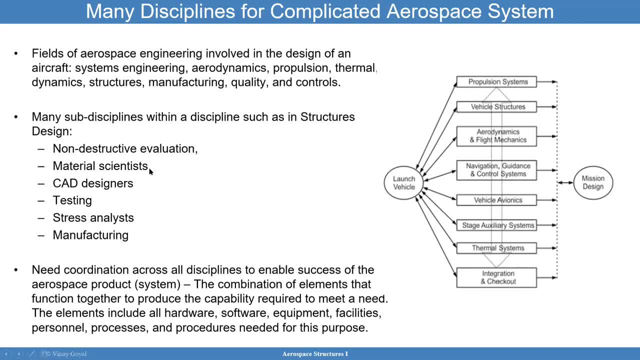 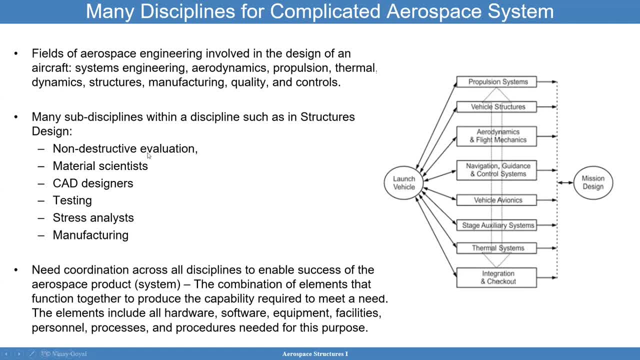 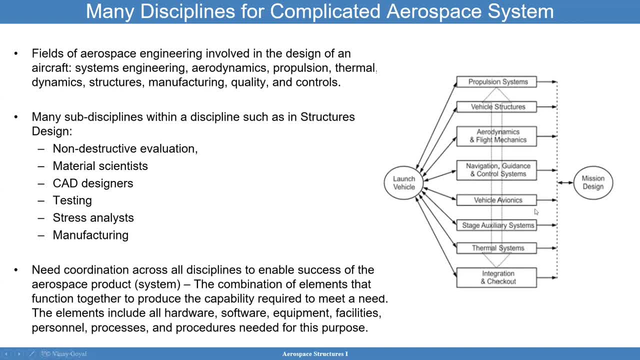 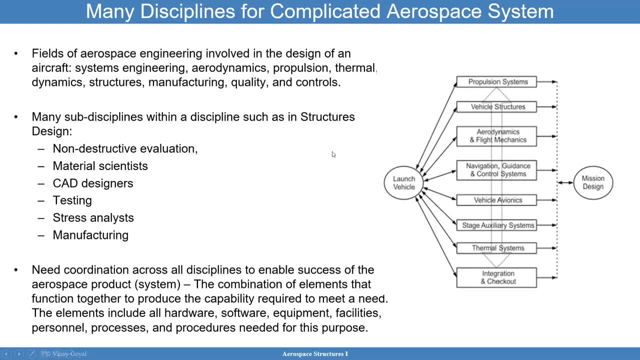 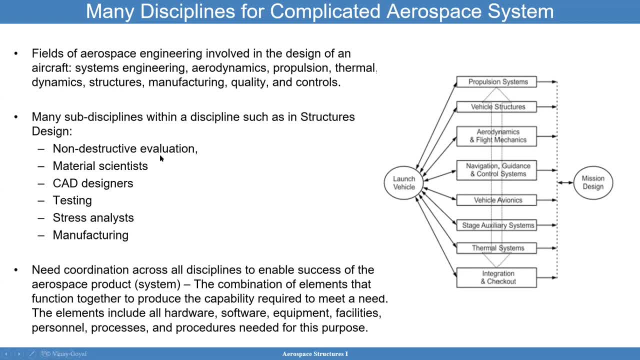 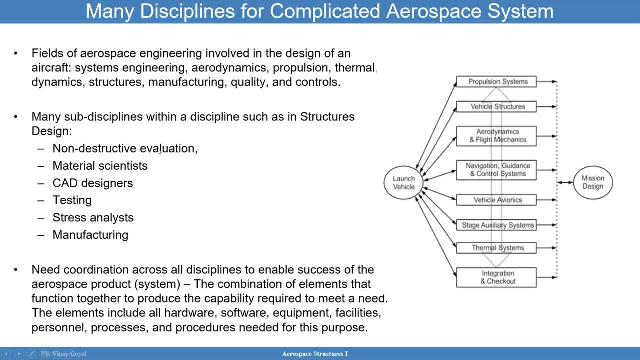 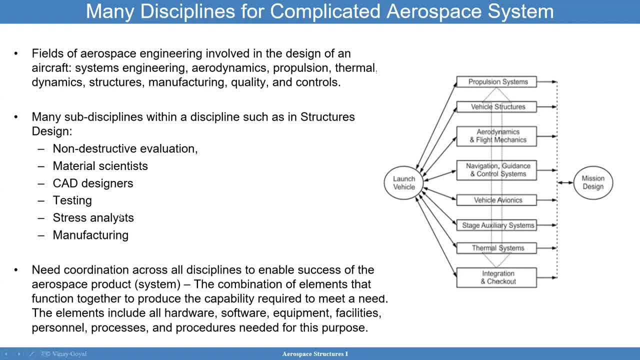 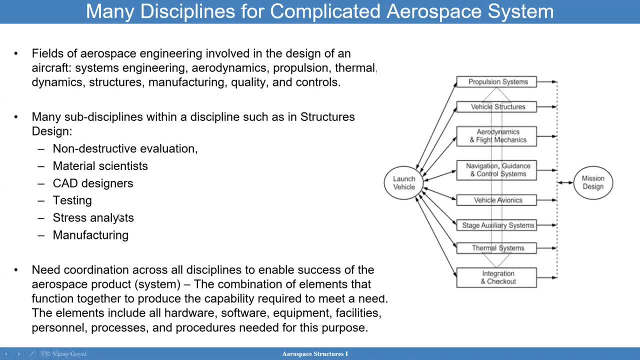 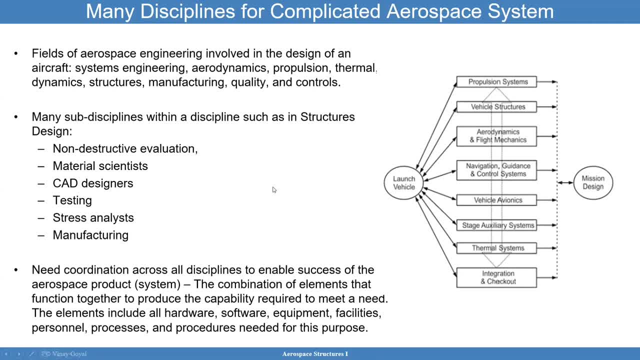 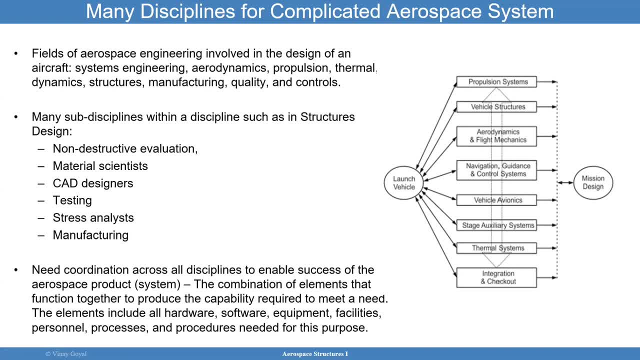 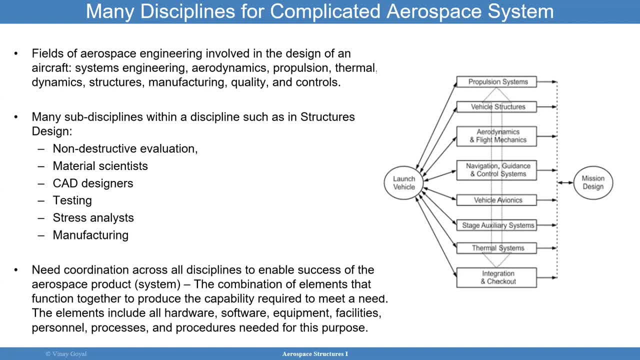 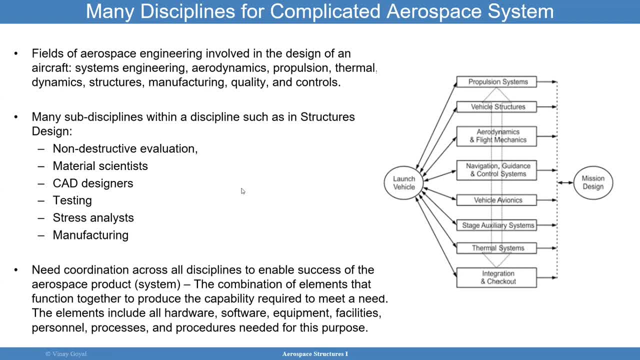 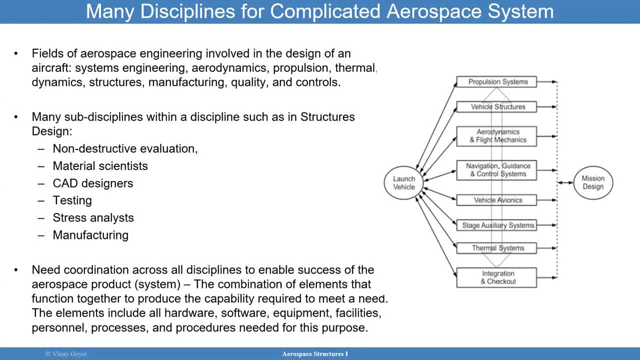 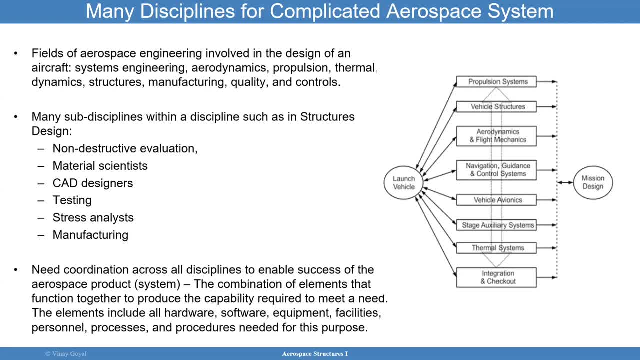 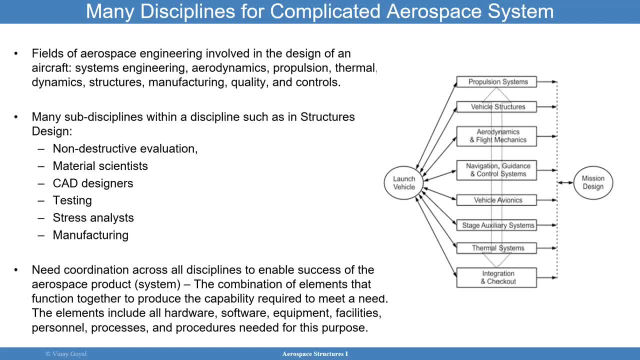 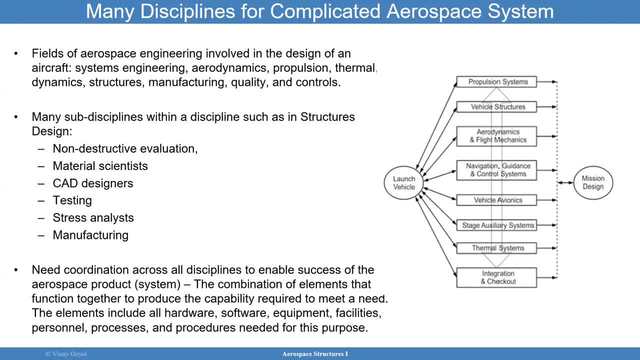 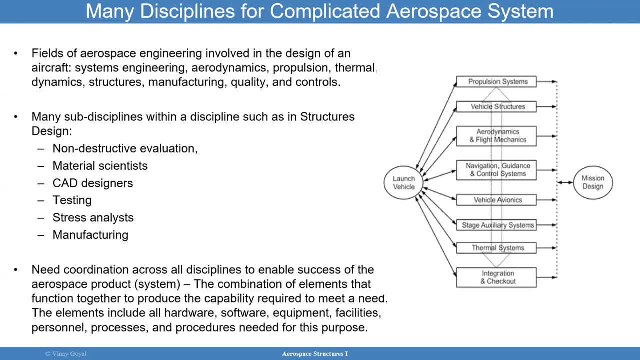 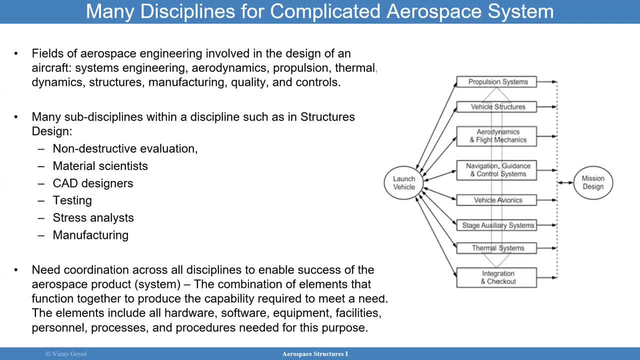 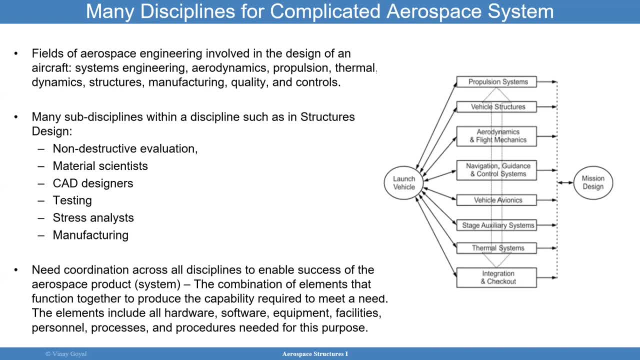 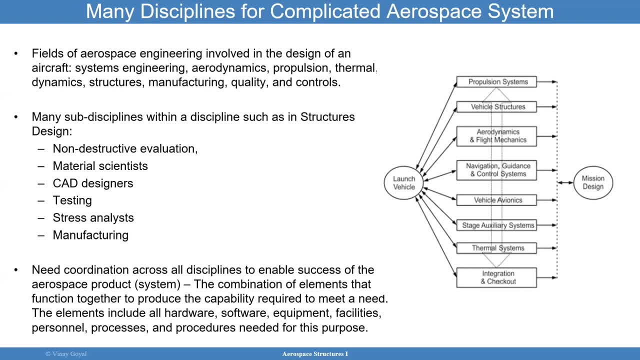 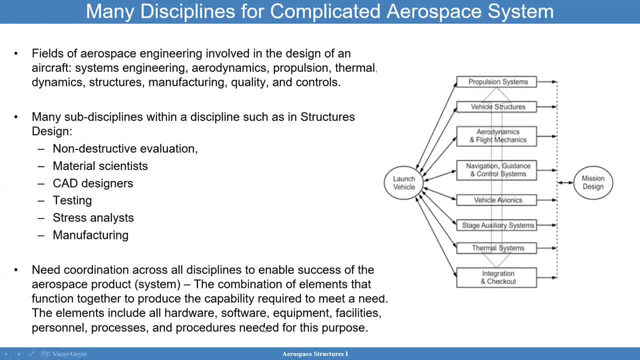 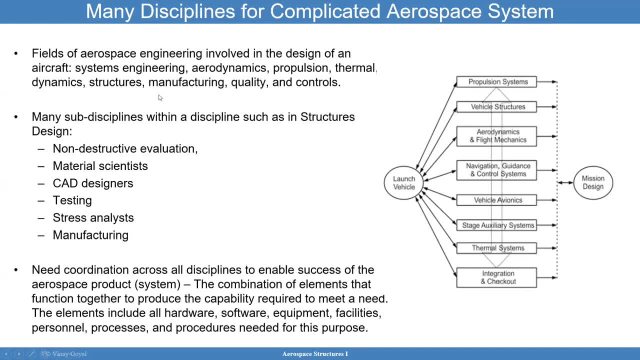 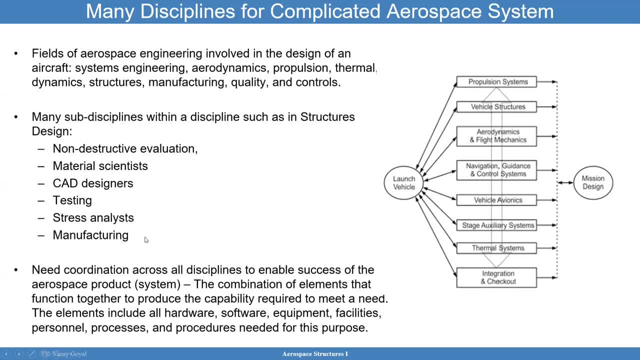 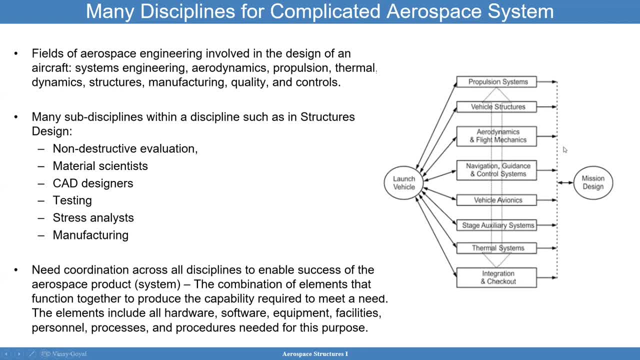 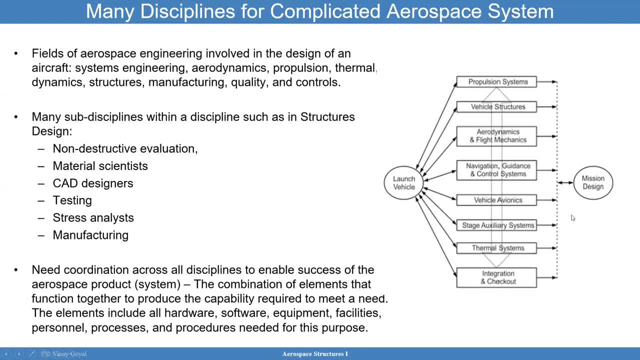 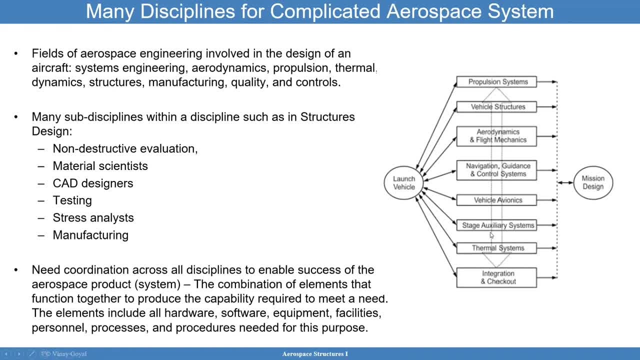 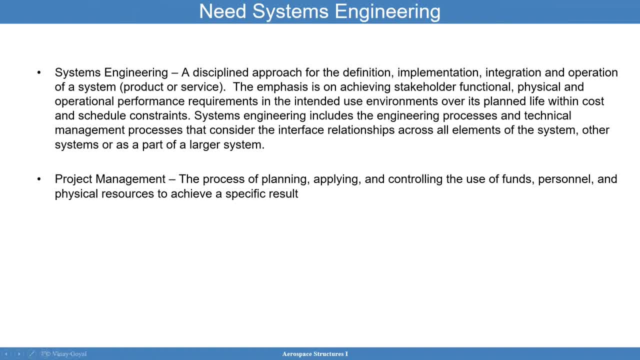 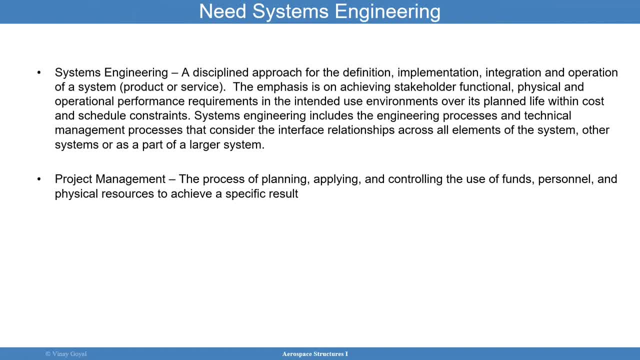 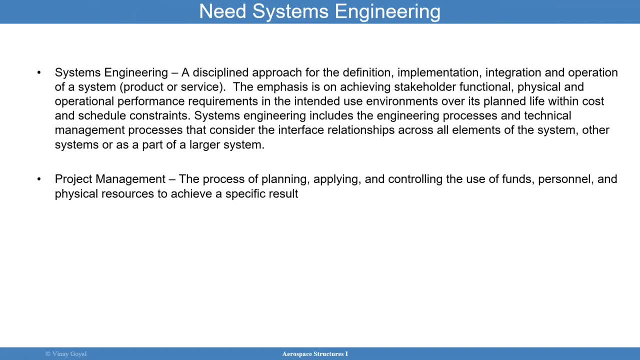 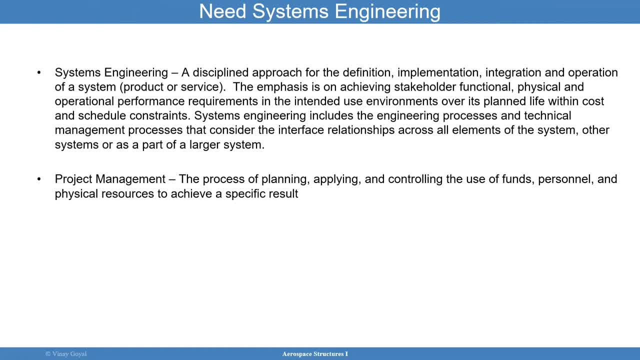 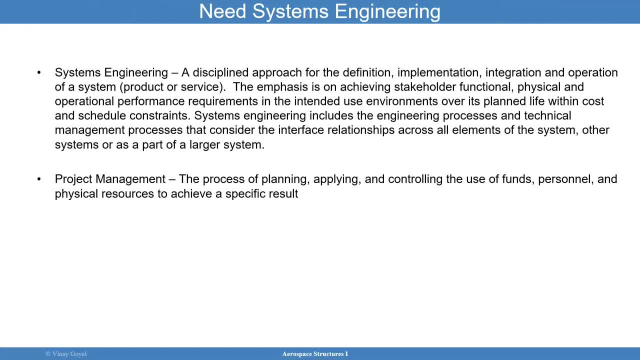 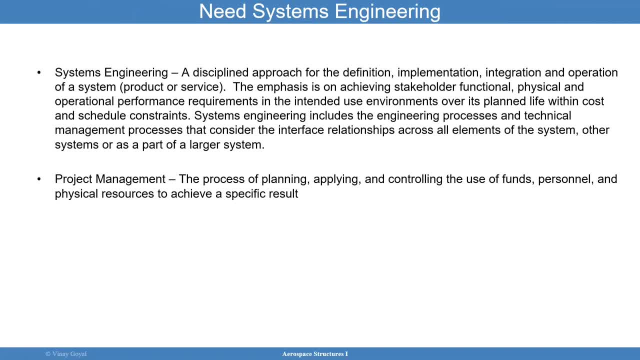 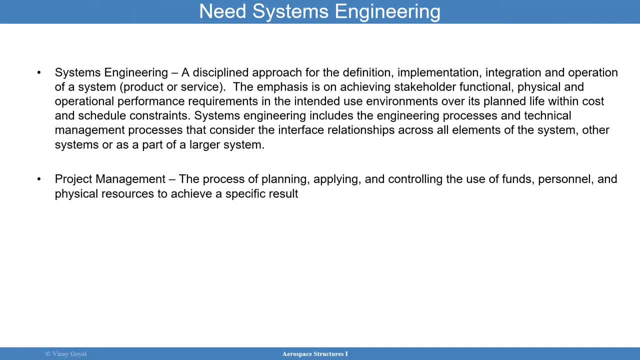 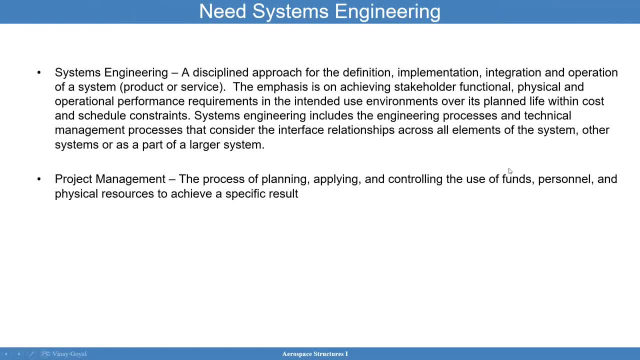 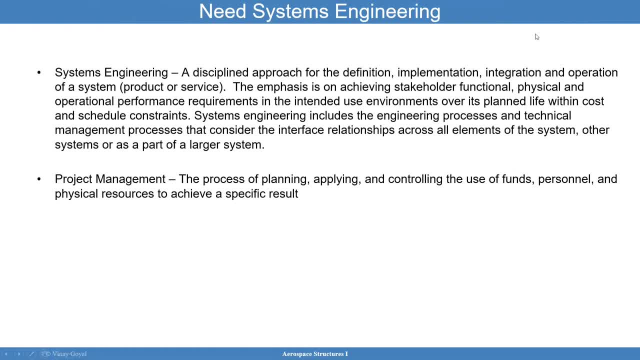 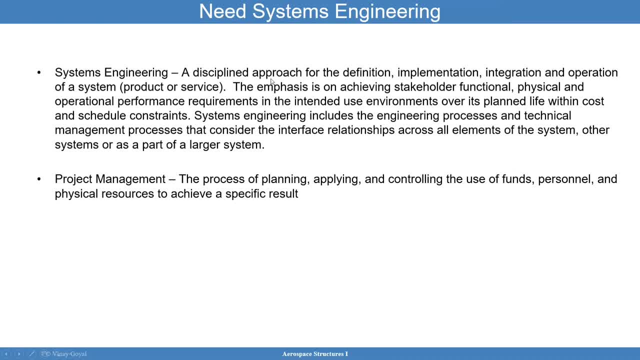 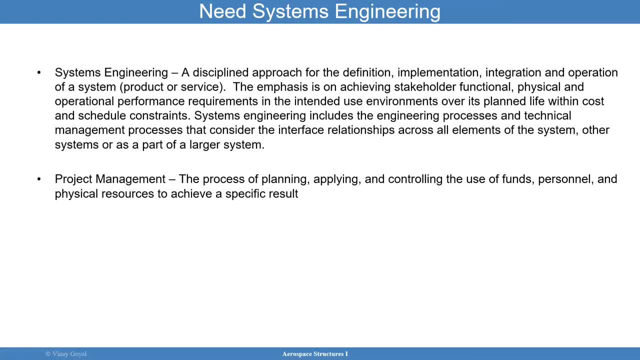 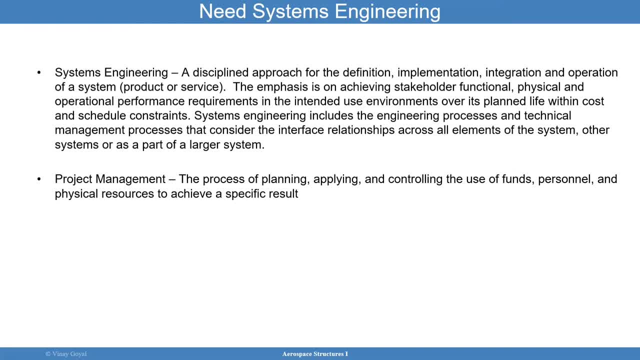 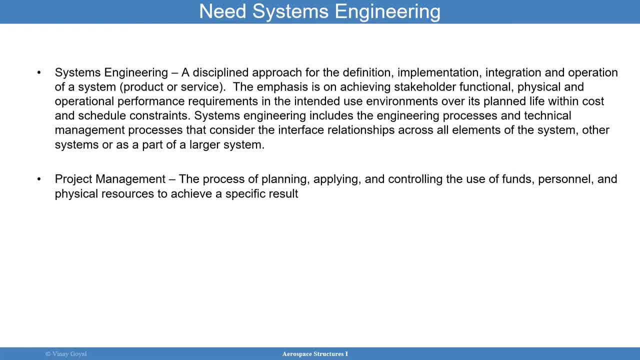 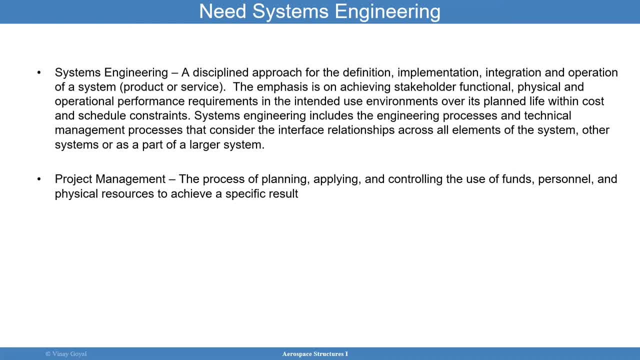 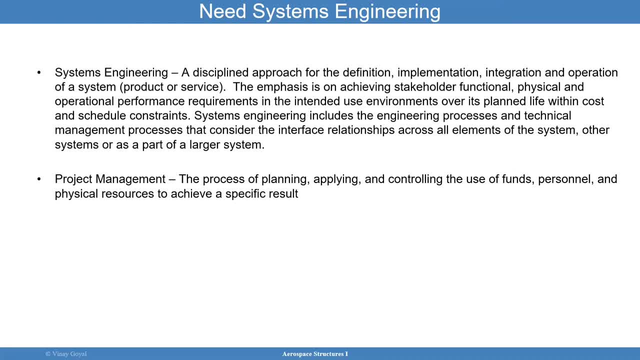 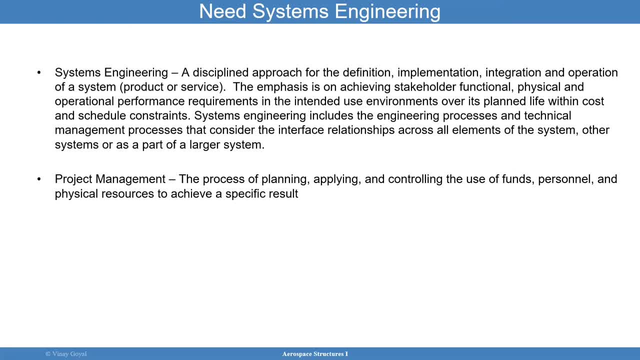 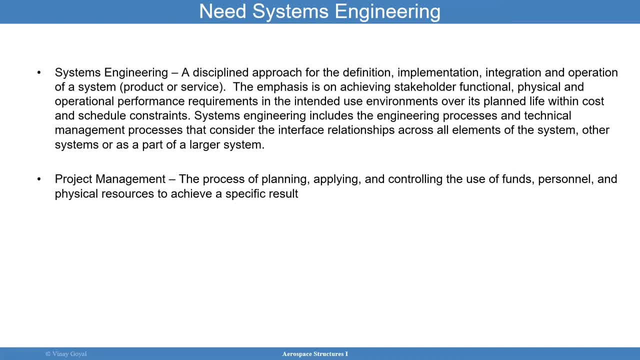 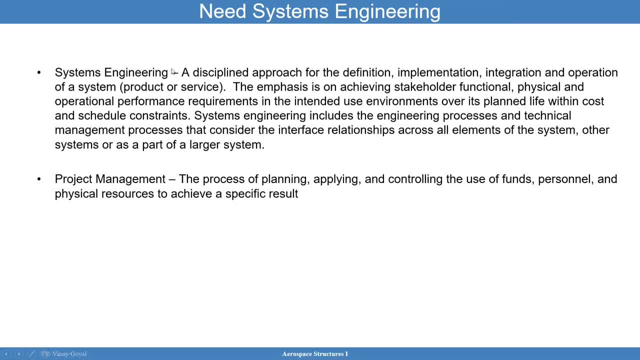 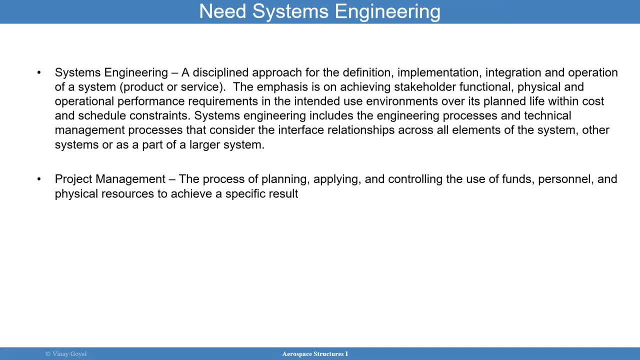 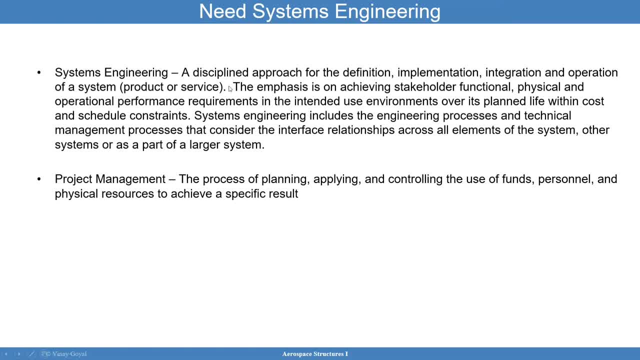 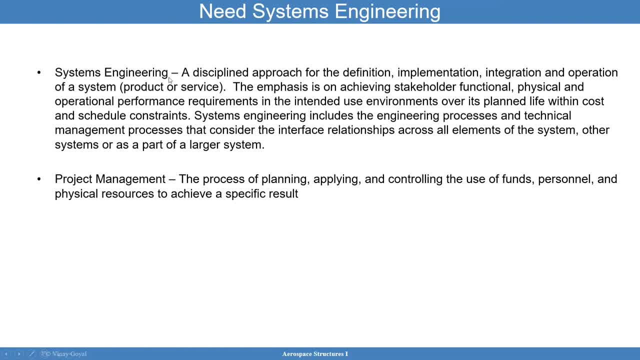 We're going to go through the overall design process for Aeris. We're going to go through the overall design process for Aeris And systems engineering relies a lot on the project management and that's a process of planning, applying and controlling the use of funds, personnel and physical resources to achieve a specific result. 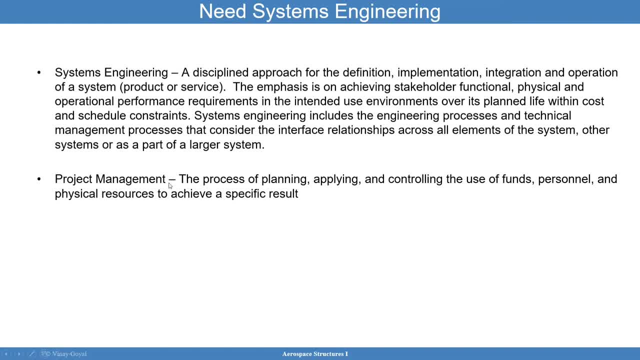 If I don't have good project management, the project is likely going to be a failure. and I have to have some planning. I have to have controlled use of funds. I have to make sure that the efficiency that's embedded into the planning of the project is optimal. 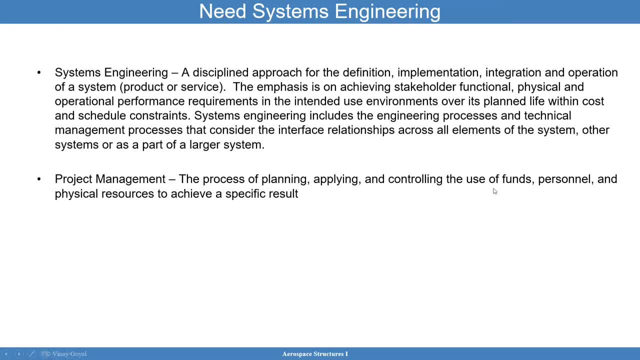 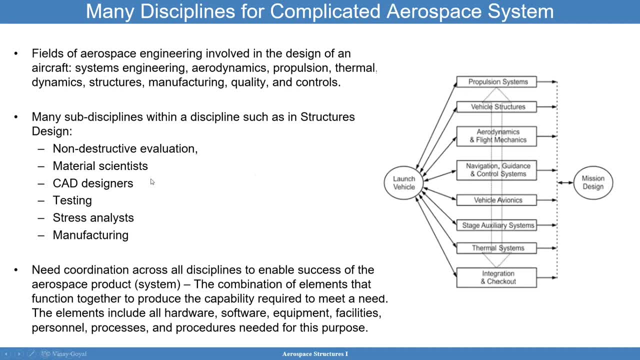 I have to make sure that the teams are talking to each other, Otherwise the project will be a failure, And so then also the systems engineering needs to make sure that the interfaces between the disciplines are working well and they're communicating. For example, if the structural team 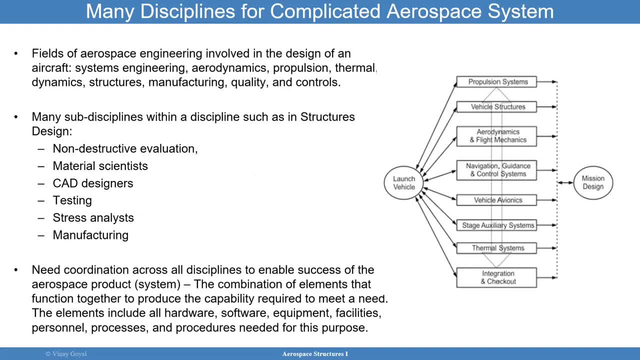 is designing an aircraft or launch vehicle component to 150 degrees Fahrenheit, but the thermal team worked with a fluid mechanics team and determined that the temperatures that the system is going to see is closer to 300 degrees F. Well, if these teams are not communicating, 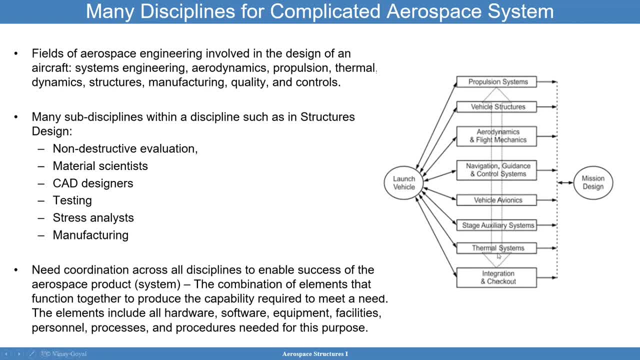 the structures team will complete their design and the thermal team will complete their design, And the thermal team will have not communicated to the vehicle structures team that there is an issue indeed, for example, that that should be looked at again. And so all these disciplines have to constantly talk to each other to ensure that the requirements 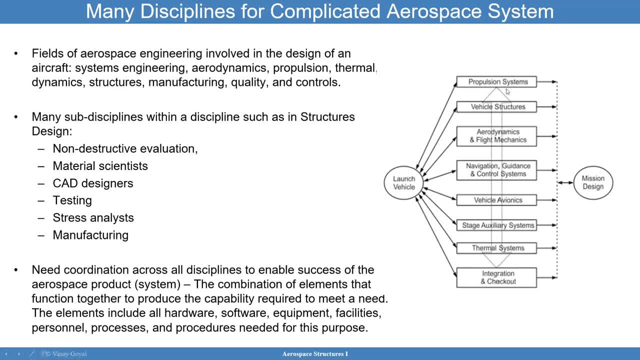 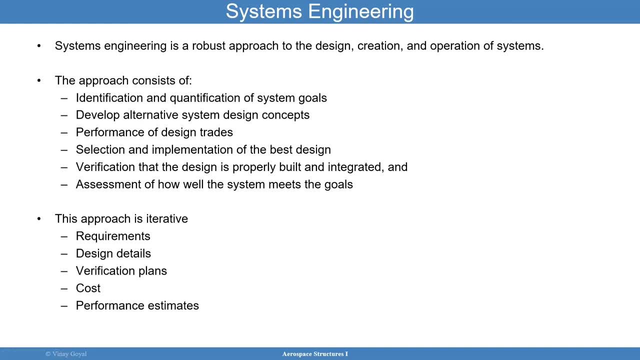 from one discipline to another are getting flowed down properly so that their interfaces are smooth and that we can make progress in the designs. So the systems engineering is a robust approach to the design and creation of our operational systems, And the approach in systems engineering relies on several key elements. 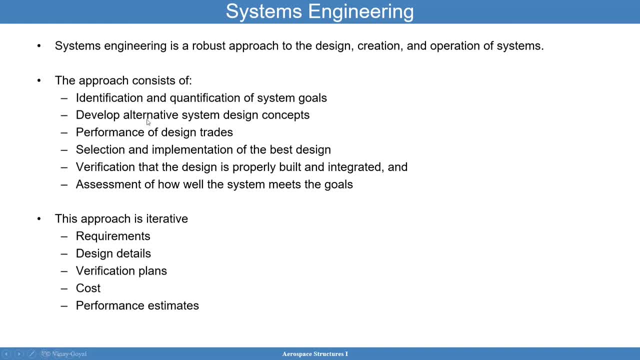 Identification and quantification system goals, develop alternative system design concepts, performance of design, trades, selection and implementation of the best design. So you may have many different designs, But if your need to downside the best design, that's what you want to do. 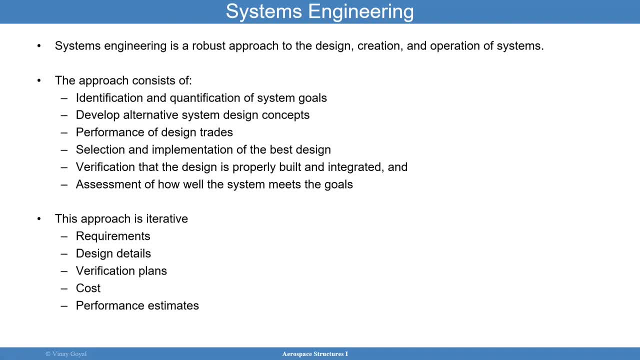 verify that the design is properly built and integrated and then perform an assessment of how well the system meets the goals. You do want to have alternative concepts for the design, because if you only put your eggs on one basket or one particular design, there's a potential that if that design does not put the design, 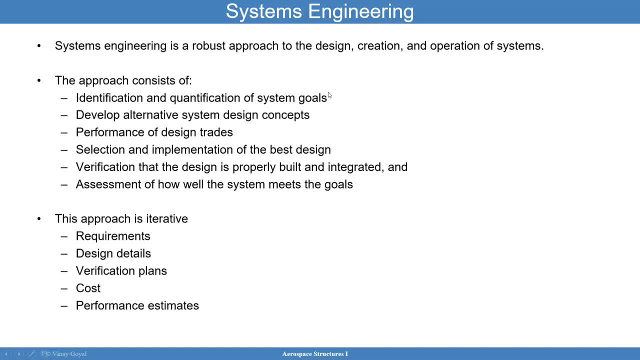 design does not play a part in that pan out. you're left with nothing. so it's important to entertain multiple design concepts that are strong, and then you do the design traits that allow you to down select to the best concepts, which then you can then mature further. the approach here is further. it is quite iterative. 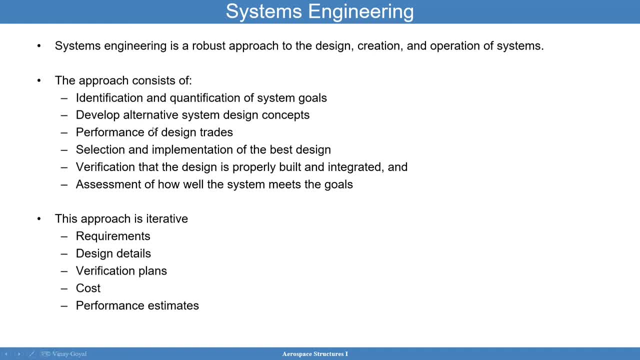 you have to iterate on the requirements, the design details, the verification plans, the cost and performance estimates. and when i say requirements, as an example, if i want a launch vehicle that needs as as a impulse, a specific impulse of some kind, say i need 350 isp for my launch vehicle design. that's a requirement. 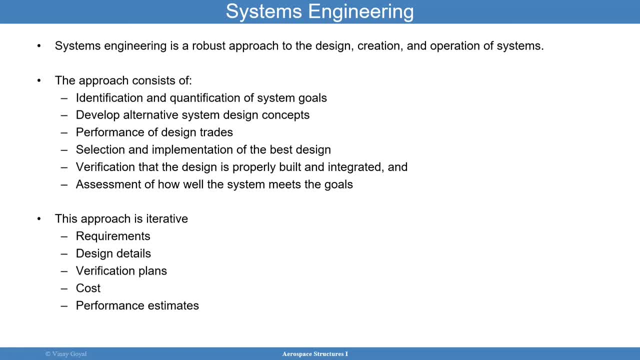 you have to iterate on the requirements, the design details, the verification plans, the cost and performance estimates. there's a system has to meet. if i have an aircraft i'm going to design and the aircraft design has to fly from here to a country that's, for example, in africa. 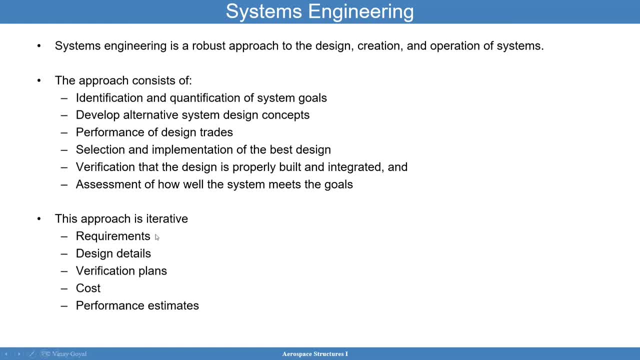 non-stop. that's a requirement. i have to make sure the aircraft is capable of doing so. so those are the kinds of requirements that need to be put in place to really understand whether your design can meet those requirements. those are functional requirements, performance requirements that need to be met. 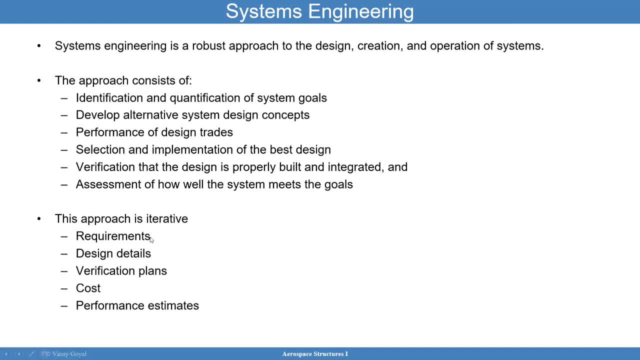 not to be confused with regulatory requirements like from the faa, making sure the requirements that the system meets faa requirements different from functional requirements. you also may need to iterate on the design details and the cost and performance estimates. these things may be invalidated by new findings during the 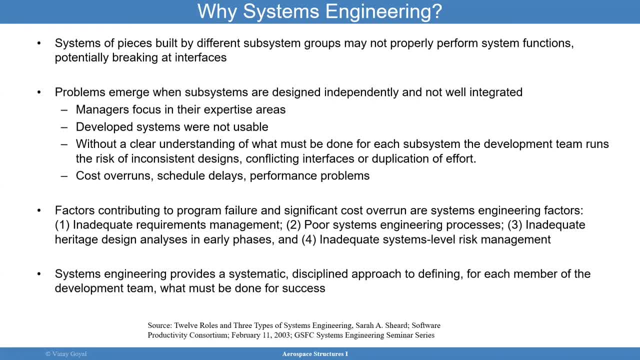 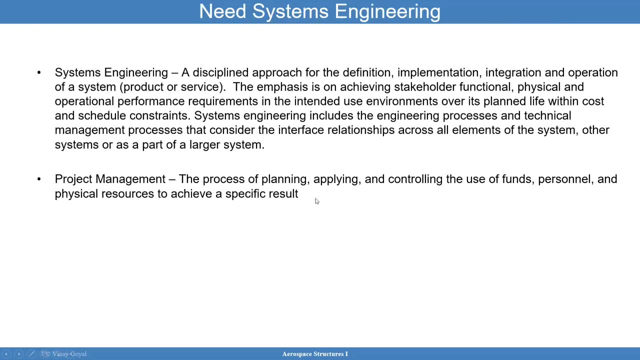 during the process of the design. so why do we need systems engineering? the systems of pieces are built by different subsystem groups and may not properly perform system functions, and so at those interfaces i need smoothness, i need to know that these subsystems are working well together. now i'm not just talking about the 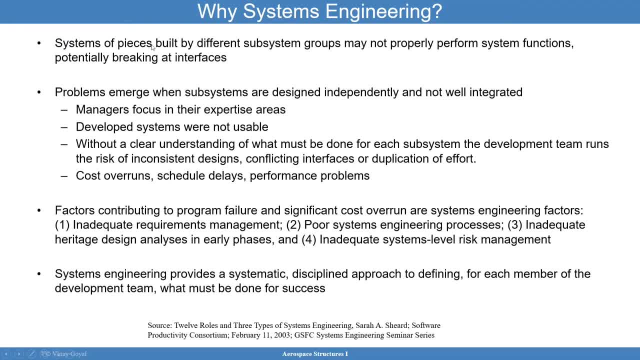 disciplines, but i'm talking about the pieces that are being built. for example, if i have the team that works on the engines and i have the teams that works on the rotor system and i have another team that works on the nose, i may have a multidisciplinary approach for each of those. 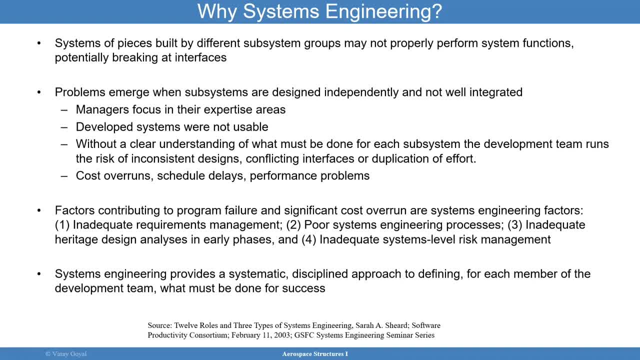 subsystems, but i need to make sure those Subsystems can come well together as well. So not only I need to make sure that Each subsystem is working well together as a team, I also need to make sure that The interfaces where the subsystems come together. 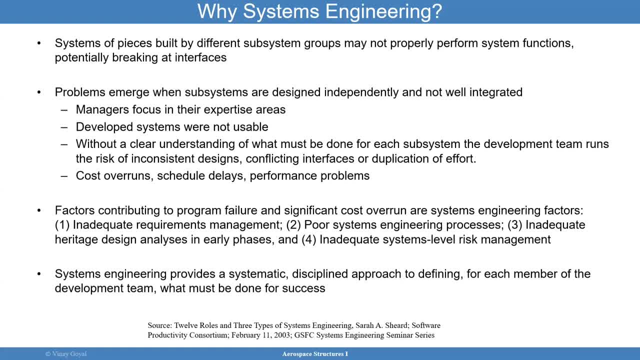 That we don't have an issue there at those interfaces. The problem really emerged typically when subsystems are designed independently and are not well-integrated. Why that happens is because managers will focus in their areas of expertise or in their subsystems arena And forget how their subsystems has to work well with others. 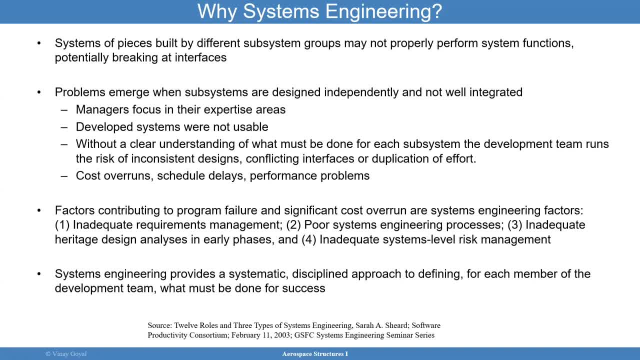 They may develop systems that are not even useful to them By the other subsystems. So we got a clear Understanding of what must be done for each subsystem. The development team runs the risk of inconsistent designs, conflicting interfaces and even duplication of efforts. This also can cost money. 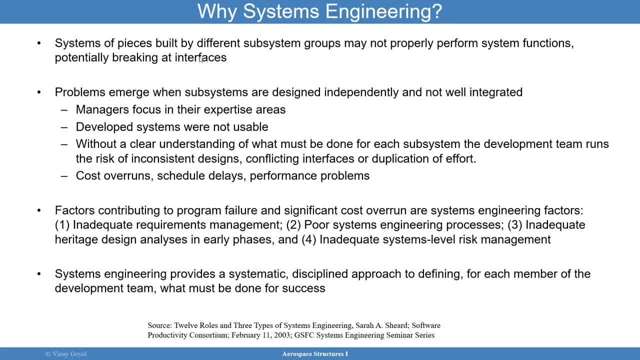 cost schedule delays and also cost performance problems, and So factors contributing to program failure and significant cost overruns are systems engineering factors, Inadequate requirements that are not flowed down properly, poor systems engineering processes, Inadequate heritage design Analysis in early phases, and what I mean with heritage is that when you're designing a product, you may have an early version of that product. 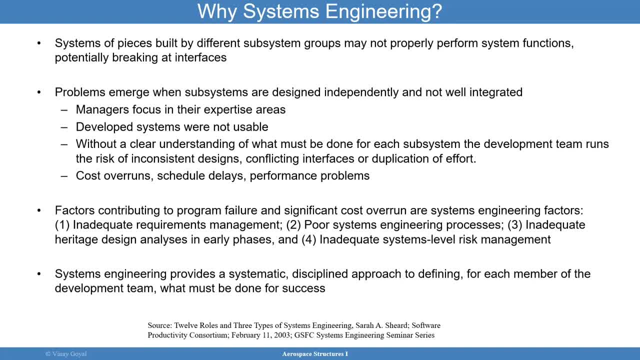 That has been successful. So Using those heritage design analysis practices and not using the property could be a problem. Inadequate system level risk management management meaning, Say I have a risk in a particular subsystem and that risk can affect other systems. Not having a system level risk. 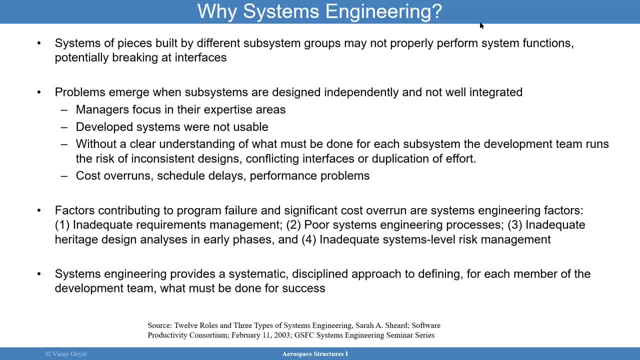 That can be visually seen by other groups Could be a problem as well. so the systems engineering needs to provide a systematic discipline approach to defining the problem for each member of the team and what must be done for the success, and So I encourage you to look at this source here at the bottom. 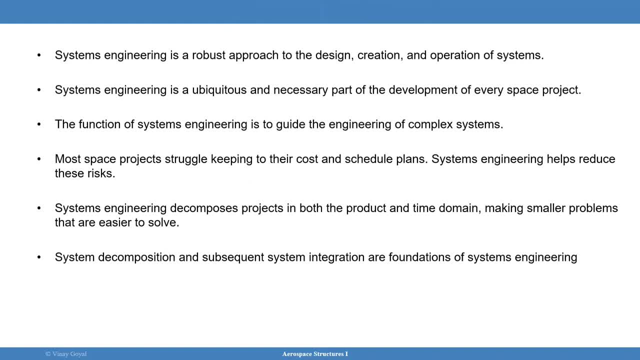 So it is also a necessary part of every space project: the function of systems engineering to guide the engineering of complex systems. Most space projects struggle keeping their costs and schedule plans down, and systems engineering helps you reduce those risks. It's just the complexity of space systems that makes this so difficult to attain. You can look 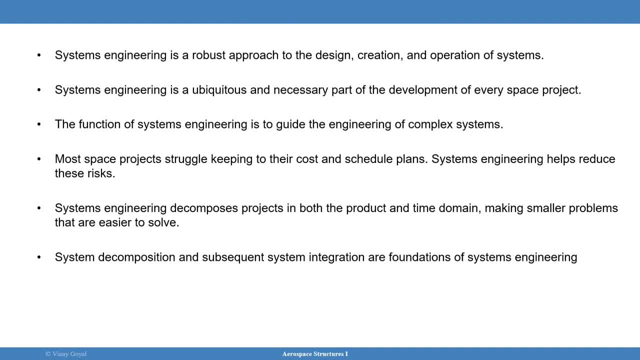 at almost every space system, and the James Webb telescope has, for example, been delayed over and over and over. Systems engineering decomposes projects in both the product and time domain and then breaks up the problem into smaller pieces that are easier to solve, And so this is the 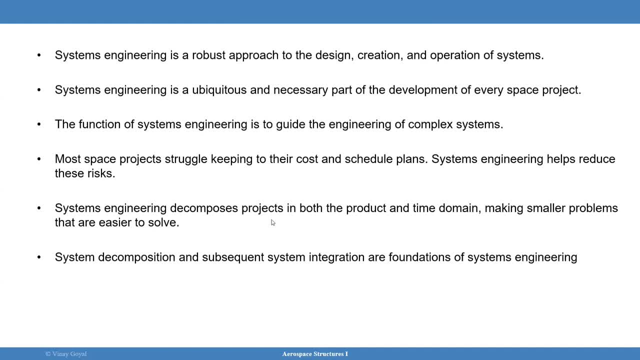 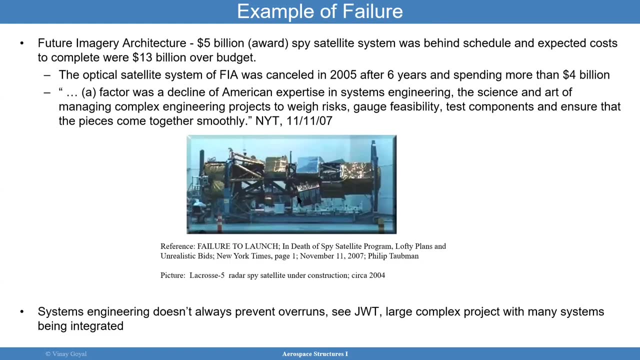 foundation of systems engineering is that building block approach- they'll be covering later on- but breaking up the problem to small pieces so we can then attack the problem in a in a way that's doable. Here's an example of five billion dollars by satellite does behind schedule and expected cost. 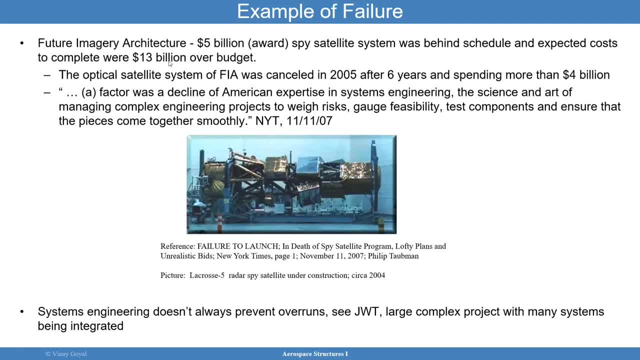 went over 13 billion over budget. The optical system of this future imagery architecture was canceled in 2005 after six years and spending over more than four billion dollars. And why is that? Why is that? There was a failure in how systems engineering was applied. There was there was a decline in the expertise. 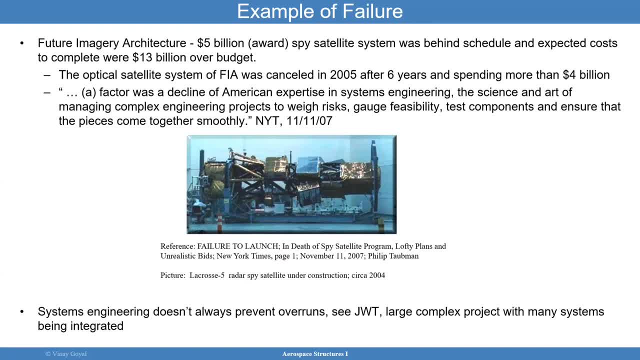 in the arena, The science and art of managing complex engineering projects- to weight risks, gauge feasibility, test components and ensure that pieces came together- was a miserable failure And you can look at the article there to look at that deeper. So systems engineering: 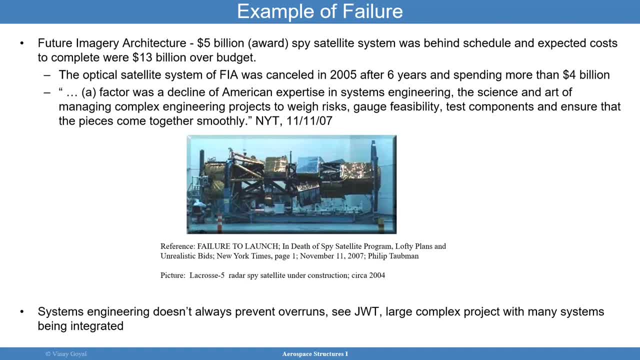 may not always prevent overruns. See JWT, the James Webb telescope. It's a large, complex project with many systems integrated. So a systems engineering may not always prevent overruns. but bad systems engineering can be equally bad as not having one. So it's important to understand. 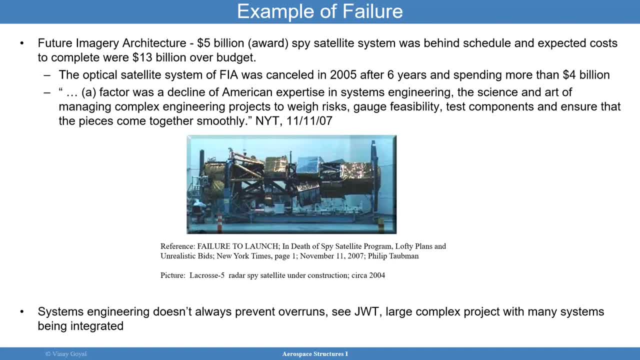 that the whole point of systems engineering is to stay on schedule, be efficient and bring teams to get it working very closely together in a well-oiled machine. If I don't have that, then you may not be even profitable down the road. 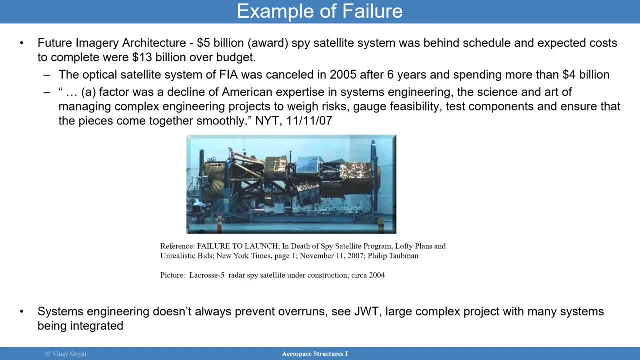 And you may not be able to even meet program requirements, and the final product will be a failure. So it is important to understand that nobody is asking a systems engineer to foresee all possible issues that could happen during the life of the program that may not allow you to fly when you're. 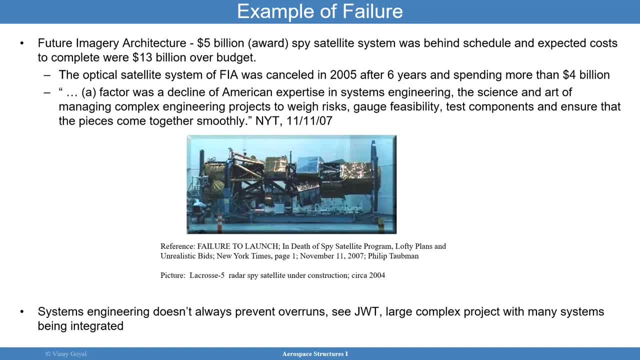 done, But it's important that the systems engineering team that's put in place works very hard with the team in place to make sure that we have a well-oiled machine. Then any risks that are coming up are getting mitigated and worked on to ensure that we have a product that is going to be. 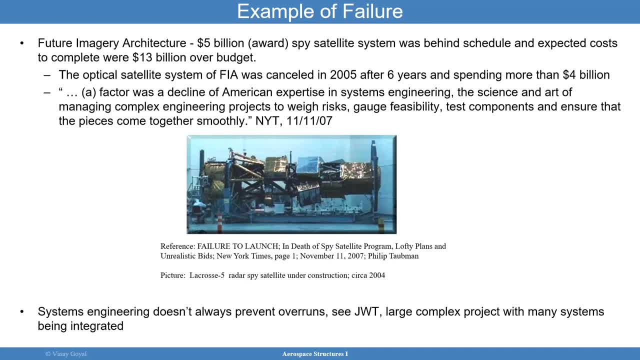 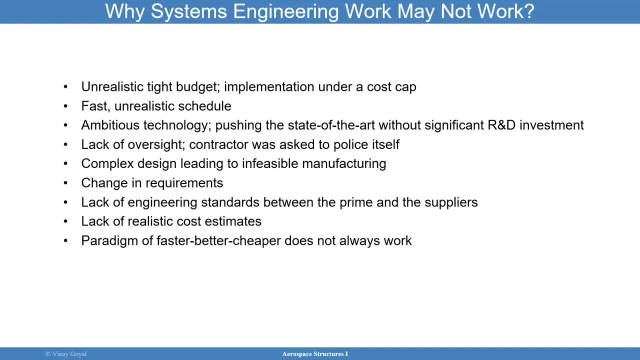 successful. Now we don't have a product that is more likely to succeed. Nobody can guarantee that product will succeed, but what you want to do is put the pieces together to increase the likelihood of success. So why does systems engineering work? It may not work. You have 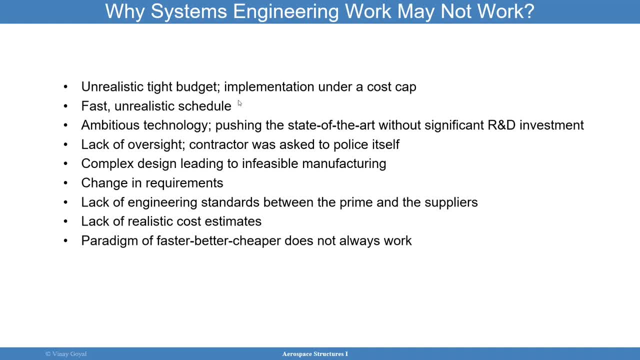 unrealistic budgets, you have unrealistic schedules, you have a technology that is not very, a technology that is so ambitious that you're pushing the state of the art with a significant rd investment, and so you may not have the technology readiness level that's required and that may not have been completely, completely vetted. and what is a technology readiness level? 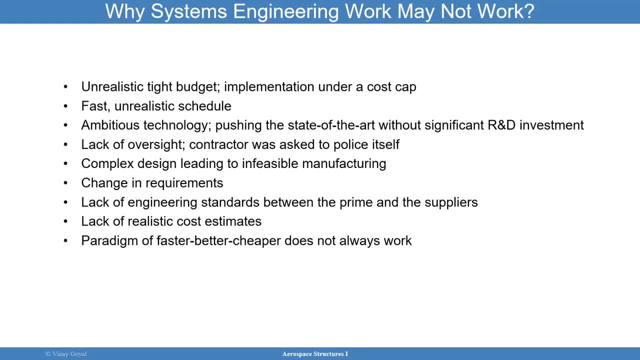 is a method for estimating the maturity of technologies during the program, and this is really developed by nasa, and the idea here is to really understand how, how, how how competent this design is going to really be and how mature it is to where it needs to go. so trl1, for example. 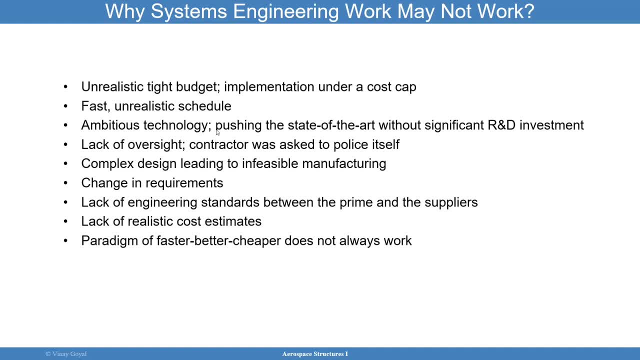 is basic technology research and if i say okay, in two months i'm proposing a, a constant design that has never been investigated before. if it's a trl1- basic technology technology research- you don't even know if this is going to work out. so any schedule or budget. 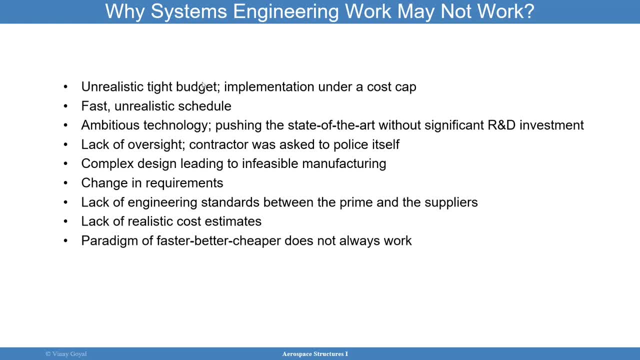 amounts they put in on paper may not be even prove, you know, may not be able to achieve those budgets and schedules. then you have trl2, which is research to prove feasibility, and that's also trl3. then you can move trl4, which is technology demonstration. 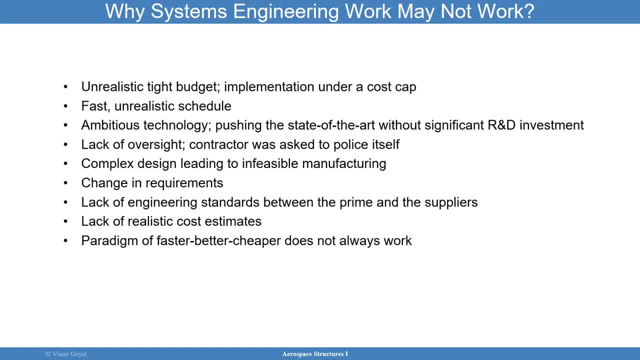 and then you can go to more mature systems, such as system test launch and operations, and so it's really important to understand how ambitious you are compared to what your schedule looks like and your budget impacts are. there's nobody's telling you not to be ambitious- you can be. 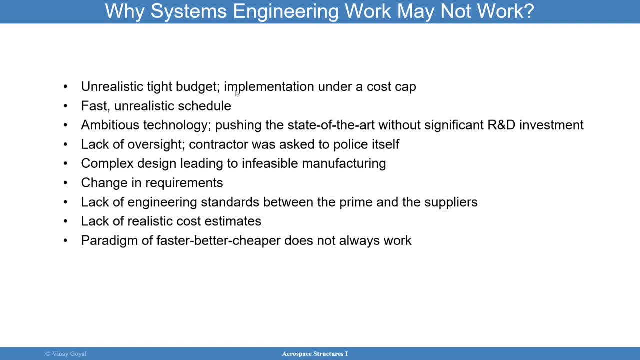 ambitious with the technology but then make sure there's really a lot of work to be done to make sure there's room to develop the technology. with irnd research and development lack of oversight, so perhaps the faa or the nasa or whatever organization may not be overseeing what's. 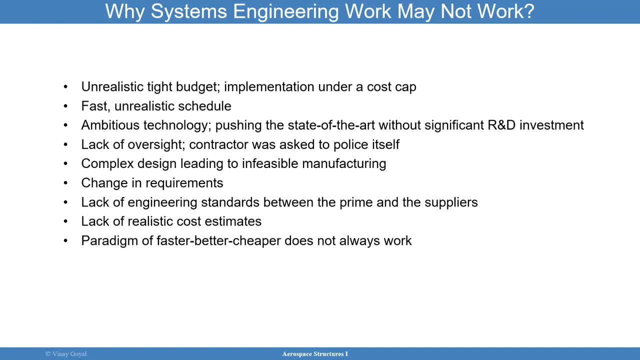 going on. so, when the product are close to completion, we have an issue where, uh, the product is not meeting the regulations that need to be put in place for safety. up, safe in the design, complex designs leading to infeasible manufacturing. you could have a designer that. 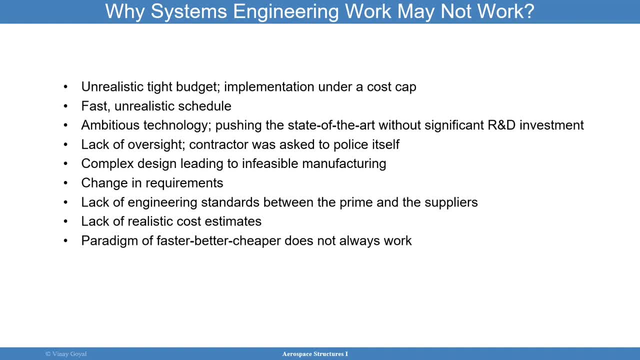 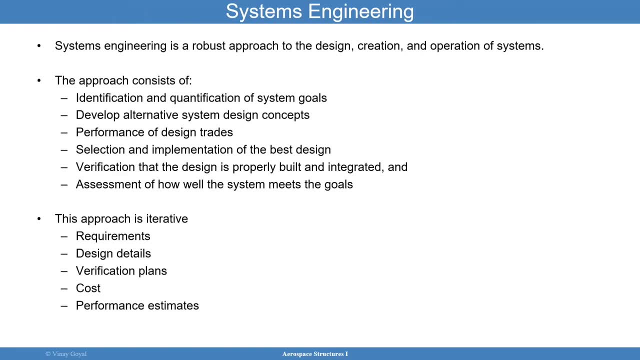 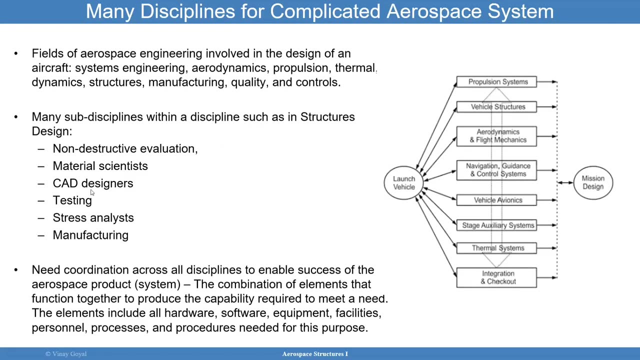 all the designer has done is cat modeling in his brain, in his head. the question is: can i even make the design? and that brings me back to this point i was making, where we want to make sure the cat designers are working closely with manufacturing team. they're closely with the 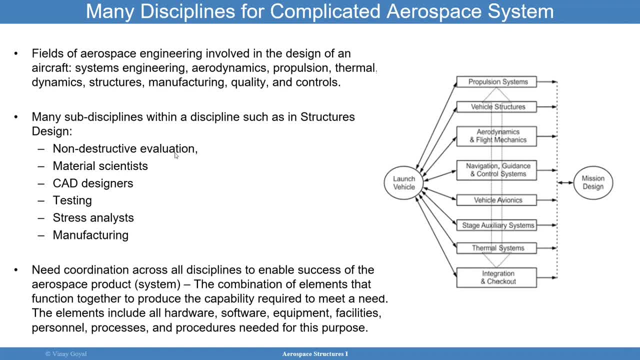 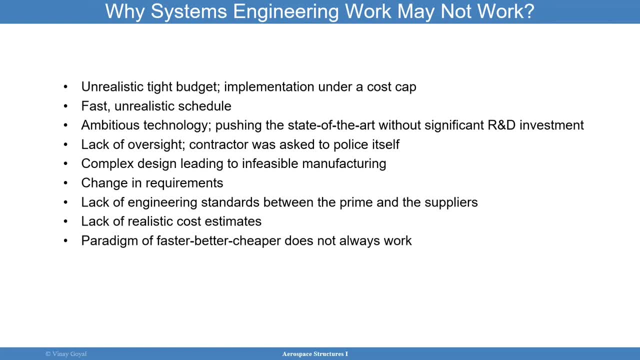 materials team and testing and analysis and non-destructive evaluation to make sure that whatever designs are being proposed can be achievable. and the designers have to be respectful to the stress engineers and the stress engineers have to be respectful to the material scientists. everybody has to respect each other and sometimes these design organizations. that's not happening. 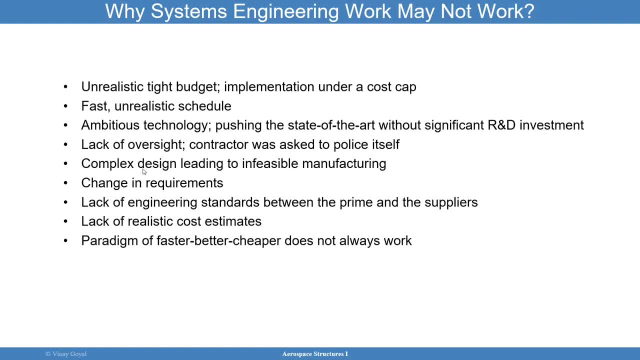 and when that doesn't happen, and when the team is working, uh, not very oiled together, then you're going to have these issues. what happens if you're working to a set of requirements and the requirements are changing on you? for example, i told you design this structure to 100. 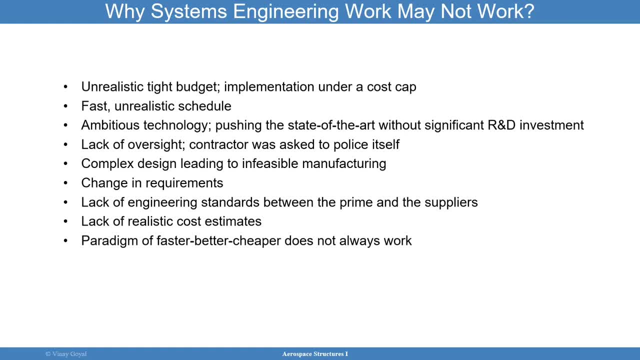 degrees fahrenheit. but later i told you: hey, you know, sorry, we cannot go above 90 degrees f. then that's a changing requirements that could happen late in the game. where could, which could cause the whole thing to slip? so that's why requirements, functional requirements and governing requirements that 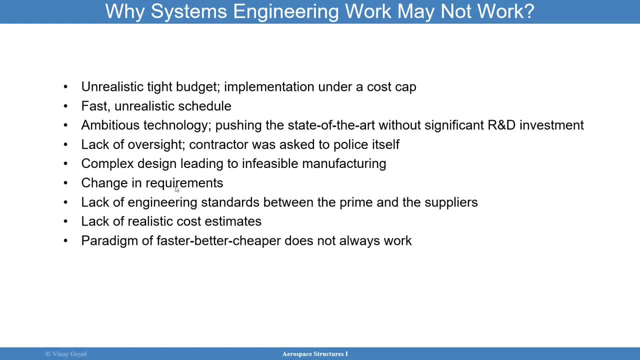 regulate the structure need to be communicated early in the process so it can be prepared for what's coming. the lack of engineering standards between the contractors and their suppliers. that can also cause then the suppliers to create products for the prime contractor that may not meet their own requirements or the requirements for the for the governing agency, like. 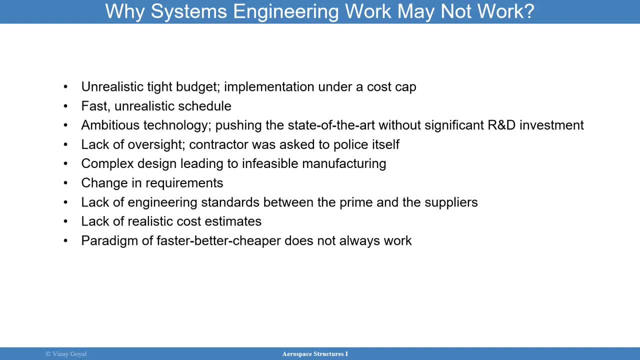 fa or nasa or whatever we're looking at here. there's also the lack of realistic cost estimates, and this idea of the faster, better and cheaper is always better not necessarily faster, better and cheaper could cause: 잘상 정작 86 оно, which means higher rates of fanдаlorization. but there are real vragenco cost estimates. there is no lack of value. findings: Yang Zhenным. 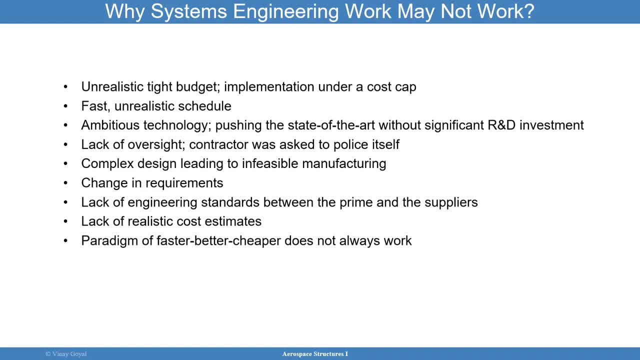 people to cut corners and not do the right things, such as getting material properties- we'll talk about that later. you know, getting the material properties that you need for your design so they can then design it in the first place instead of making them up, you know. so cutting those corners can also be an 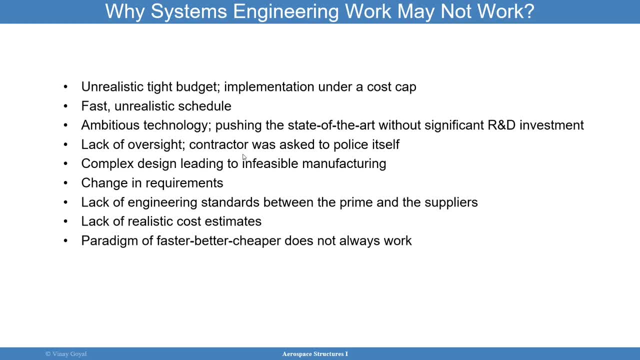 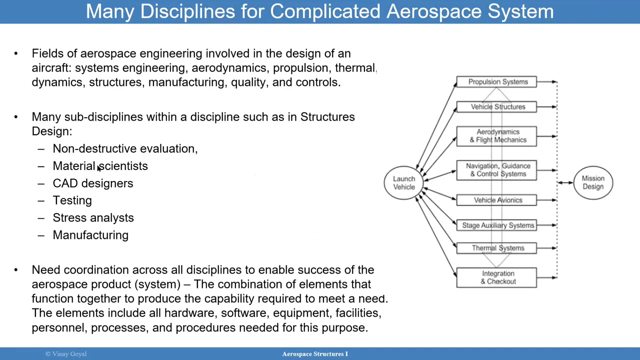 issue. so you may have assistance engineering in place, but you may not have the best systems engineering in place. that could then cause an issue in the designs. you know you can design the best structure in the world, but can you manufacture it? can you are using the right materials? can you even test it if 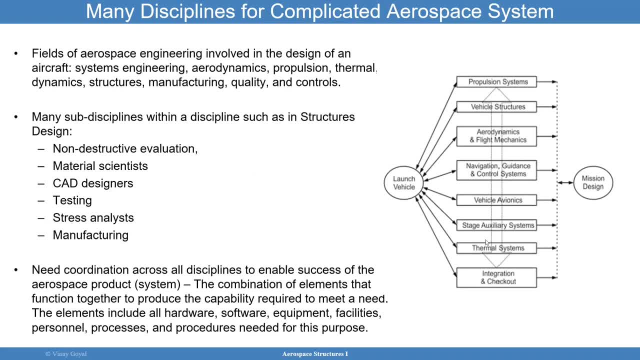 what if you design it and it doesn't meet any of these other requirements from propulsion, thermal and anybody else? so I think the point I'm trying to make here is that if you design it and you don't have the best systems engineering in place, but you have the best systems engineering in place, but you 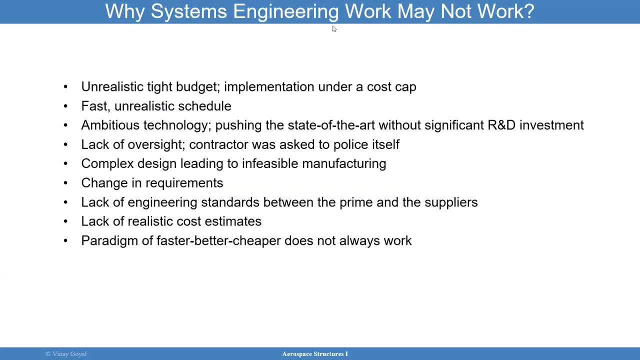 design it and you don't have the best systems engineering in place. but you trying to make is that you ought to work with a team of engineers. you ought to work with a team of engineers, otherwise we're gonna have some serious issues on their consideration. that's a that's a great point and great question. so what it? 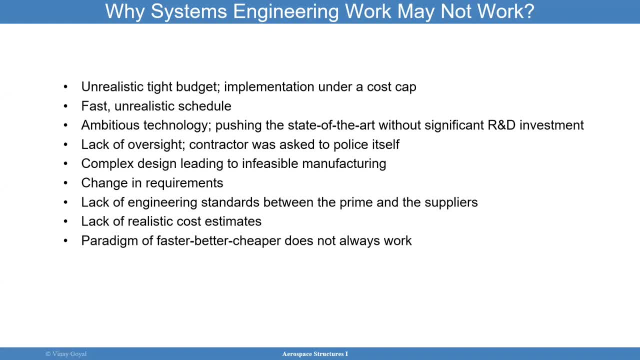 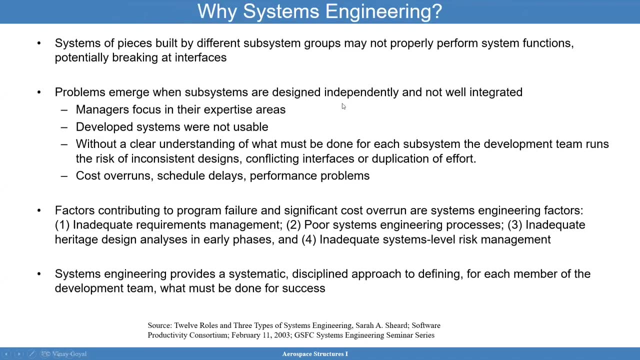 takes to be assistance. a good systems engineering is to actually take training in the area. number one, so you want the courses in the area. but number two, a good systems engineer is one that has experienced doing it, so it has gone through various areas of expertise. the best system engineerants I have seen are ones that 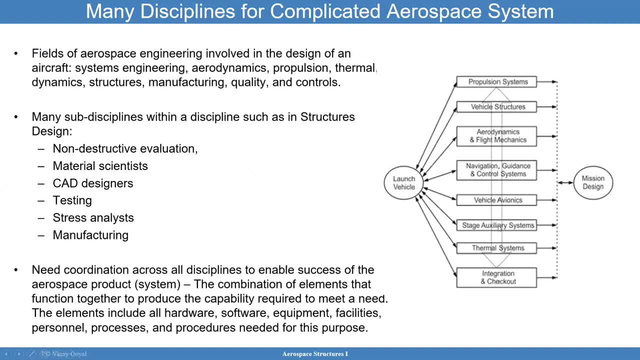 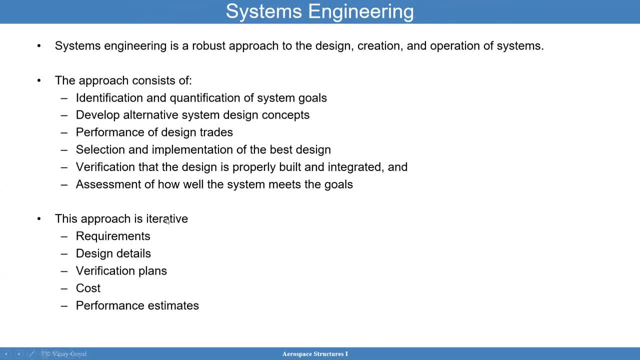 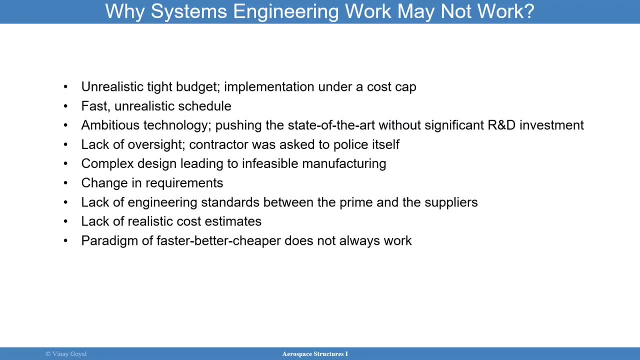 have actually worked all the systems and then when they go back to systems engineering, they have all the knowledge from different disciplines. so they know the roadblocks to. they know the roadblocks to to overcome. so in other words, a good systems engineer is one that that knows everything from higher level to. 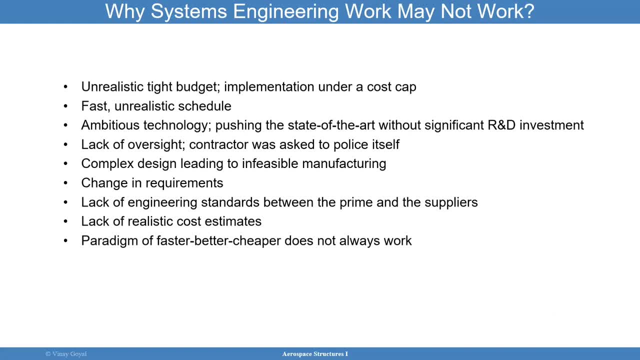 the many different buildings in the neighborhood. why is a good system? engineer is one that has experience doing it. so it has gone through various areas of expertise- the business engineering I've seen are ones that I have- that has experience in multiple facets of the program and each discipline. so when they're in 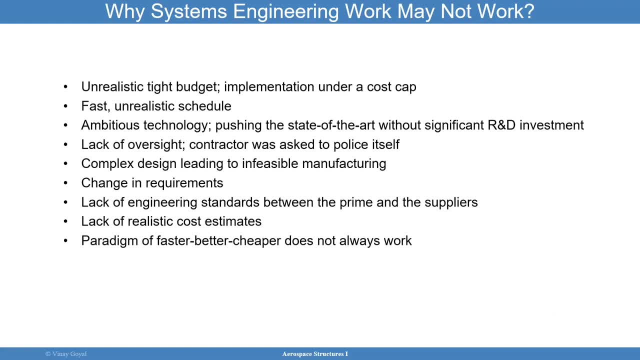 that position. they know what roadblocks will be encountered. it makes sense. you need to be a generalist, you need to know how to do a little bit of everything, and even schooling may not give you everything you need for that. you may want to um get some experience when you work at a particular 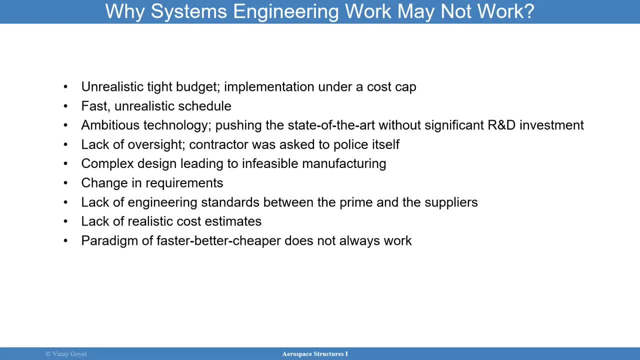 company and you tell management: hey, i want to work on systems engineering, help me, rotate around, right, help me if you don't be good systems engineering when you are hired. you want to get training, but you also want to get good at everything. you also want to get uh experience. 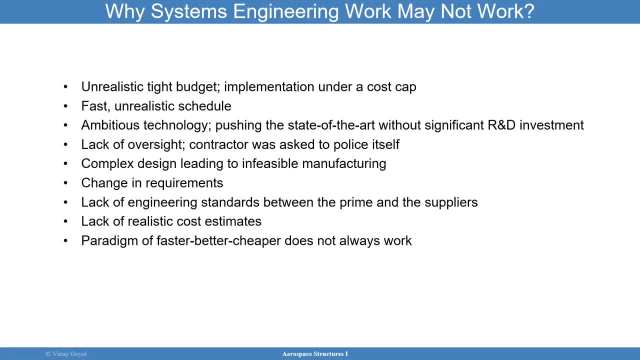 in all the different areas that you can so that when you're working in systems engineering you can be a generalist and you can. you know you can identify those roadblocks when they show up and you can help teams work well together, and that's hard to. 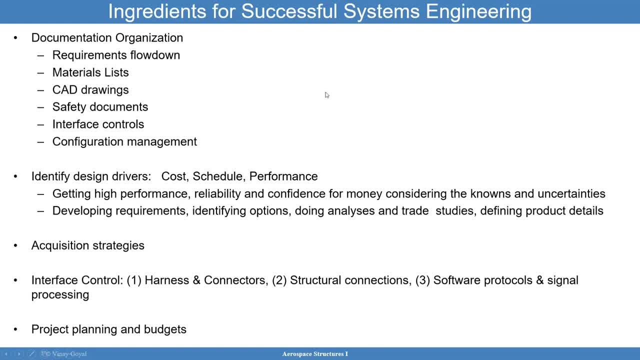 do when you don't understand what each team is really doing? the key ingredients, uh for successful systems, engineering, documentation uh require, you know, bringing the requirements down to the lowest level, so flowing down those requirements, functional requirements and regulatory requirements- all the way down- um, all the materials are going to be used- and making sure everybody understands what the 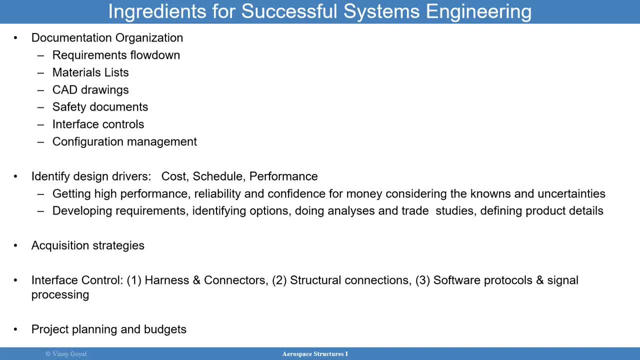 materials are being talked about the CAD drawings. having a very good configuration, management of these CAD drawings, safety documents, interface controls, the interface uh controls between components. you also want to identify design drivers, the cost schedule and performance to get high performance, reliability and confidence. uh, it is important to really consider the unknown. 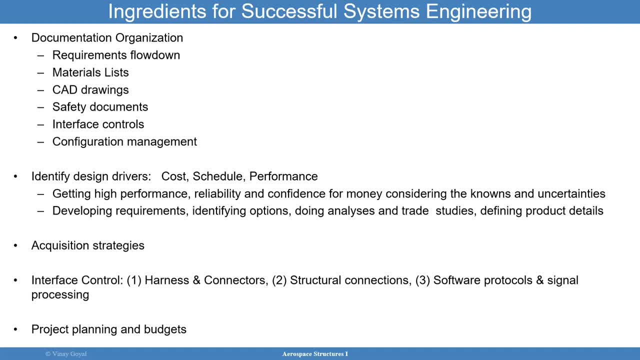 the knowns and the uncertainties, developing requirements, identifying options, doing analysis and trade studies and defining product details. you also need to understand the acquisition strategies and for the interface controls here that we're talking about. we're talking about what are the features, and you all trust the system's functional capabilities and we also want to know what are the. 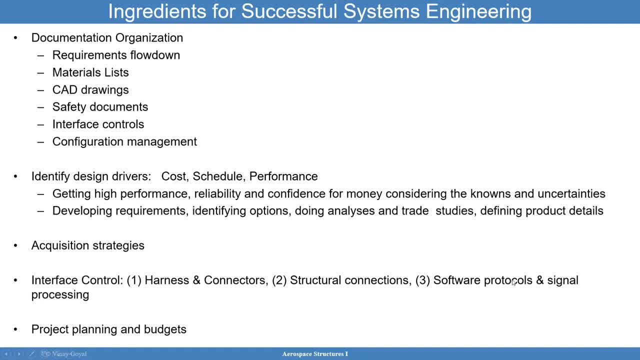 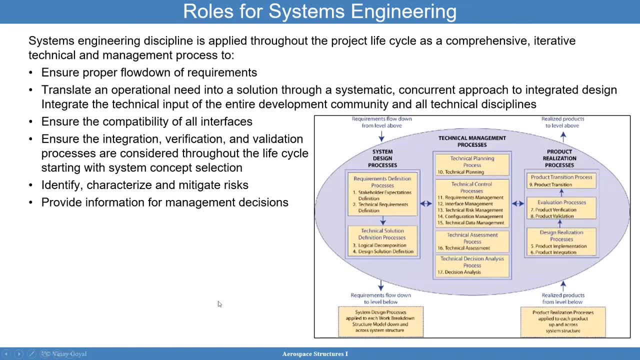 features, and we can do that through this small friendly conversation, and then, ultimately, we're going to look at a variety of different, you know, systems engineering, automation for the project management, and so these are the main components of the system engineering organization to develop the project set as a comprehensive process, to install a project in a very user-friendly. 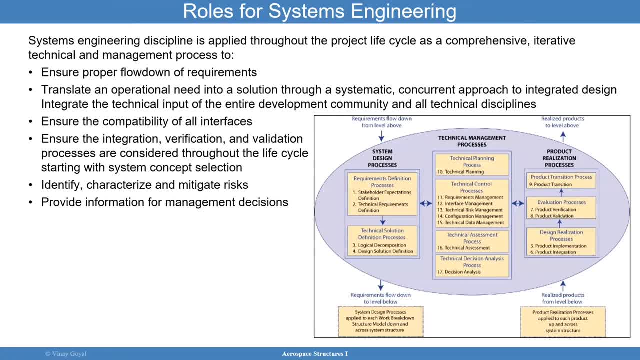 way making sure that the systems engineering, engineering operations are a commander to the project management and human beings in general. so, unless you're a user or a part of a team or an office, you are going to need to determine the overall engineering infrastructure and to prepare to work. 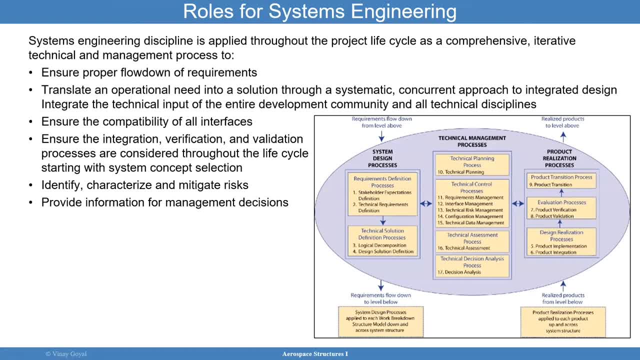 out the project as a whole and ultimately you're going to have to be able to build the systems engineering, Translate an operational need into a solution through a systematic, concurrent approach to integrated design. So you want to make sure that the team is working well together. 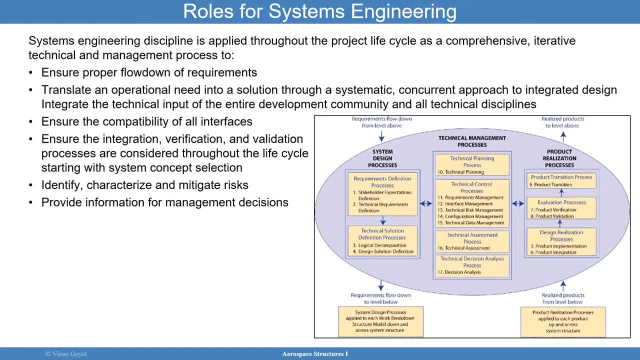 That's really what concurrent is really saying here is: you're working towards an end goal together. You want to integrate the technical input of the entire discipline team, the entire community and all technical disciplines together. There needs to be a lot of communication between disciplines, ensuring that all compatibility of all interfaces, that all interfaces are compatible. 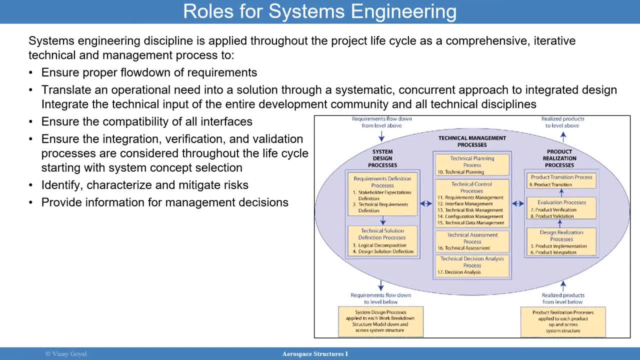 You want to ensure that we consider the integration, verification and validation of the processes through a life cycle starting from the concept design. We also want to identify, characterize and mitigate risks And provide information for management decisions, And so here I have three legs. at top level, 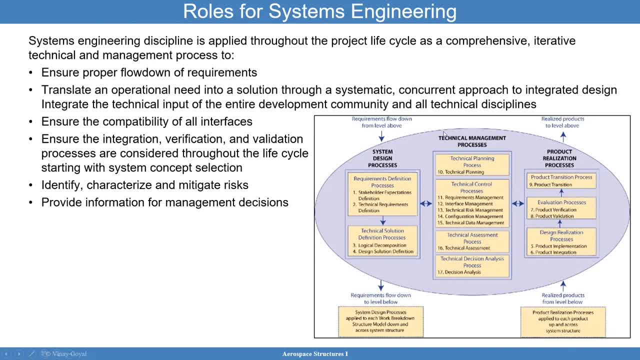 The first one is systems design processes, The second one is technical management processes And the third one is product realization processes. In the systems design processes, what we're really looking at. there are four pillars in the systems design process And they're used to define and to baseline expectations, generate and baseline technical requirements and then take those requirements and decompose them into logical models and provide them to the teams and convert them to technical requirements that the team can use to satisfy those baseline expectations. 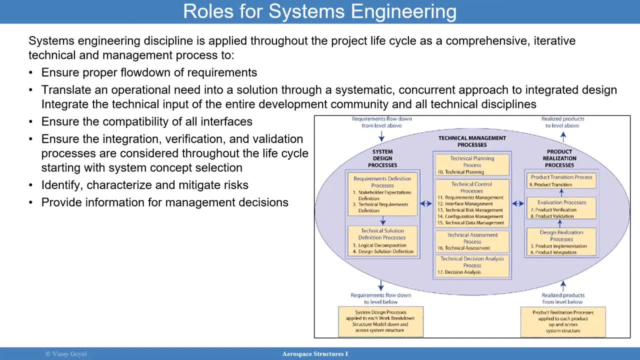 That's the bottom line, Okay, And Without that we can't have a good systems engineering. If I don't have a good flow down of requirements, I don't have a good technical management process, I don't have a good way of talking about product realization processes, then we're going to have an issue. 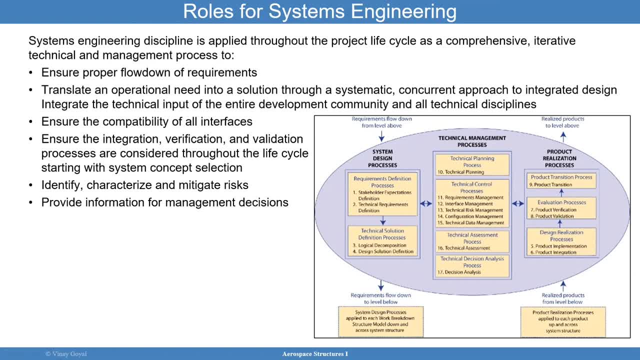 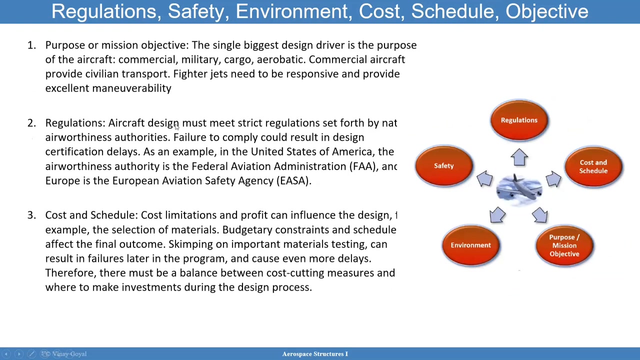 To the point that I cannot realize a product in the first place, And they are established AS AS 91 requirements for systems engineering. that that can help provide some structure To these systems engineering processes, to the 17 Systems engineering processes. Okay So regulation, safety, environments, cost schedule objective. we need to really understand. 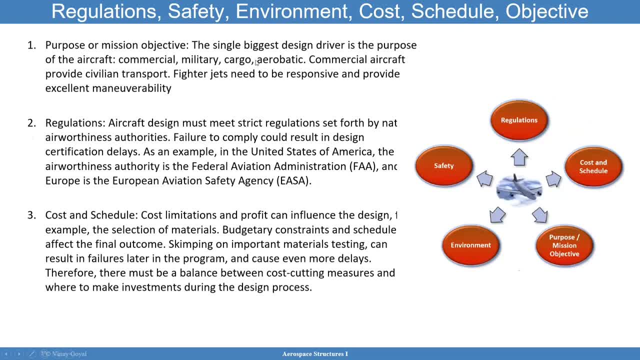 What is the objective? Am I developing an aircraft for commercial applications, military cargo? who are the key players, who are the stakeholders For the particular objective I have in mind? Is this aircraft going to just go from here to San Diego, or is it going to go from here to Africa? 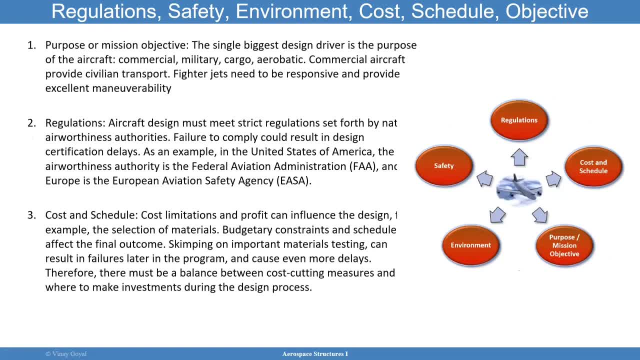 Or another country. If he's a fighter jet, needs to be extremely responsive, But if it's a fighter jet For military applications, direct, the regulation for that may be different than if it's a commercial application. You also need to understand that regulations in the first place and need to understand what are the agencies involved. For example, the Federal Aviation Administration is airworthiness authority here in America, United States of America. 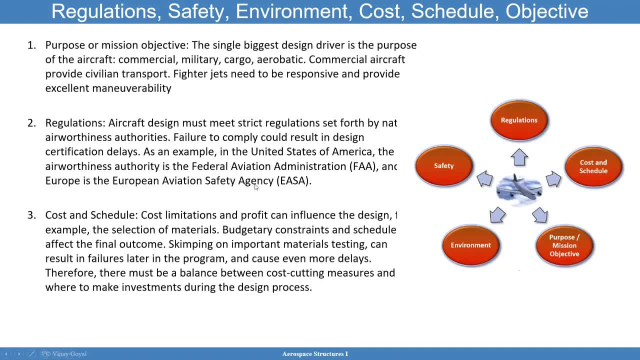 Well, the European one is a European Aviation Safety Agency. So there's various organizations. or, if I have a launch vehicle design and launch vehicle design is for NASA, Well, it needs to meet some NASA requirements and so forth. Cost and schedule: Again, we we touched on that. But the point I want to make here- that comes up a lot And I will be covering more in this course- is skimping on important materials: testing. 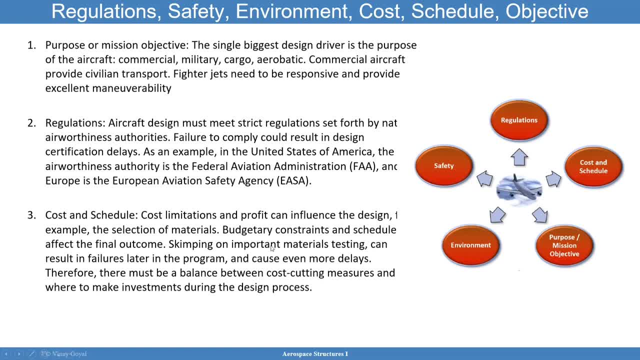 And not paying attention to that, because If you do not put attention into materials testing, it can come to bite you later in the program where that testing could have been valuable and could have Basically expose issues early in the program rather than when it's too late. Maybe the failure happens during the testing of the full scale article and airplane and then later on It's just too late to build to to accommodate. 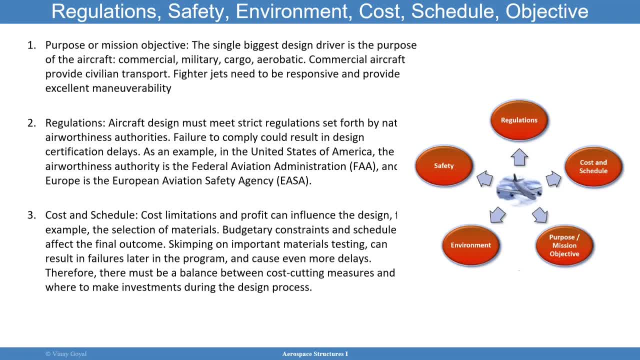 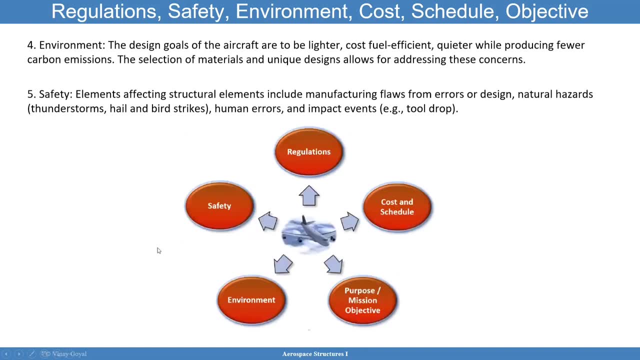 Any redesign. And if you were to redesign may as well just cancel the program. So so it's very important to understand this and the consequences of of not balancing costs and schedule with technical considerations. We also have the environments: the launch environments, the aircraft environments. We also have to make sure that the design goals are clear: lighter, cost, fuel efficient, quieter. 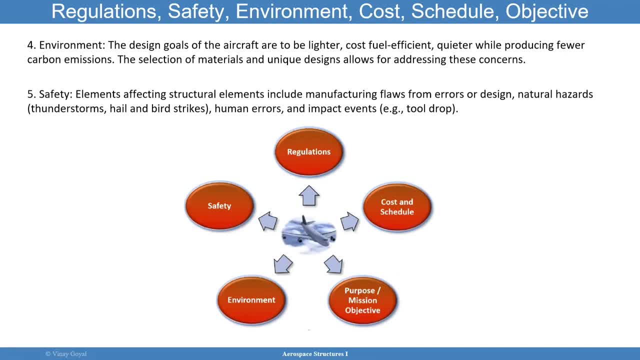 And while also producing for your carbon emissions. So the selection of the materials and the unique designs will allow you for addressing this concern. Safety is another one, and it affects elements such as manufacturing flaws, errors, human errors, natural hazards, Impact events. These are things that need to be considered in the aircraft design. 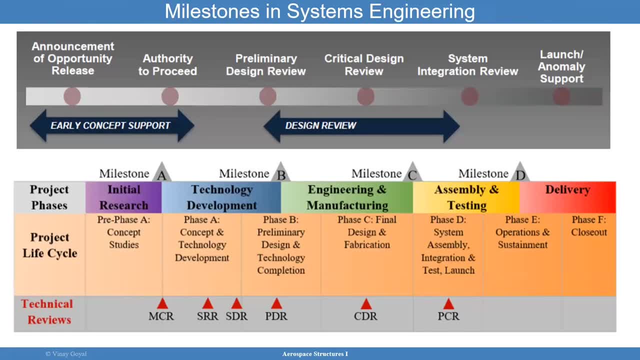 So let's talk about the design goals now. So milestones become the quarter quarter bit of importance, The play quarter bit of importance in systems engineering. It basically allows you to check the system health as a function of time from early opportunity to release Early concept design. 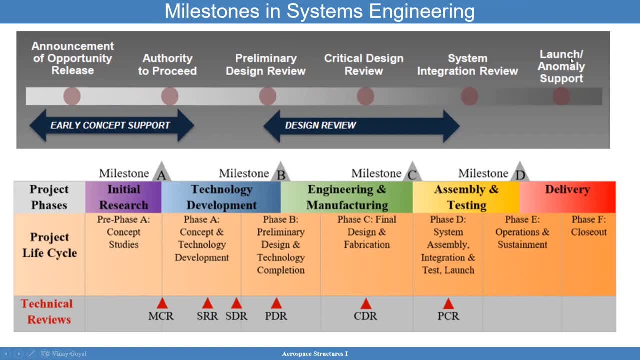 And all the way down to the launch, Launch event or aircraft deployment, or aircraft deployments to the different airliners. so these intermediate steps become a key role in determining how the project is going. you have several cycles that could be iterative at times. you have the initial research, the concept studies, 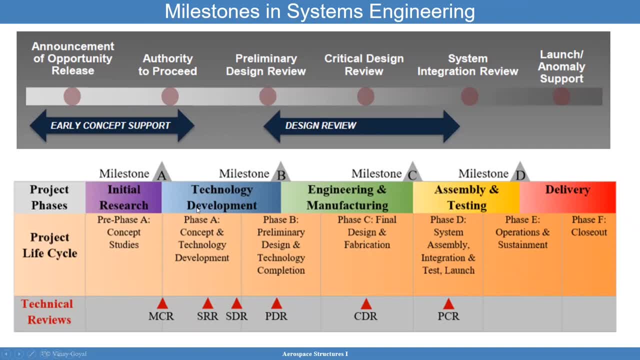 you have the concept and technology development and some of these could have a lower maturity readiness level in terms of technology and then you can now start entering once you have the concept design in place and you've gone through some mission concept reviews, and i'll be covering some of these: mcrs, srs, sdr, pdr, cdr, pcr. i'll be covering that in the next. 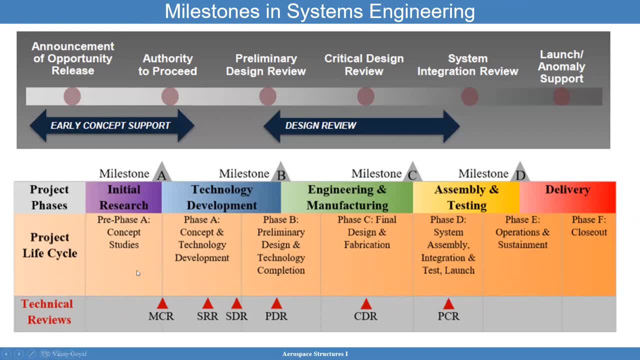 slide. but once you have the mission concept review- and i'll cover that in the next slide- uh, and you've maturing the, the technology and and the project cycle is maturing, right, you, you're, you're maturing that design. you can then start fabricating and designing and then you can assemble, test and then you'll be able. 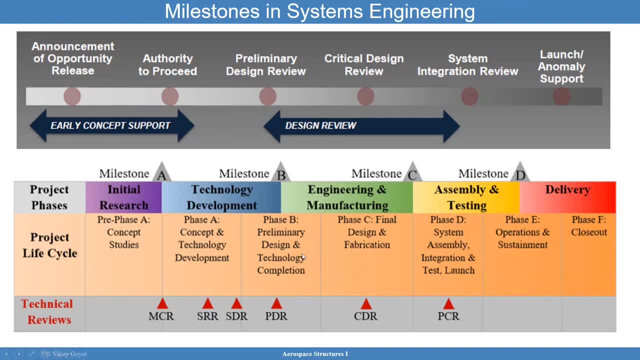 to then either have to redo some aspects of this if there's a failure, but generally you're coming here down the road by going to an operational phase where you're going to have to start tracking issues with the hardware. they're basically- most of them are- human errors or non-conformances from not being able to build everything as you. 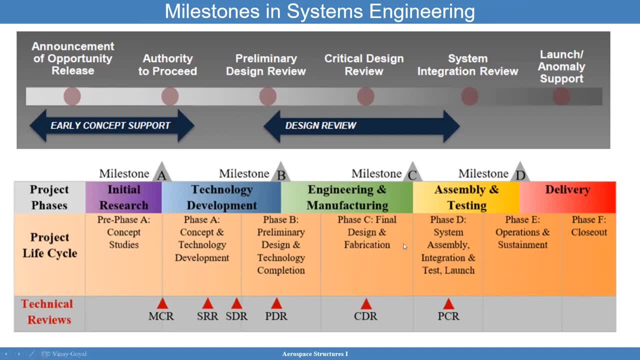 had expected. there's no single way. no way they can put a drawing out of a design and expect that everything's going to be perfect. that's not going to happen, and so you're going to have to address that during the delivery phase and you're going to have to say: well, 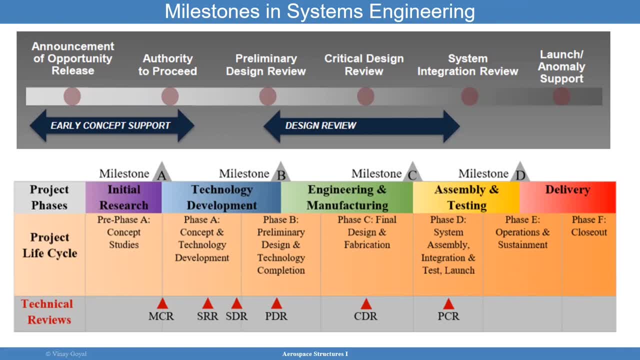 the ticks. you know the. the aircraft thickness was supposed to be 0.12 inches, but when i made it and i'm testing, it's not quite 0.12 inches, it's more like 0.08 inches. well, you may have to revisit the. 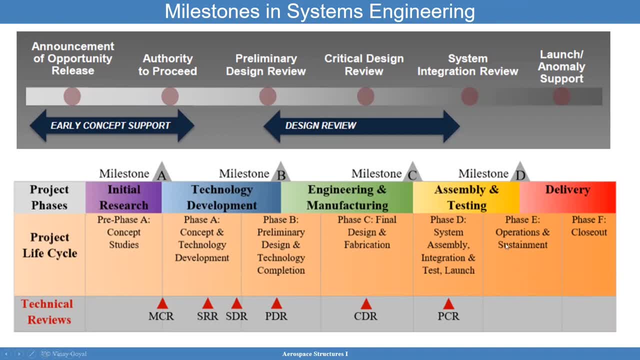 test, or you may have to then assess whether you know the, the, the during the delivery phase, whether the customer will be okay with that delivery, which you know. with that big of a difference for the skin thickness of the aircraft, i'd rather go back and make sure i have everything well designed and manufactured properly. so there. 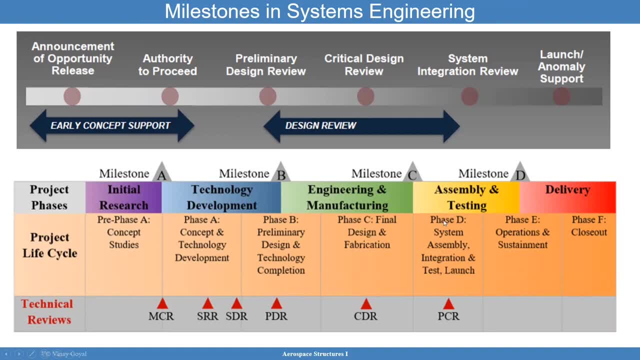 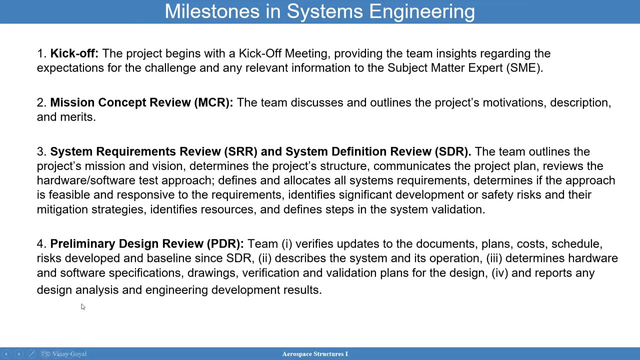 are technical reviews as you go through this life cycle process, and these technical reviews- mcr, sr, sdr, pdr, cdr and pcr- are the ones i want to talk about now. so you have the kickoff meeting here, typically, where the the team is provided some expectations about what the project 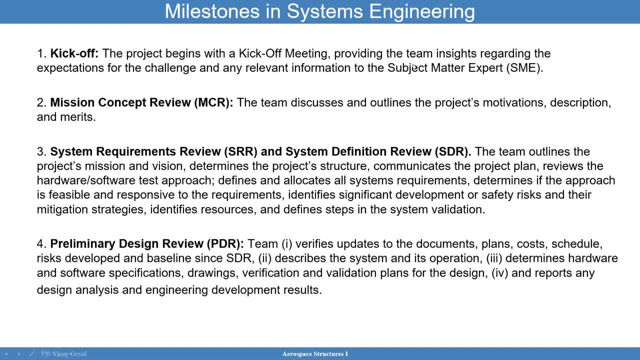 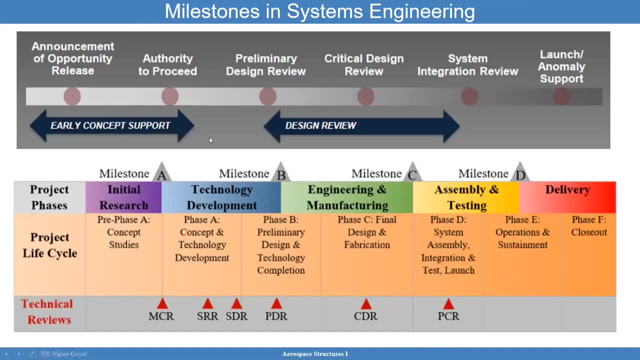 is about. you know you're gathering the subject matter expertise, you're trying to make sure you have the right expertise in the room, and then you have the mission concept review, where the team discusses and outlines the project motivations and descriptions and merits in. here is where you 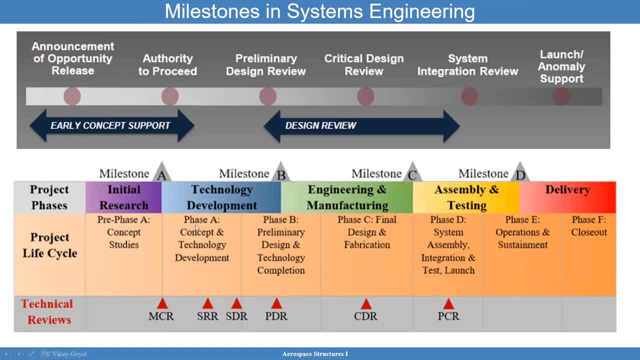 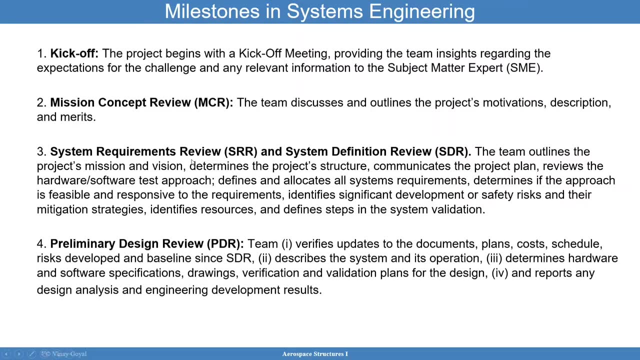 are start to talk. you're starting to talk about the concept review and you're starting to talk about the concept designs. and in the midst of this phase, here, phase a- you conduct a systems requirement review and a systems definition review, and here you outline the project's mission and vision. you. 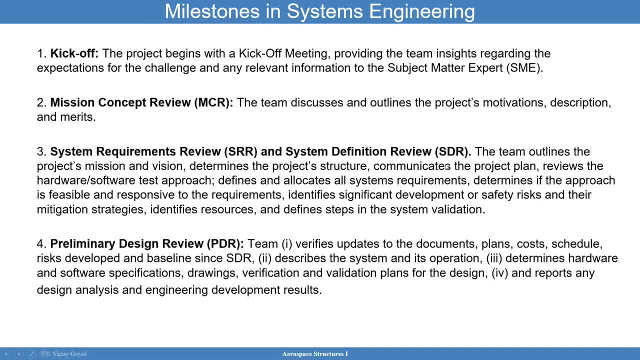 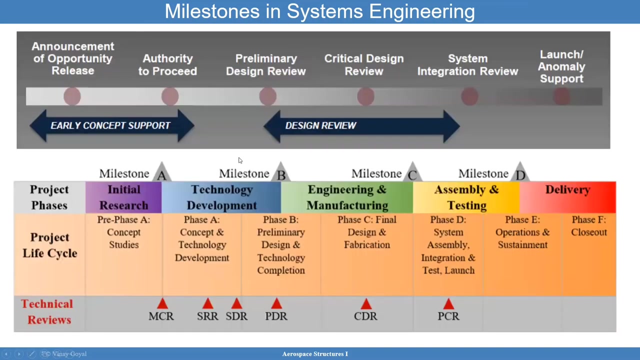 determine the project structure. you communicate the project plan, you review the hardware, the software, you define and allocate all systems requirements, you determine the approach that's going to be proposed is feasible and you're going to determine the project structure and you're going to think about the location, the ability, the facility, the framework, the and then you identify significant developments of, or safety risks and their mitigation strategies. you also identify resources and define steps in the systems validation. once you're gone through this process and your concept designs are likely to pass these functional requirements and these requirements that were defined through these. 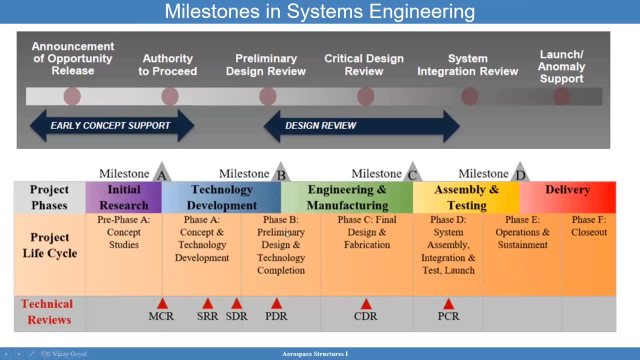 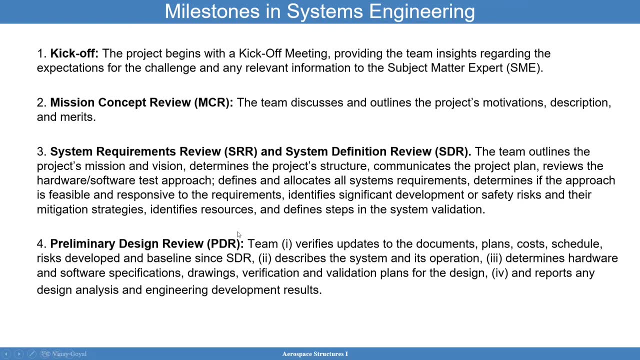 two reviews, then you are readier to go to the PDR And the PDR you're looking at a preliminary design review where the team is getting closer to. it hasn't finalized a design, but the conceptual design have been further matured. 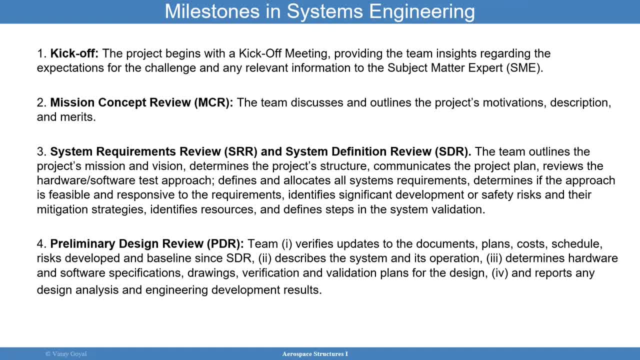 You have down selected the designs and you verify updates to the documents: plans, cost scale, risks- they're involved with the design you're proposing. Perhaps you have an additive manufacturing material that is not looking that great, So that's a red risk right there. 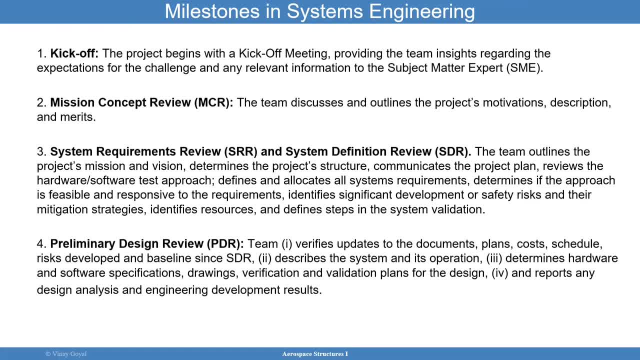 Perhaps you have a bold design, a joint design that is looking good. You can call that a green risk. It's not a risk at all. You wanna describe the systems and its operations. You wanna be able to determine the hardware and software specifications. 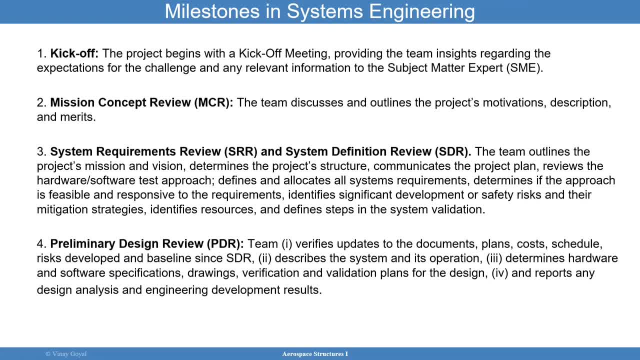 drawings, verifications and validation plans for the design and reports any design analysis and engineering development results. So here is an important milestone that can be used to determine the health of how the design is going. Then we have the critical design review. Here, if you pass a PDR, 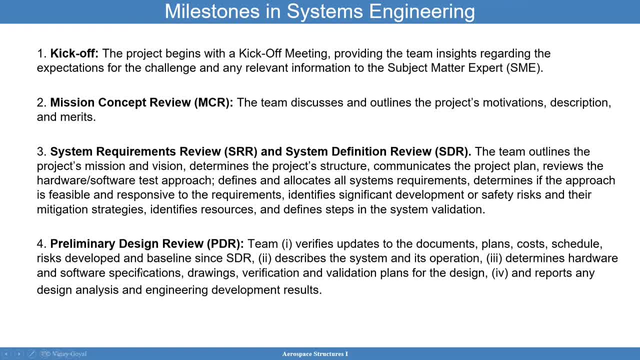 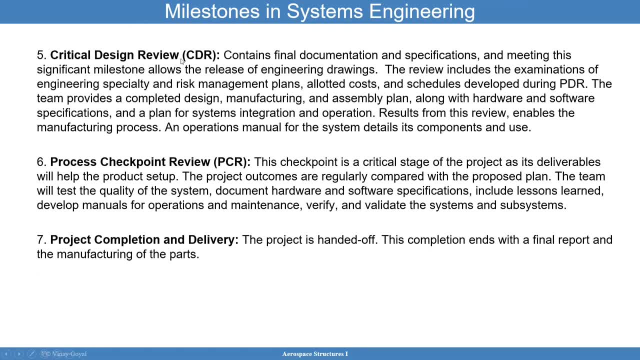 and you have addressed all the action items and you have addressed the risks that are coming up. you're closer now to start talking about what is going on with the structures that were designed. How close are we to getting it out? We have the final documentation, basically, at this point. 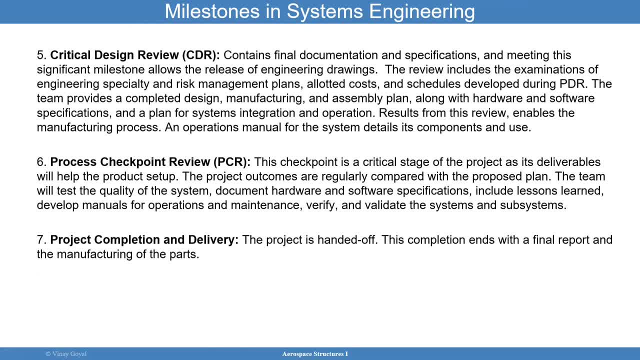 the margins of safety of the system have been defined and they have been discussed. The risks of the system have been mitigated for the most part. Some of the open items may be addressed later during testing, but this is a significant milestone that allows a release of engineering drawings. 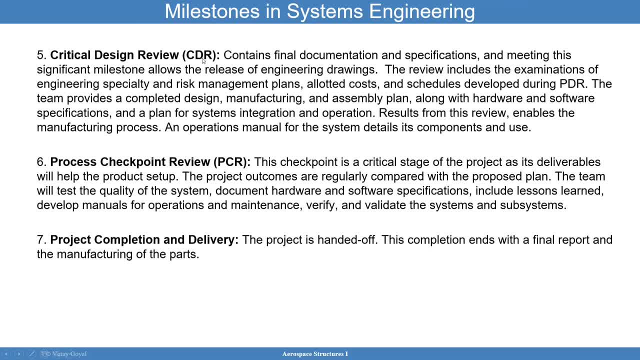 And so it's important that the designs are matured to the point there's high confidence They're likely to pass the testing That's going to be done later. Remember, at this point you may not have done testing, Although in some cases you may have had some testing done. 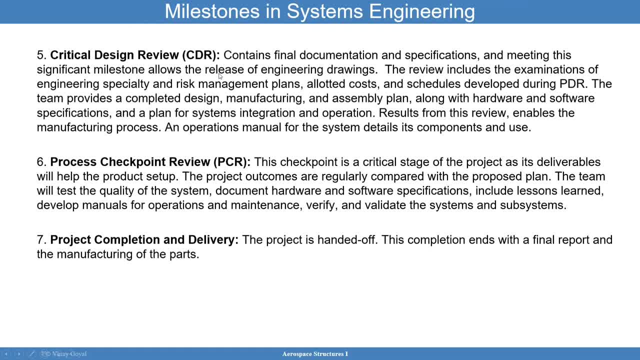 and some even heritage testing done. But at this point in time you have some confidence through analysis with sufficient factors of safety, that you are going to succeed. There are some great possibilities there that you'll succeed. The review will include examination of engineering specialty. 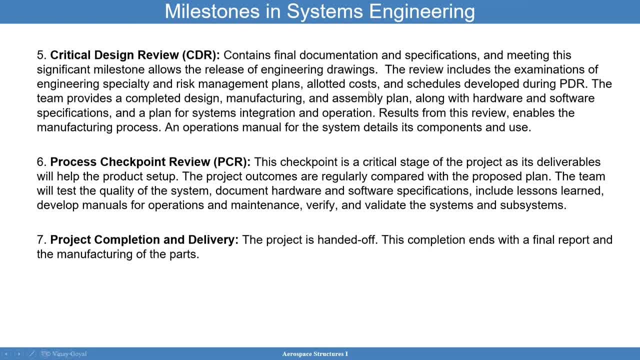 risk, managing plans, allotted costs and schedules, And the team is going to provide a complete design manufacturing assembly plans. They're going to tell you how everything gets transported, What kind of testing is planned. You may you know you gonna review this. 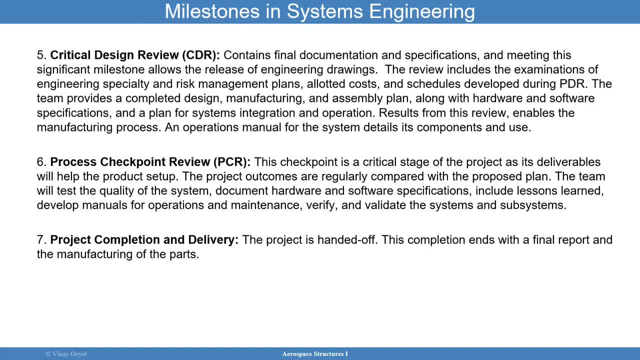 and make sure that you can actually even manufacture it. So the CDR is a major part of this, but it's also going to be a major part of the engineering process: major review in all systems. then you have the process checkpoint review. it's 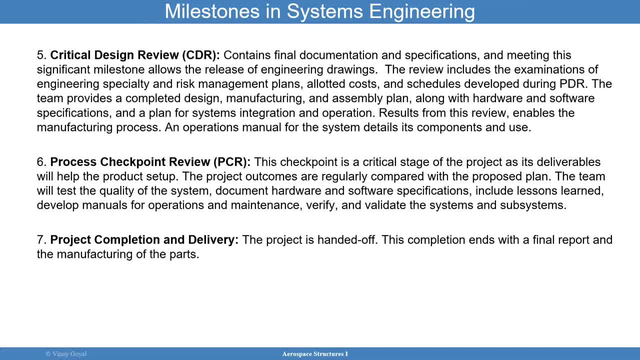 a checkpoint to make sure that we are on track for delivering the product and that the team will test the quality of the system and include all the lessons learned. you also, at this point, are developing operational manuals and maintenance manuals and verify and validate the systems and subsystems. 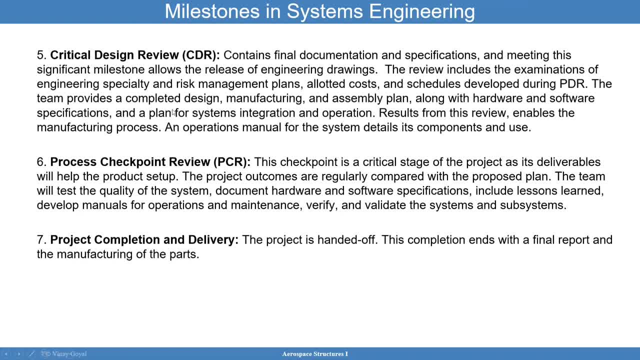 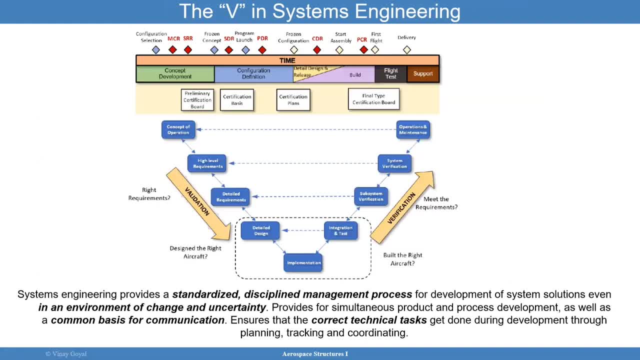 because if there's an issue and you have to redesign, you may have to go back a little bit in this lifecycle process. systems engineering, like I said, provides a standardized approach. here is what we call the V, and this V is superimposes, the major milestone mission. 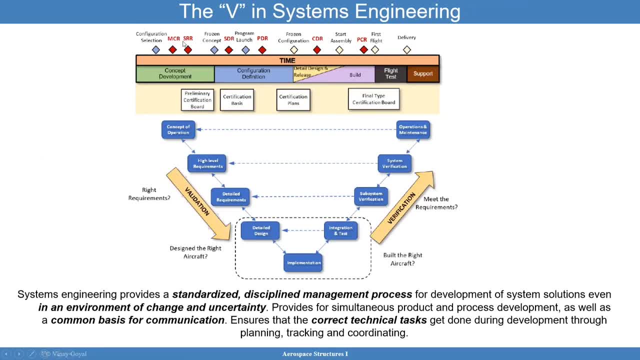 and basically you have the mission concept review, which is MCR, then you have the systems requirements review, which is SRR, and so forth. here we're outlining that superimposed with the V, the systems engineering V, validation and verification, the concept of operation, the high level requirements, the detail. 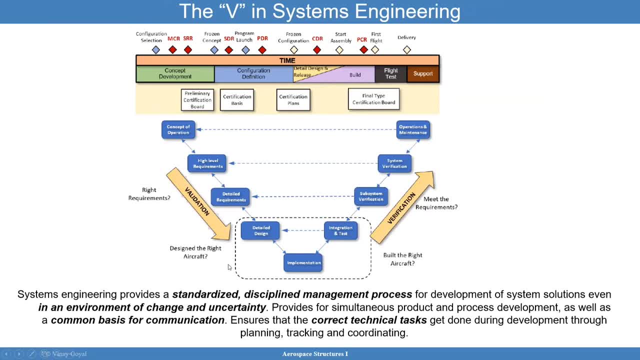 requirements, the detail design. so have we designed the right aircraft? are the requirements right? that's what you're asking here. and, as a move on to the later part of the V, I'm looking at implementation now. I'm looking at integration and test. I'm looking at subsystem verification. I'm looking at 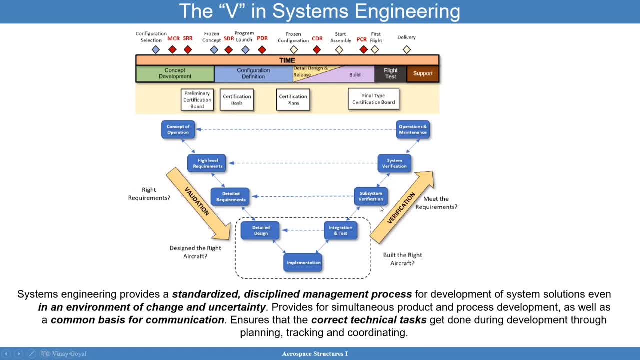 system verification. I'm looking at operational maintenance as a move up the V. the question now turns from design the writer: have I designed the right aircraft to have built the right aircraft and have a I met those requirements? here I'm saying: are those are right requirements? here is: 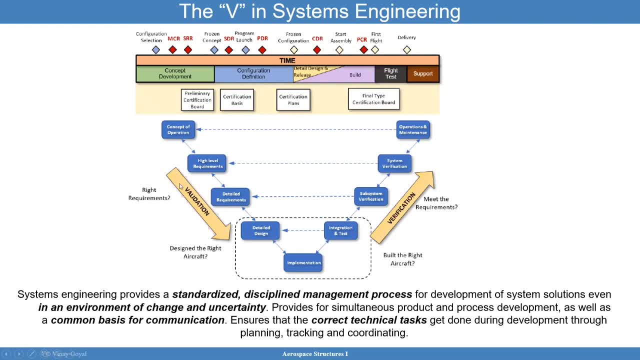 have I met those requirements, and so it's a big turn of events here, as you can see. okay, and so this V provides a simultaneous product and process development, as well as a common basis for communications, and ensures the correct technical tasks get done during development through planning tracking. 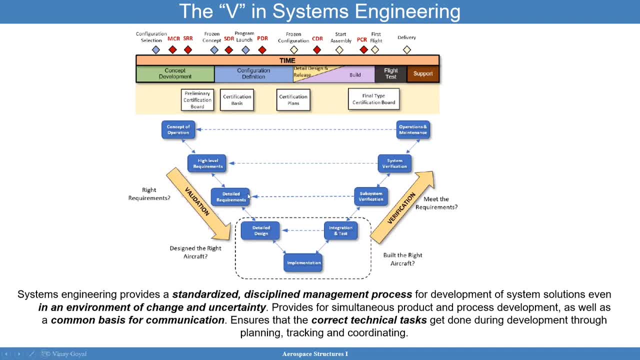 and coordination here. I'm always going back and asking those questions again. I was going back and checking: does it make sense? did my original assumptions make sense? did am I building the right aircraft? you know you're asking those questions even when you're going up the V, because what if you mess up? you may 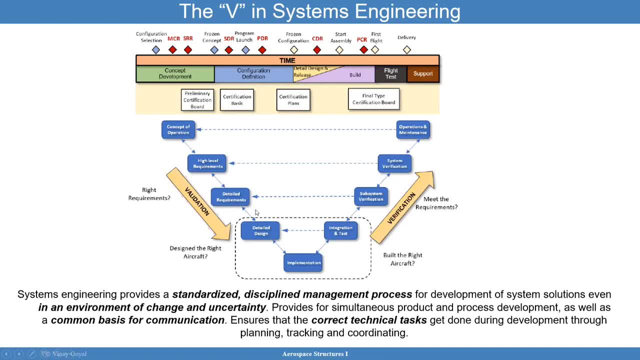 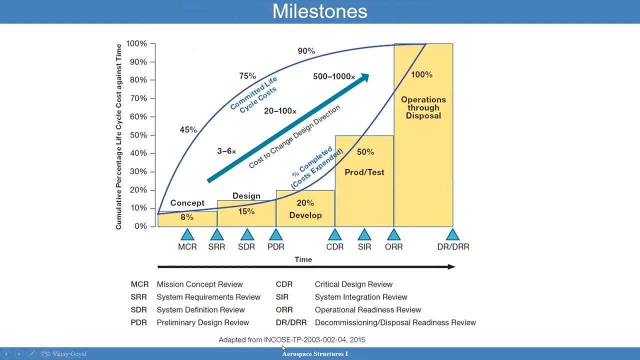 have to go back and revisit these requirements and you may have to revisit. am I redesigning what I wanted to in the first place? okay, you can see here the cumulative percentage lifecycle cost against time. this is: this has been adopted by this report here and you can. 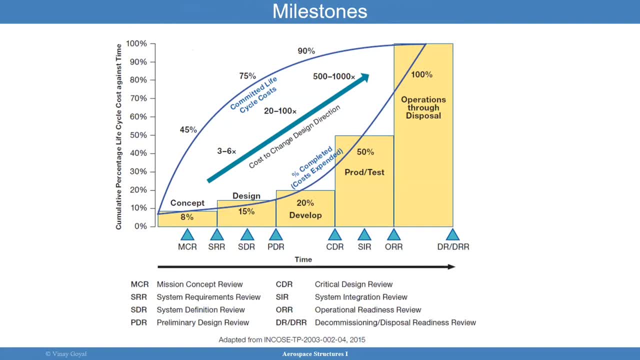 see here that you are spending a great deal of time here in the product test side and then you're gonna spend a lot of time later on doing operations and the cost is typically increasing over time as well. okay, and the cost to change direction later on becomes more and more difficult. so if I'm further down in the design, 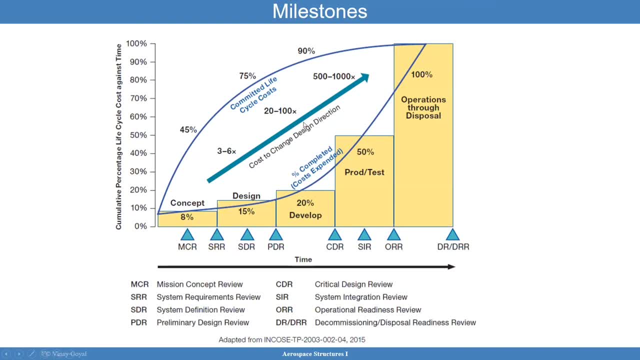 process and I find I have to change something, then that's gonna cost a lot of money. I have to go back and redo a lot of stuff and that's why it's important to do as many material tests as you can and subcomponent level testing as you can at the beginning to inform the designing. 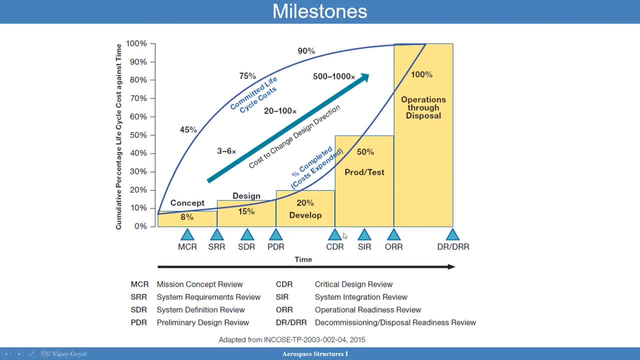 inform the developments so that when you're in this phase, any change in direction is minimal in terms of cost and schedule. but once you step into production and testing and you have some major issues, you're looking at five hundred times increase in cost and that's gonna be a significant problem in. 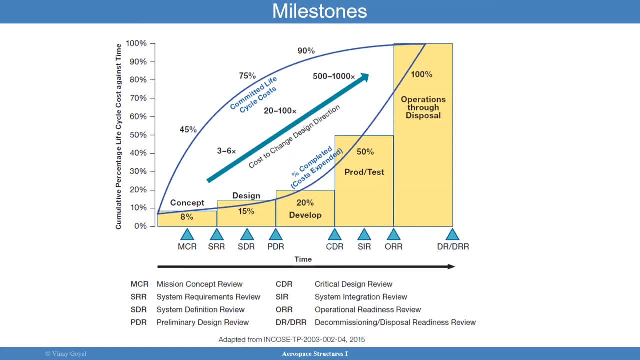 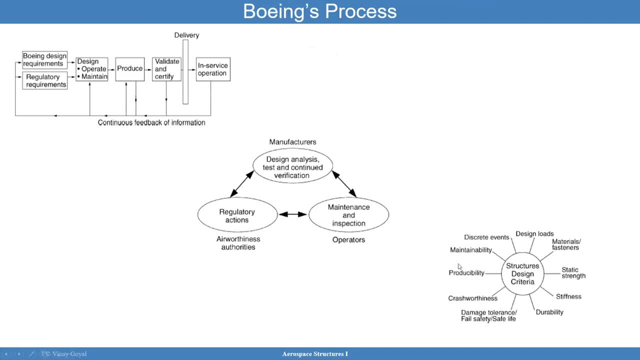 coming out long term because the quantity stays the same, for you, for the product. the Boeing process can be summarized in three different flow charts. you have a continuous feedback of information going back and forth between design requirements, regulatory requirements- so design requirements are different from regulatory requirements- and 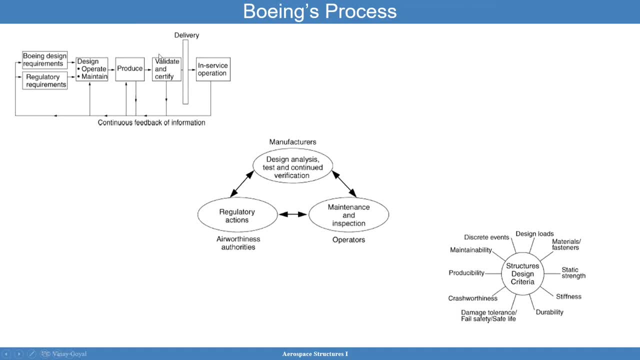 And we need to then validate and certify those designs so that I can then certify to enter it into service. But through this process I have continuous feedback of information. I also have to keep in mind that, as assistance engineering comes into play, that there's three areas that have to work very well together: Manufacturers, the airworthiness authorities and the operators. 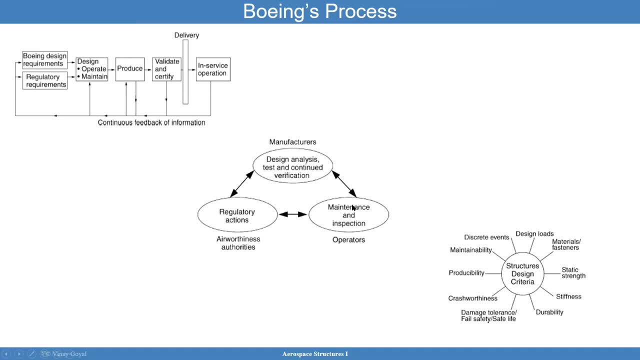 And all these three things have to work together. These three areas have to work together, Otherwise you may have a design that does not. it doesn't work well, And so it may not meet the regulations, it may not be easy to inspect, it may be difficult to maintain, and so forth. 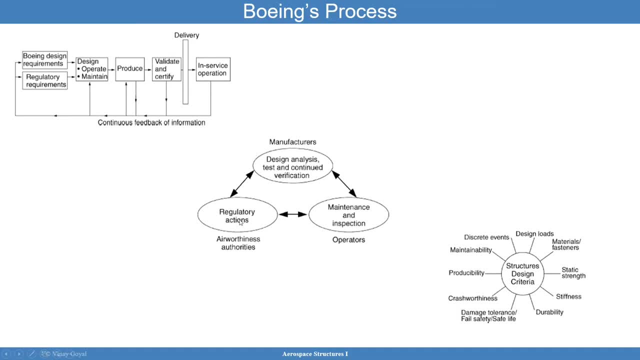 And so in all this, when I go one layer deeper, we have the structures design criteria. Can I make the part? Is it crash-worthy? Does it meet? is it damage tolerant? If I have a flaw, will it stop? Will it arrest? 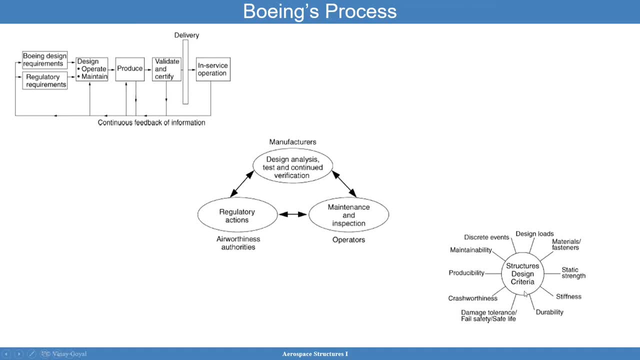 Does it have enough damage? Does it have durability? Can it take impact damage, for example? Is the stiffness correct? Do you have good fastener designs? Are the design loads adequate? Have I looked at all the discrete events? Can I maintain the structure that's been designed? 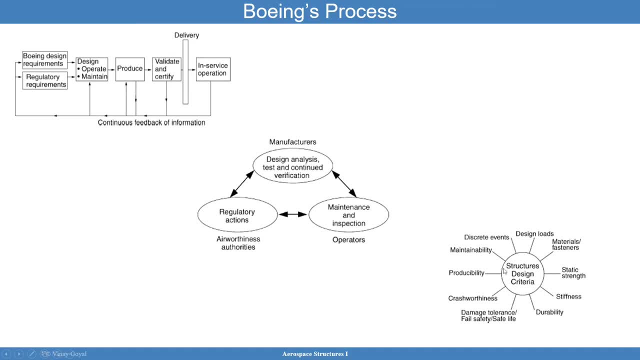 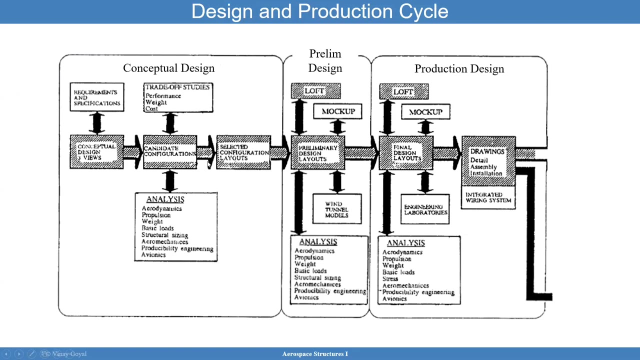 All these three floor charts need to be taken into account, And Boeing did a good job Of putting this together, And that's the one paper I discussed earlier that you should go ahead and read. And so here, when I look at a bigger floor chart now that includes disciplines, for example, it has the same elements that we talked about. 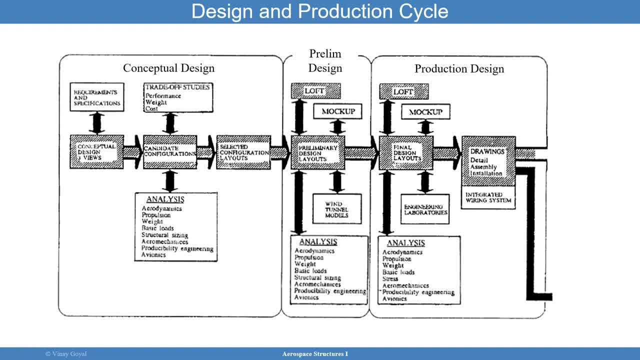 But I think it's good to see them. I think it's good to see them in this context. You have requirements and specifications, You have performance and weight cost trade-off studies And here you're in conceptual design And you're looking at candidate configurations. 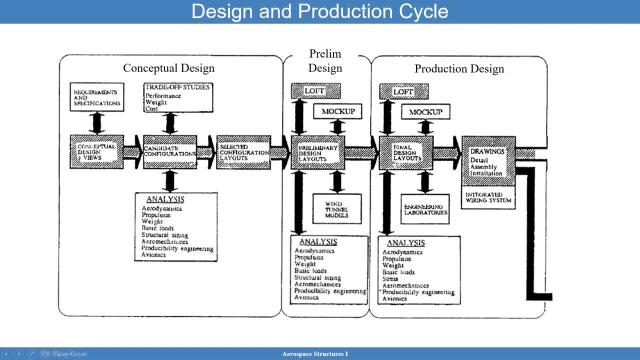 You select the right configuration layouts And here you're looking at analyses. that's going to be multidisciplinary. You're going to have aerodynamics, proportion, the mass properties team, the loads, the structural sizing, the air mechanics, And can you even make the part. 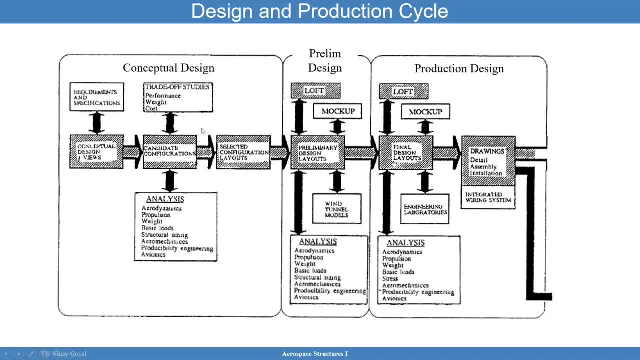 And the avionics. All that has to come together, And this is typically true for launch vehicles, aircraft and spacecraft. Once you go there, you go into preliminary design, And again all disciplines are involved, And wind tunnel models become important to demonstrate that those loads that are presumed are even accurate. 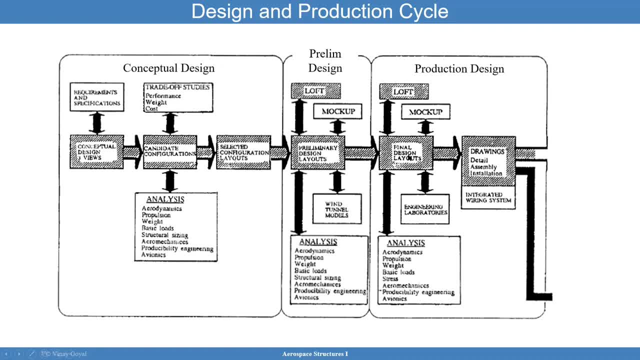 And then you enter into a phase where you start fascinating, You start finalizing those designs And you enter into production because you're going to have to test those designs to make sure they work And again that requires engineering laboratories. It may include integrated disciplines together working together to determine whether the production design is adequate. 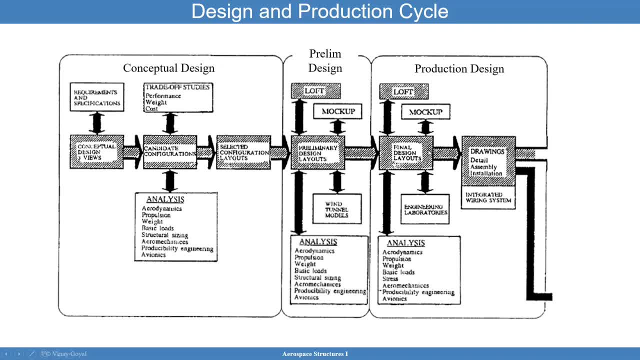 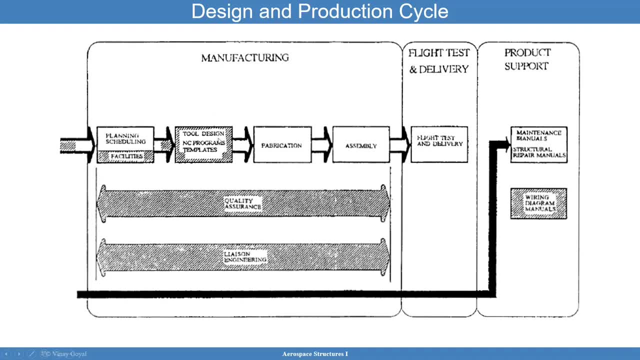 And here you have laid out the designs. After CDR, you can release the drawings To then start manufacturing the parts, And that's going to require facility developments, tool designs, fabrications, assembly, And here you have quality assurance getting involved and making sure that the parts are getting fabricated to high standards. 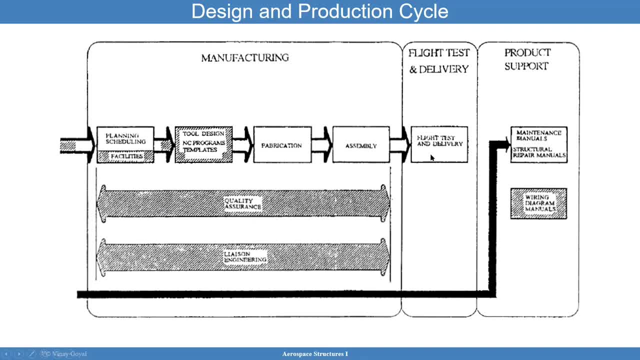 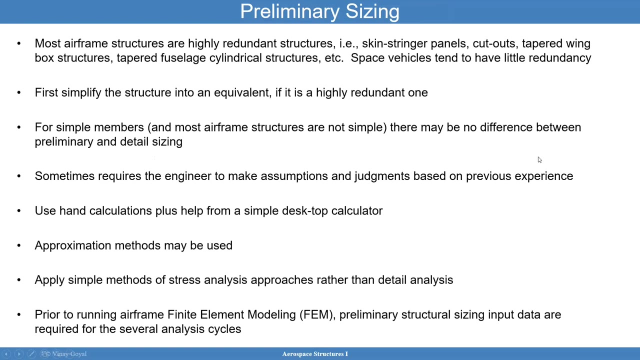 And once you've gone through flight testing And the product has been certified- Certified- It's time to deliver the aircraft. And all along with ensuring, the whole time as you're working through these drawings, That you are developing manuals for maintenance And structural repair manuals. 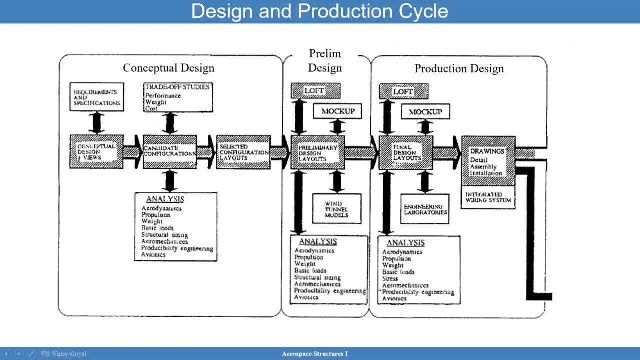 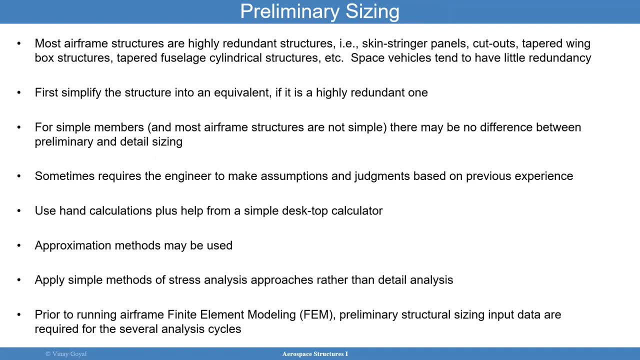 This process is going to require some preliminary sizing. A lot of questions I get sometimes is: you know, can I start using finite element models Early in the design process, The conceptual design phase? But the fact of the matter is is that most airframe structures are highly redundant structures. 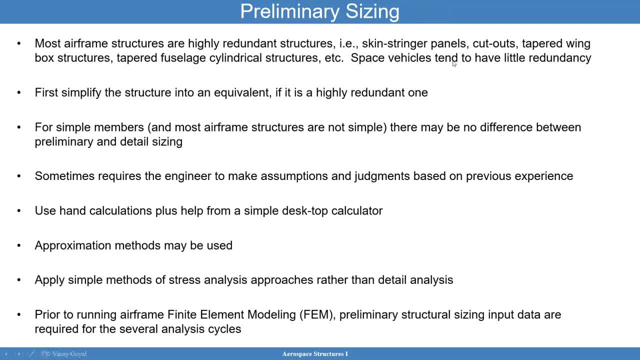 And space vehicles, like launch vehicles and spacecraft, have little redundancy. Regardless, typically when you're in the concept design phase and preliminary design, You try to rely on hand calculations That verify for simple finite element modeling And so for simple members It could be a simple analysis that's done with hand calculations and using a calculator. 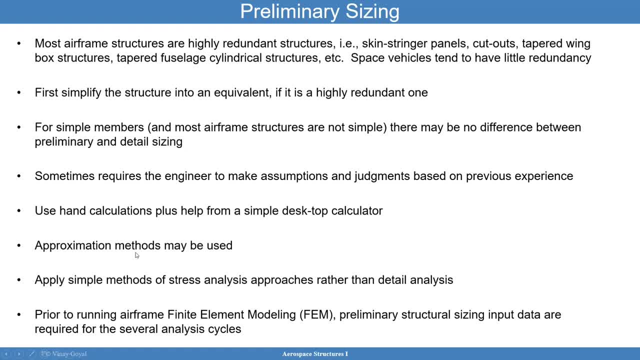 Like Excel or something like that. You can approximate some of the designs. You can apply simple stress methods that you learn from mechanics and materials Rather than a detailed analysis, Because detailed finite element modeling is highly cost, It's not cost effective And it may not put you in the ballpark as quick as a preliminary analysis. 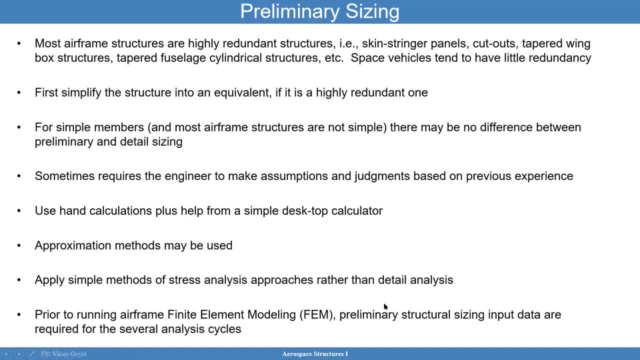 So the preliminary structural sizing input data are required for several analysis cycles, And it could include finite elements. It's just that before you touch finite elements, You want to ensure that you have done some preliminary sizing by hand calculations, Because once you go to detailed sizing, 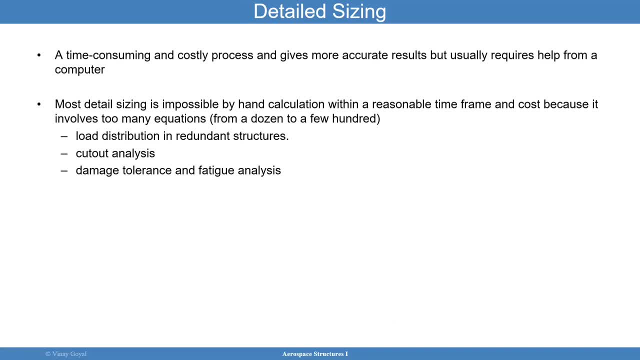 That takes a lot of time, Especially when finite elements are used. Sometimes detailed sizing is very difficult to do by hand calculation. Hand calculation puts you in the ballpark, But the detailed work puts you closer to the goals that you need to achieve, Because finite elements are really required. 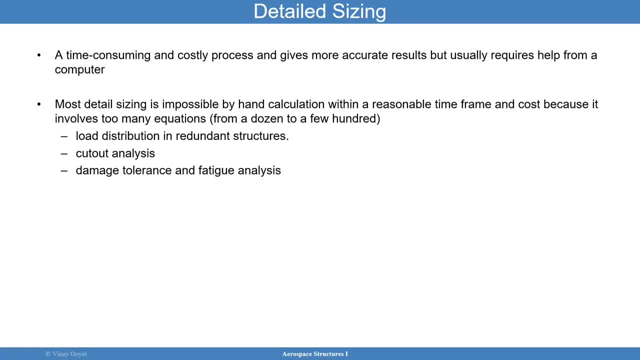 You're looking at structural designs that have very low factors of safety, That have to be weight sensitive, Basically low weight And cost effective, And so you want to make sure that you've done as much sizing as possible by hand calculation Before you step into more complicated modeling. 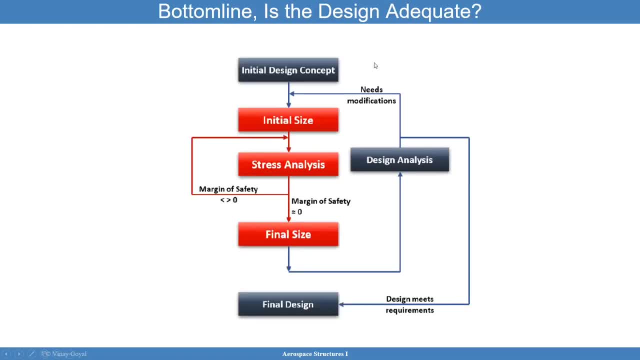 And bottom line: Is the design adequate? To answer that question, There are cycles that you have to go through. Initial design: concept: You have to ask the question: Do I have positive margins? Initial design: Do I have positive margins? I do a stress analysis. 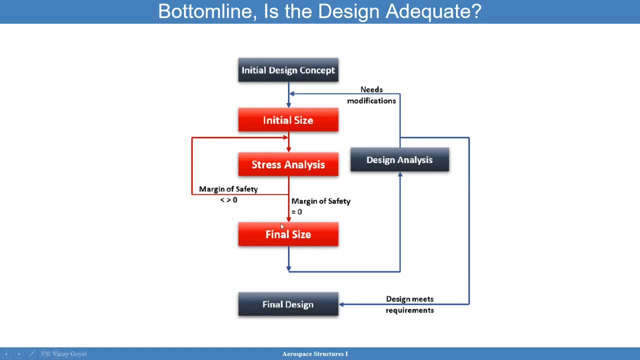 Figure that out And I iterate with the design And then go into more detailed design Until I'm happy with the final design. Now that doesn't mean That the structure is going to be safe. I have to test the structure first. 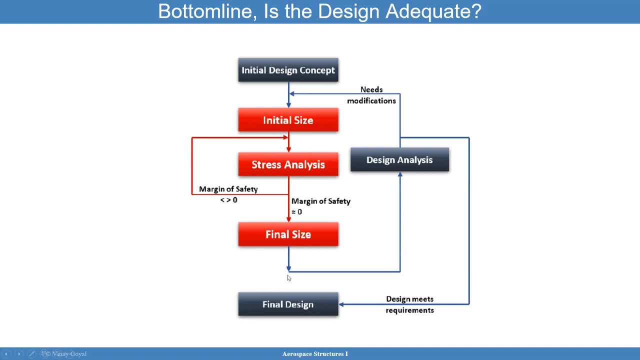 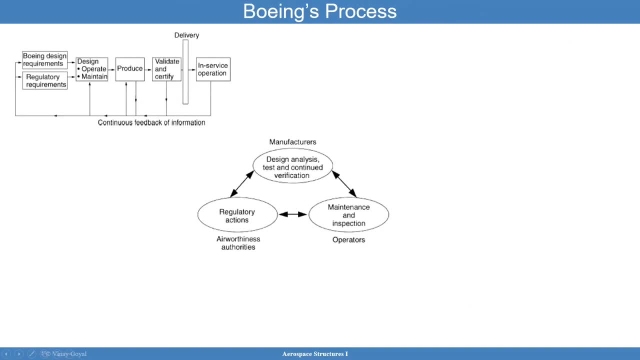 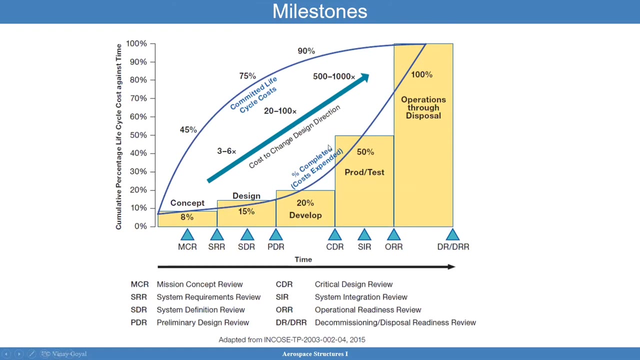 And validate my models, Because if there's a problem there, Then I may have to go back to the drawing board And that, as we said, Will cost Quite a bit of money. The more time passes by And the more mature the system begins. 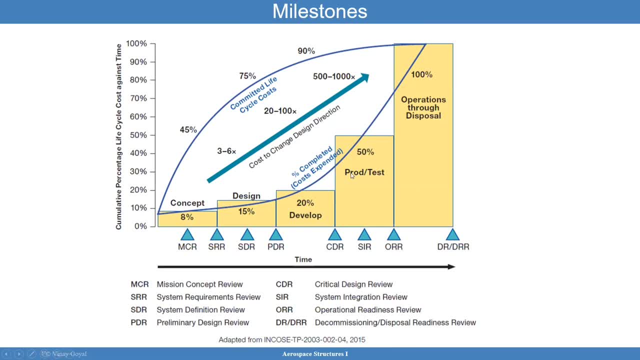 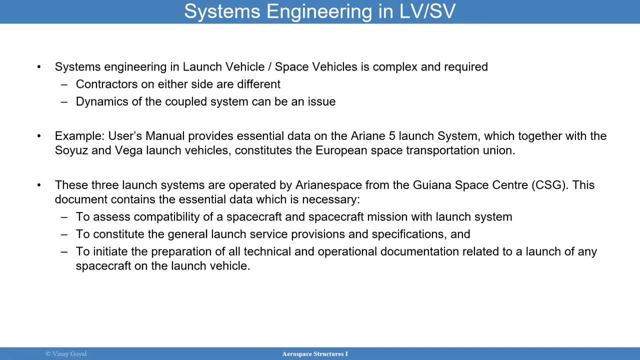 If I have to change direction. We're looking at a significant amount of cost And schedule delays. Systems engineering, Launch vehicle and space vehicles Is extremely important And is required. Contractors on either side are different, So the contractor for launch vehicle. 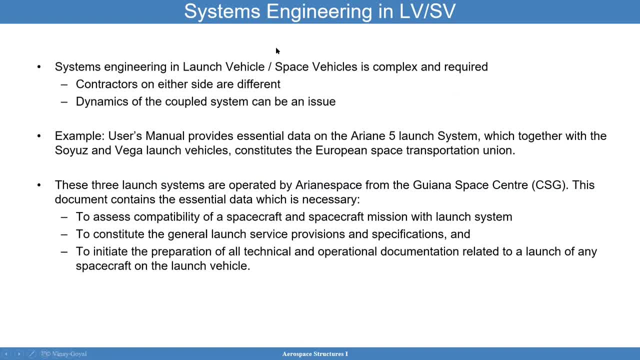 May be different from the contract and space vehicle, And also these vehicles have to be coupled together In a dynamic models. We'll be talking about that- And so systems engineering here Is highly required. Interfaces From the launch vehicle side Need to be properly defined. 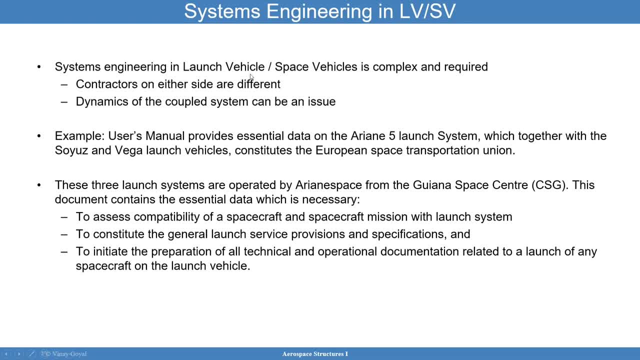 Compared to the space vehicle side, The vibration environments That launch vehicle produces. You don't want to break the space vehicle With those vibrations during ascent. So all that Shows and highlights The importance of systems engineering. What if I need a 90,000 pound payload? 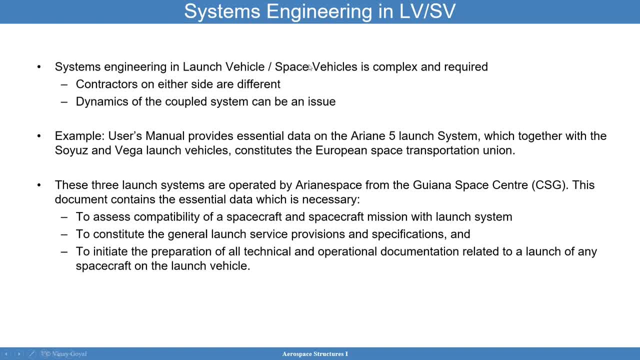 Is a launch vehicle I'm selecting even Able to take, that. I'm going to show an example of a user's manual That provides essential data on the Orion five Launch system, Which, together with the, With their other launch systems, constitutes. 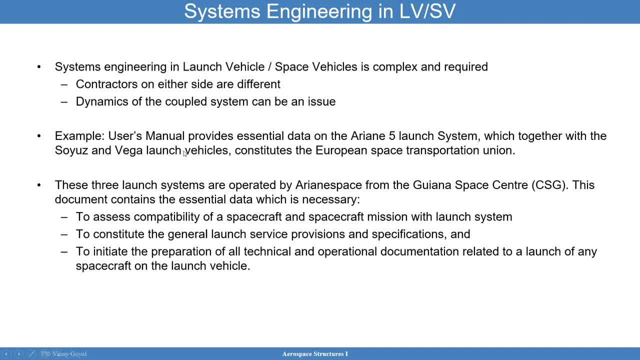 Their transportation systems, And so Their user's manual typically contains Compatibility of a spacecraft And spacecraft mission with launch system. It constitutes the general launch service provisions and specifications And provides data to initiate and prepare Of all technical and operational requirements. 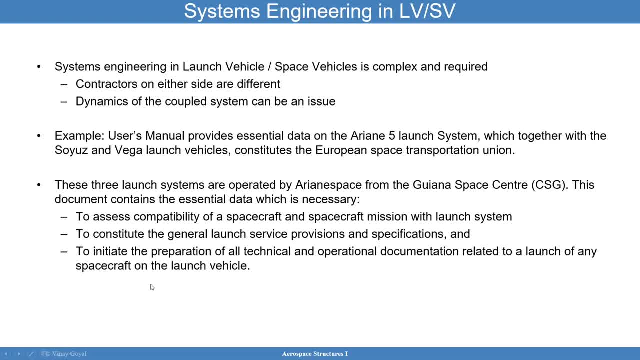 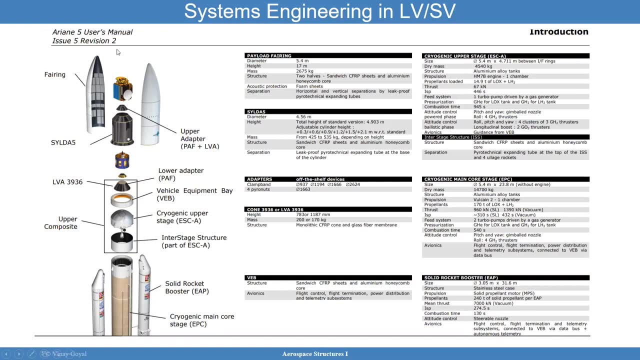 For any launch of any spacecraft on the launch vehicle. So again you have the payload inside the launch vehicle. We want to make sure That we have compatible systems, And so here Is a Orion. five years of mantle. Issue five, revision two is an older version. 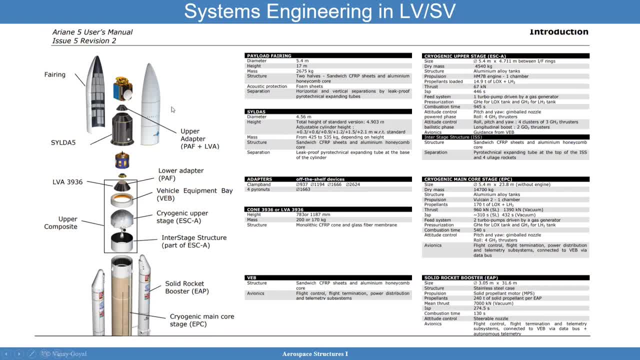 but the bottom line here is that It gives you information about the various systems From the payload fairing. The diamond is 5.4 meters. What do you have? a bigger payload? Maybe you have to come up with a different fairing. 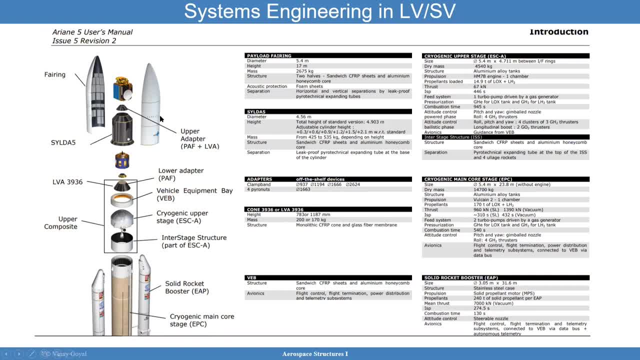 What kind of acoustic protection you have For your spacecraft. It's going to give you information about the the adapters In the launch vehicle adapters. They're going to connect To your spacecraft. It will give you information on the upper stage. 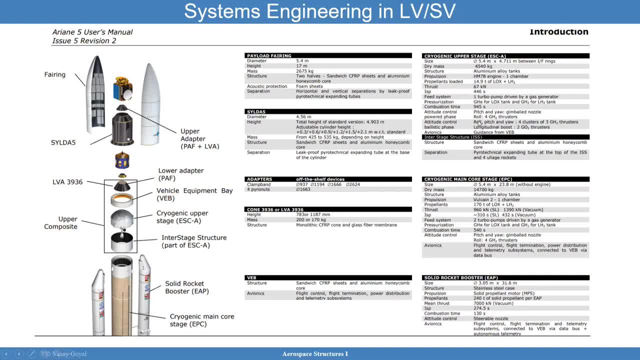 And The added to control power phase is going to give you information about combustion time And so forth. It's going to give you information about the main core stage And the star rocket booster, ISP information, Combustion time, The engines. 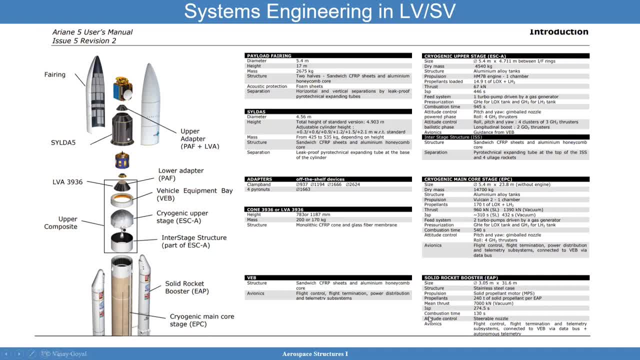 ISP And so forth. It's going to give you information about the main core stage And the star rocket booster, ISP- What kind of structure are we talking about? Stainless steel case in their case? And it's going to give you information about avionics. 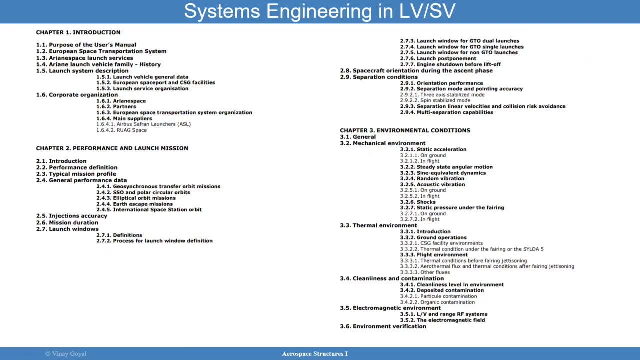 As you can see in all the different components. Here is a quick view Of the kinds of information you will find in their user's manual. It's going to provide information on The performance and launch mission, What kind of orbits you can achieve. 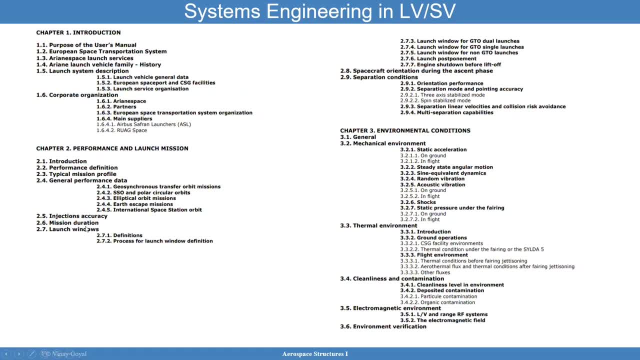 Insertion accuracies, Mission duration, Launch windows. It's going to give you information about spacecraft orientation during the same phase. Horizontal vertical: How is it oriented? Separation conditions Is going to have information The environments. Static acceleration, Steady state. 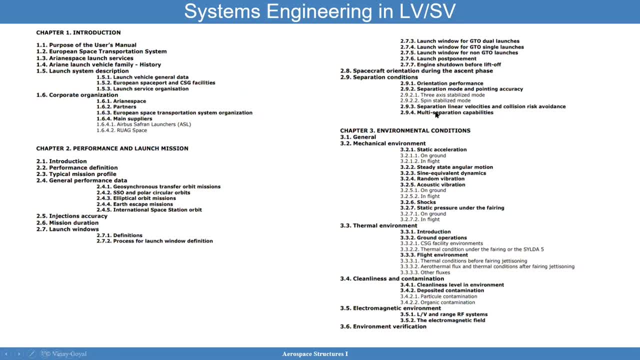 Angular motion. It's going to give me all the information you need To eat, Be able to ensure your spacecraft can Sustain those environments. And it's going to give you All the information You need To eat, Be able. 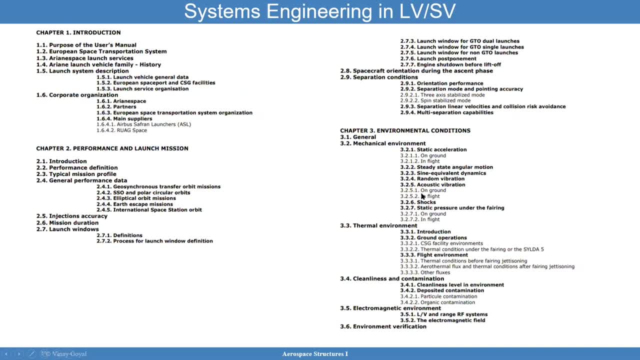 To ensure your spacecraft Can Sustain those environments. It's going to give you All the information You need To eat Meteorites, Be able to take Benefits of orbital. jakieś scan Gives you That information. 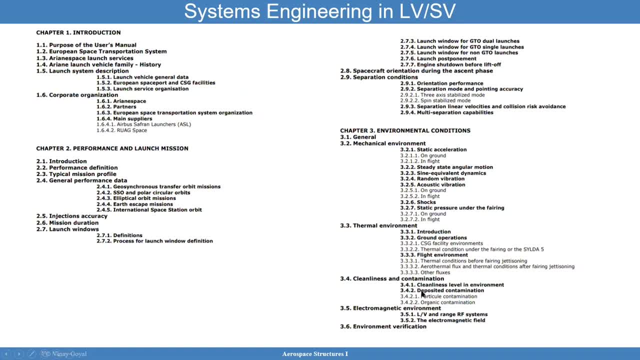 It's going to help you. Hold on for one second Here Recording, Okay, So the You know, Remember You cannot Why increasing How it works. It's a tough ask, So I'm going to To give you. 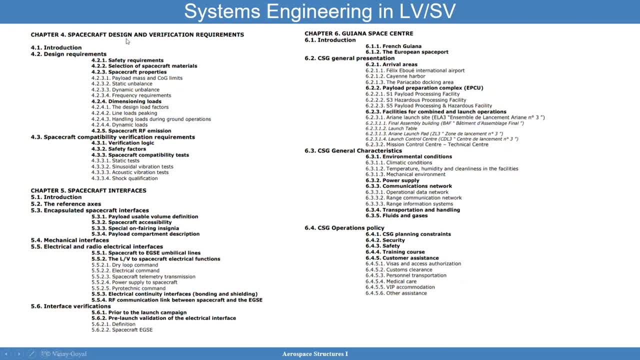 A mixed experience. cock, No mondo's. The big question, The how In Spacecraft. But you say How you breathe. Does it into Spacecraft interfaces? where are those interfaces defined and how they're encapsulating the spacecraft interfaces and so forth? 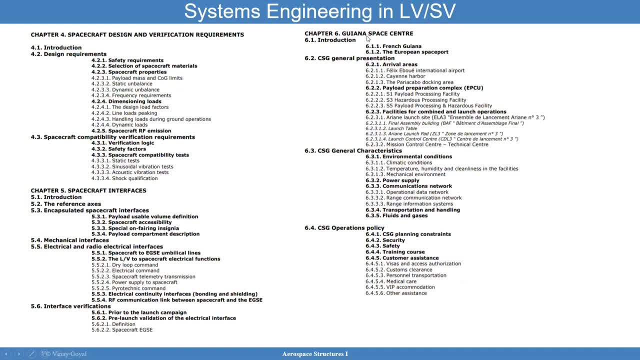 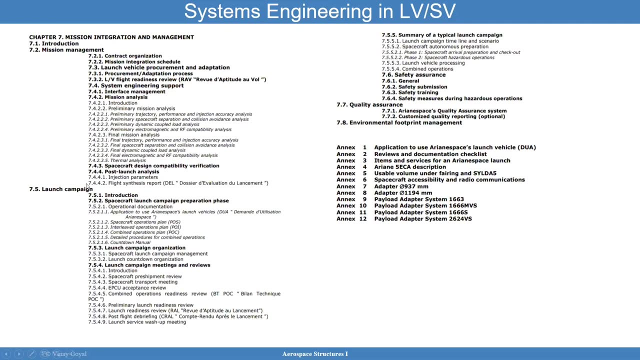 So you're going to see a lot of information there on that, And then you have the operational space center location and the range information and mission control information and so forth. You also have mission integration and management, The launch campaign itself, countdown information, spacecraft operation plans, quality assurance. 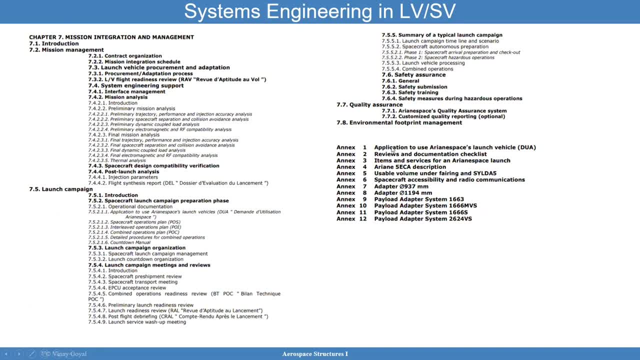 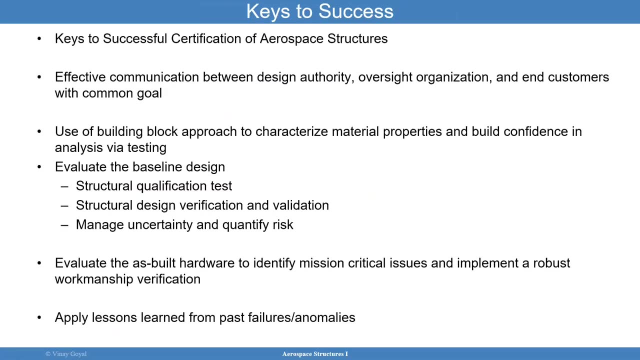 And then you also have a bunch of appendices, normally that provide even additional information there. So I hope that makes sense to you guys as we go through. So what are the keys to success? Any, any, any problem. In any program to succeed, it's important that we have effective communication across the organizations, the design authority, the end customers. 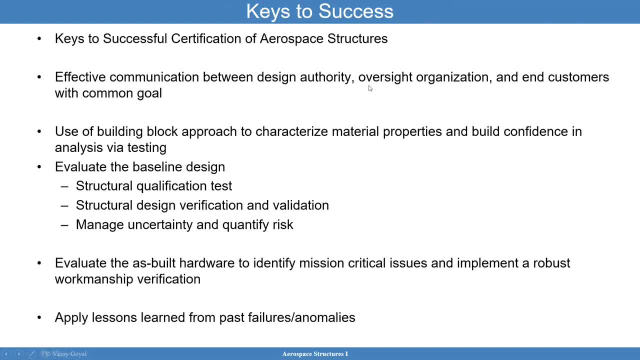 We want to have a great communication across the same company as well. It's important to use a building block approach- We'll be talking about that more- But it's important to correct, Characterize the material properties and build confidence in the analysis via testing. 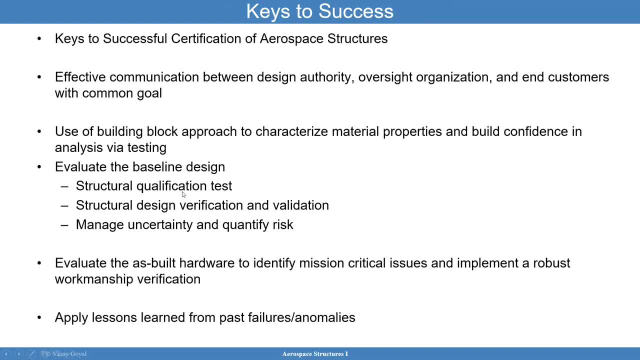 We also want to evaluate the basic design through testing, manage uncertainty, and we'll go through all that into a deeper level later. You also want to make sure that, as built hardware is is is good for the actual application. So the thickness of the fuselage came out shorter than the thinner, than the actual. 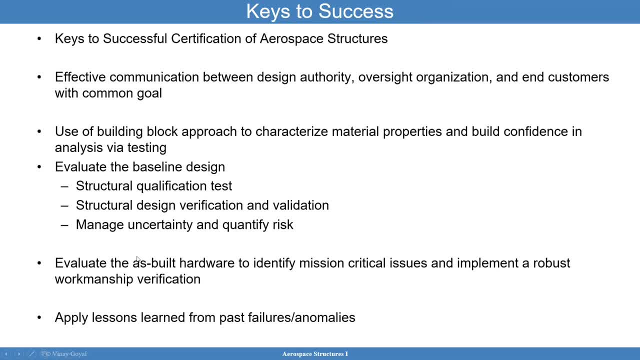 The actual Drawings. you will not be able to evaluate that, the workmanship of it, And one of the most important things is to apply lessons, learn from past failures and anomaly. One of the biggest lessons learned I want you to keep in mind as we go through this course is to not to forget the lesson learned. 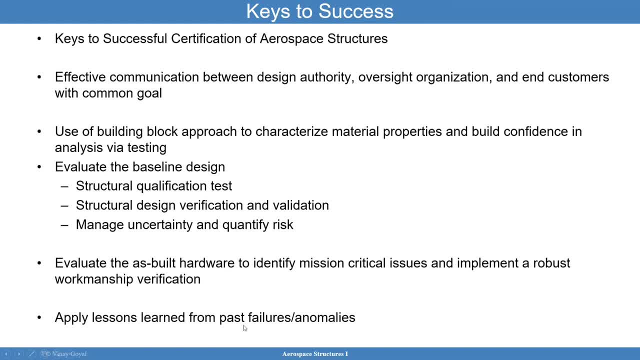 That is a lesson learned: not to forget the lesson learned from pass phasors and anomalies and bring them to light as you're working through issues. If there's a corrosion issue issue with the particular material system or there's a hydrogen embrittlement situation or 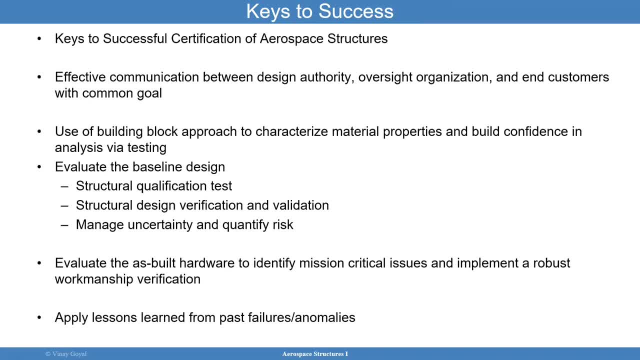 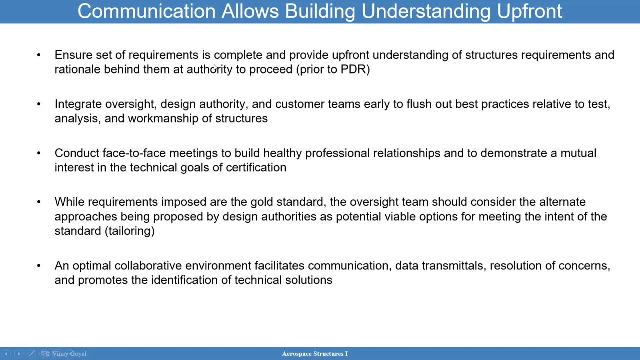 some other scenario- failure mode of concern- you want to bring those elements in into the design to make sure you're not repeating those mistakes. so communication allows building an understanding up front. ensure the set of requirements is complete and provide upfront understanding of structural requirements and the rationale behind them. you also want to integrate the 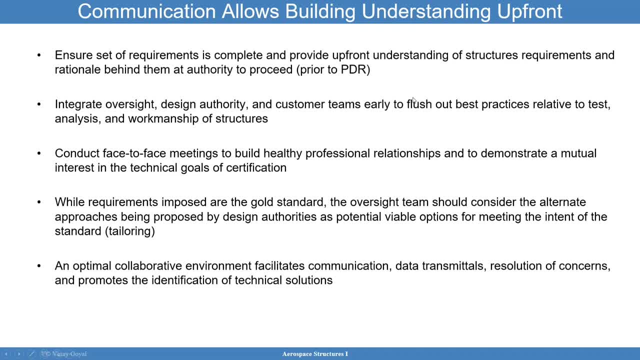 oversight, design authority and customer teams early to flush out best practices relative to test analysis and workmanship of structures. i think it's important to to have face-to-face meetings to build healthy professional relationships and to demonstrate a mutual interest in ensuring that you're marching towards the same goals. 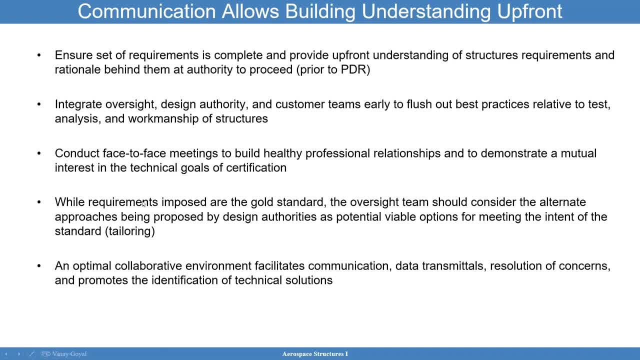 as everybody else, because you don't want to have miscommunication too late in the game. and while requirements imposed by the regulatory agencies like nasa are gold standard, it is important for the teams to be open-minded about possible ways to solving the issues at stake. you there might be ways to get there that have a low level of risk compared to other alternate.